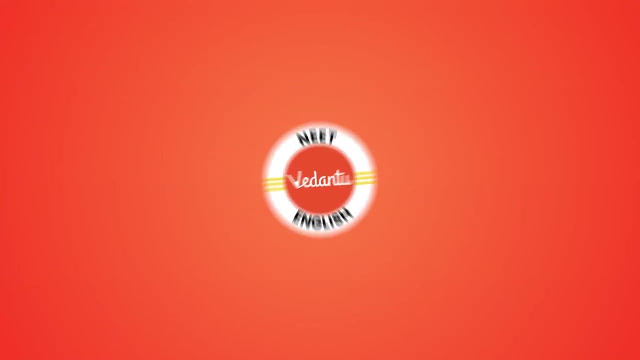 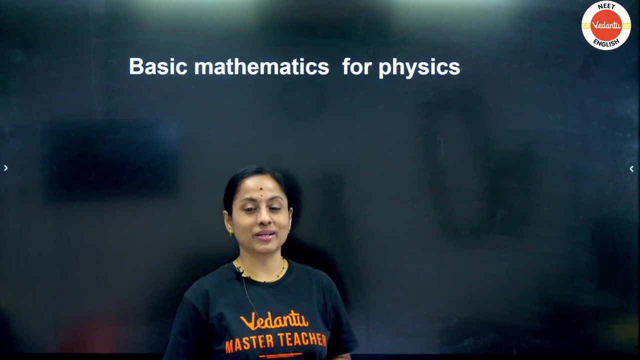 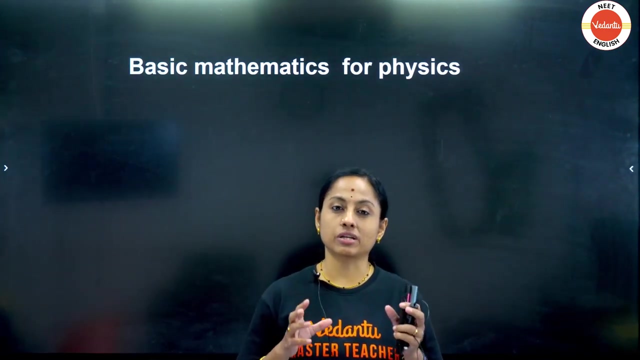 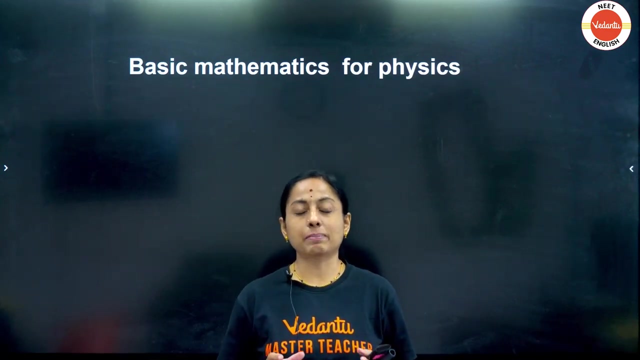 Hello everyone, hope you all are doing good. Welcome to Vedantu NEET English channel. So in the process of covering our series of lectures in part of preparation for NEET 2024.. So let us start with a very good topic which is very much useful. So, being bio students, you have 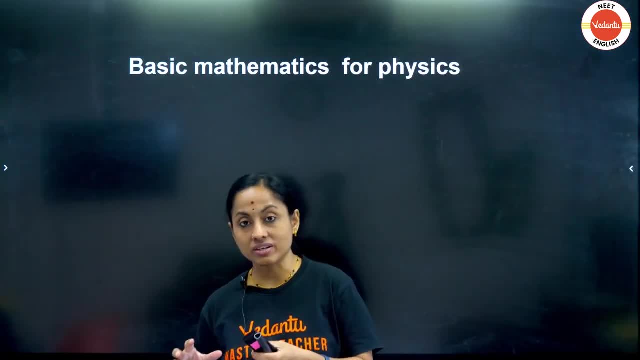 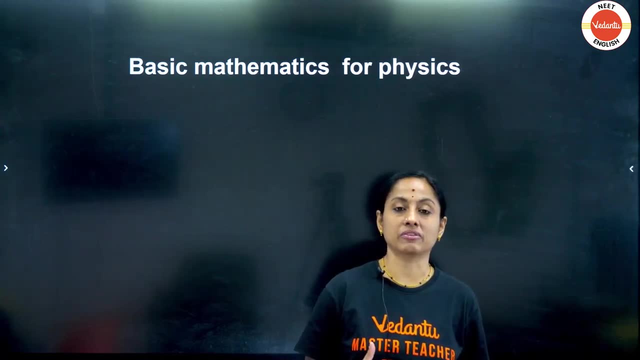 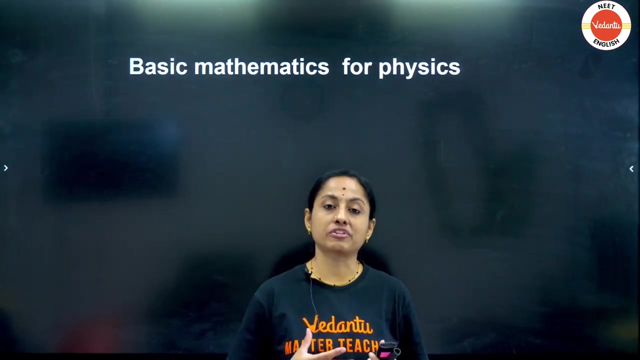 a problem with physics only because of the major reason: is the mathematics part of the physics right? So many bio students feel uncomfortable with physics when some integration problem comes, some calculus problem comes. So the mathematical part of the physics becomes tougher for the bio students because, as we know that you 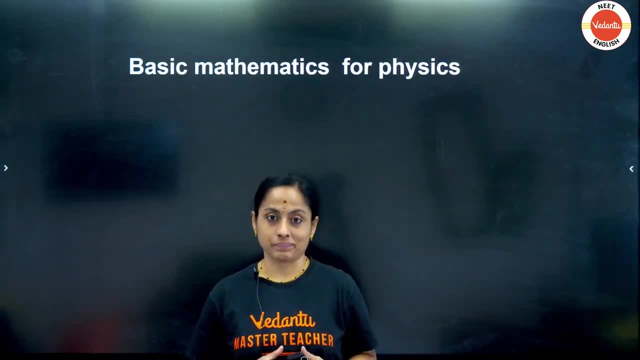 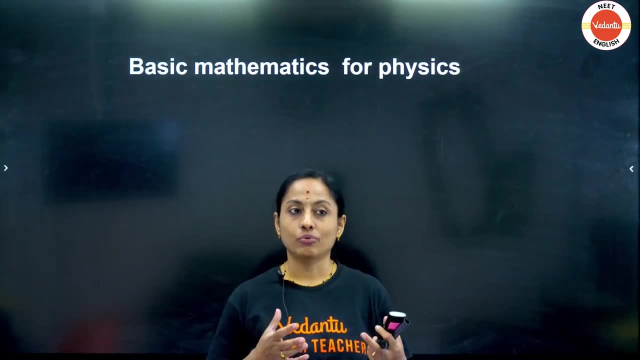 are no more going to study about maths, right? So? and we have to learn the mathematics. that is a part of the physics. So, first thing, what we will start today is with basics of basic mathematics for physics. So what are the parts? We are not going to learn the entire mathematics, So only. 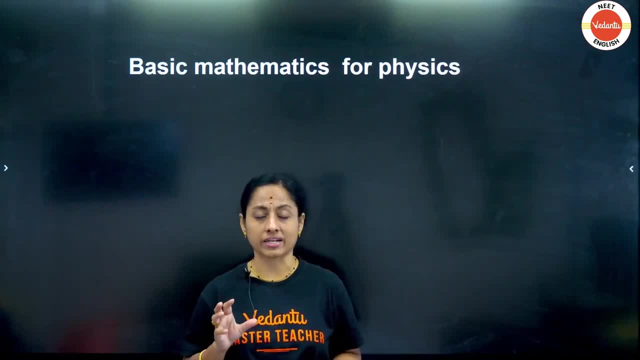 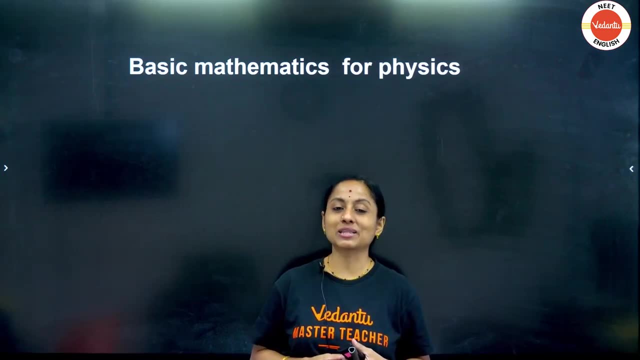 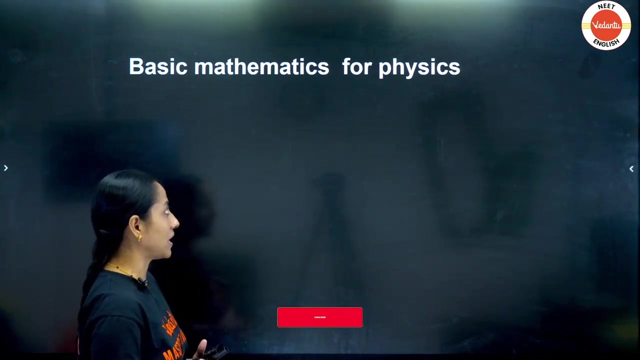 basic mathematics. What mathematics is required for the preparation of physics? Only that much we are going to concentrate. So welcome to Vedantu NEET English channel. This is your master teacher for physics, Ramadevi or KRD. ma'am, I am very much known as Okay, so proceeding with. what are the? 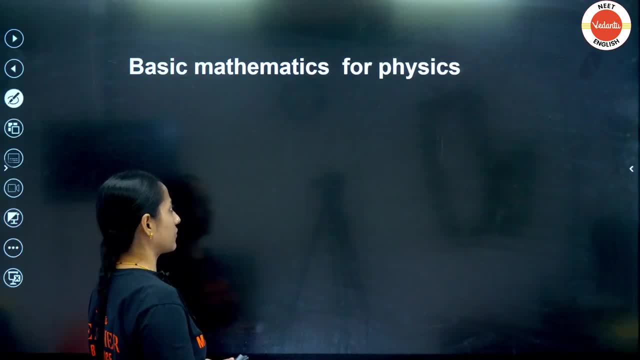 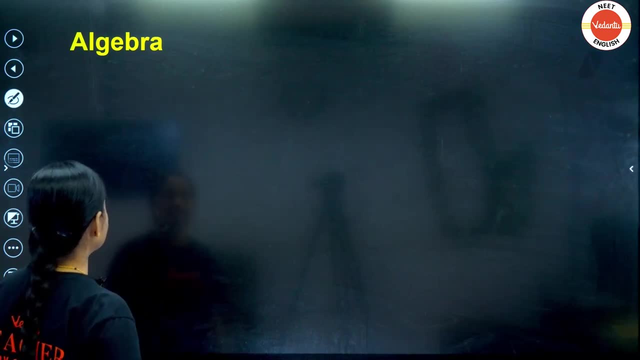 basic mathematics that we are going to learn. There are many things that we are going to learn, but I will make it as much as easier possible for you. So starting with algebra. So if we start with algebra, Algebra is not a topic which is only learnt in intermediate but, yes, in your lower. 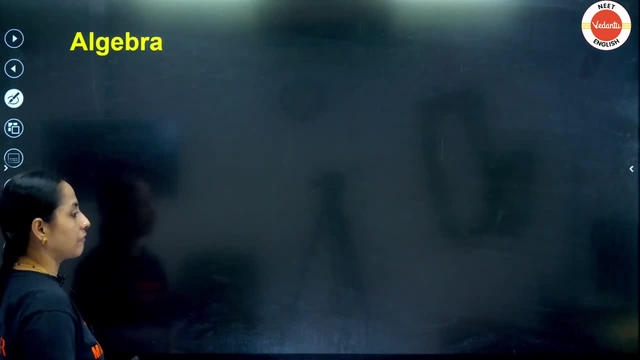 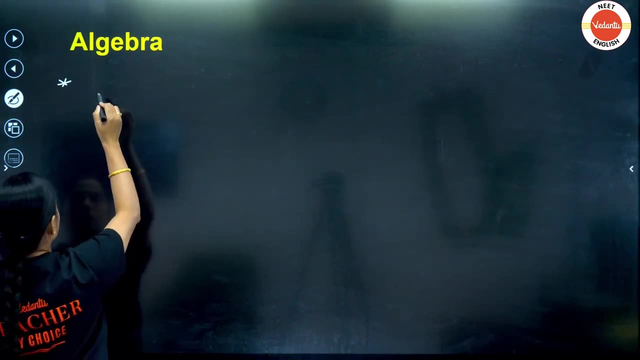 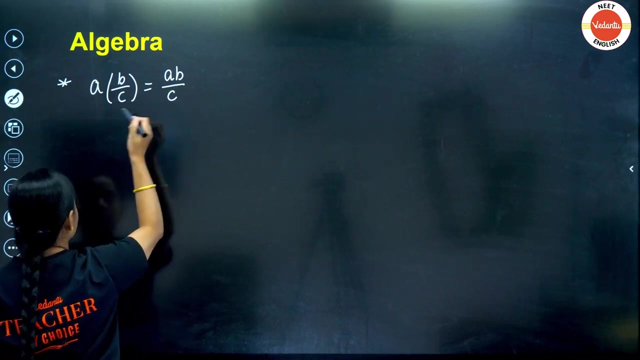 classes. also, you would have met with algebra. So in algebra we will have functions and all, But I will not name it. but we will just see what are the kind of formulae we will be using. For example, if you are multiplying A with B by C, So we can write it as A, B by C. This much you already know. 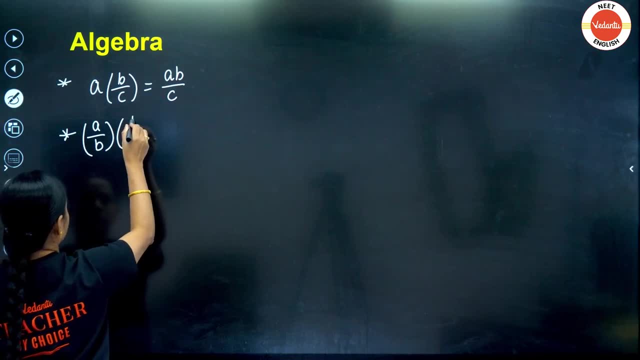 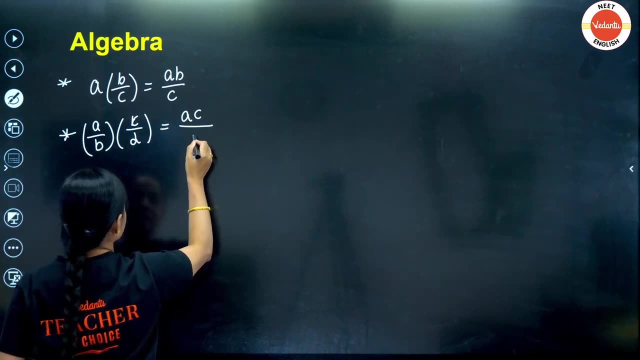 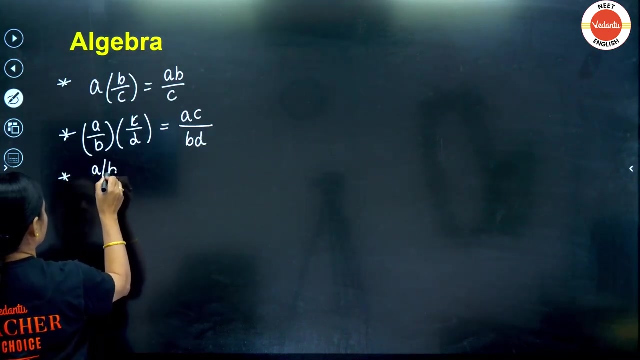 For example, I am multiplying A by B with C by D, So all the numerator part, denominator part, can be multiplied and it can be written as AC. This is also very much known by you. For example, if you have written A by B by C by D. So how do we? 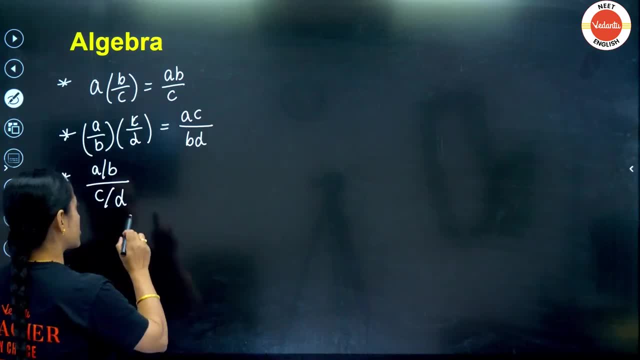 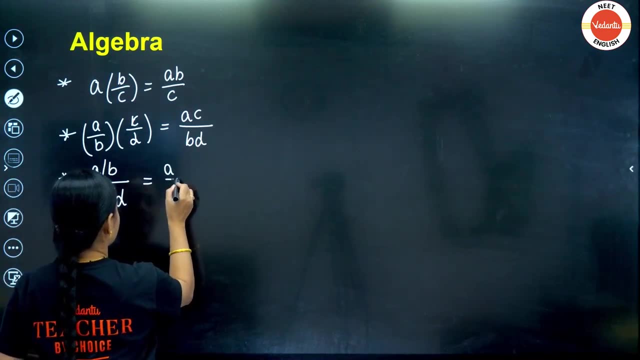 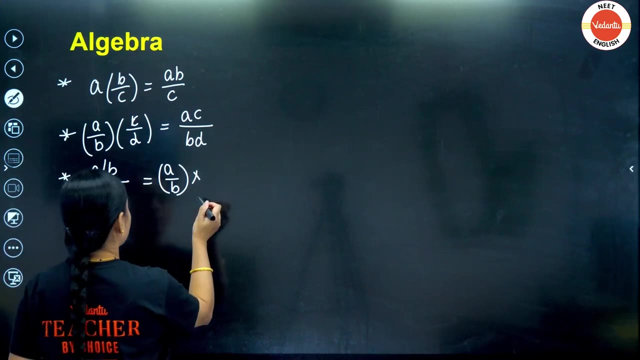 write So always. when the division has to be converted into multiplication, then denominator becomes reciprocal. So here we can write this as A by B into. this becomes actually C by D, whole power minus 1.. C by D, whole power minus 1 is nothing but. 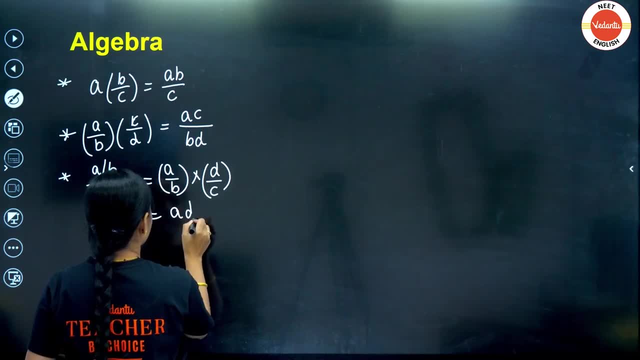 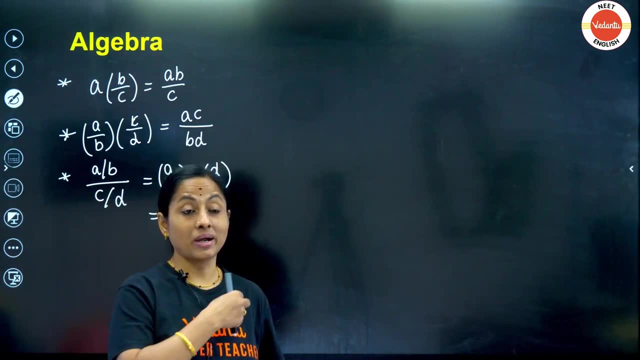 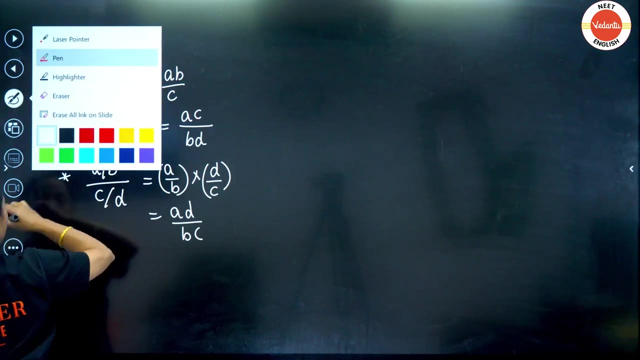 E by C. So the final answer is A into D, by B into C. So these are all the operations which we use in algebra. So you might not be knowing the name algebra but, yes, this kind of operations you can easily perform. So this is one part to be learnt in algebra. The next part to be learnt in algebra: 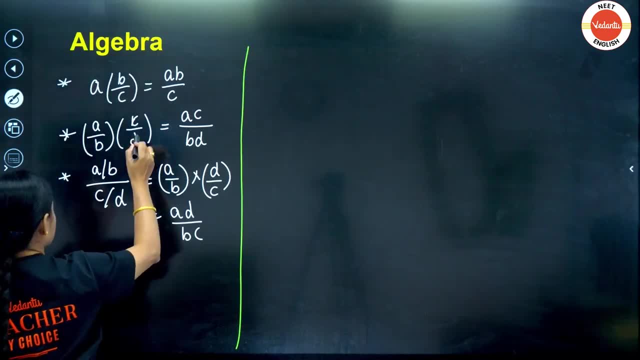 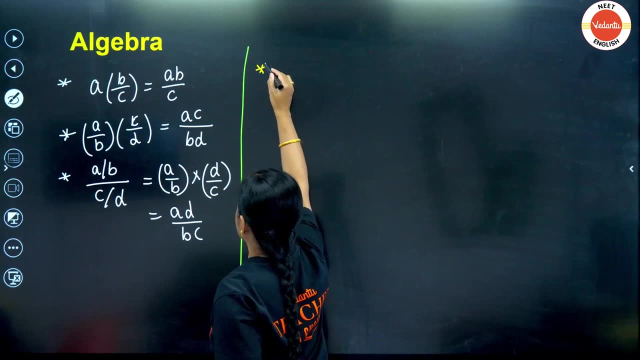 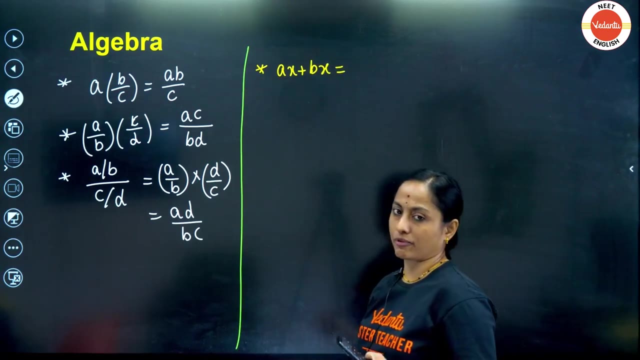 is how to find the fractions, How to find the fractions. These are the kind of functions. Now, how to find the fractions? So how to find the fractions. So to find fractions, for example, if you are given AX plus BX, This is a very simple form. Let us start with very simple forms and then we'll. 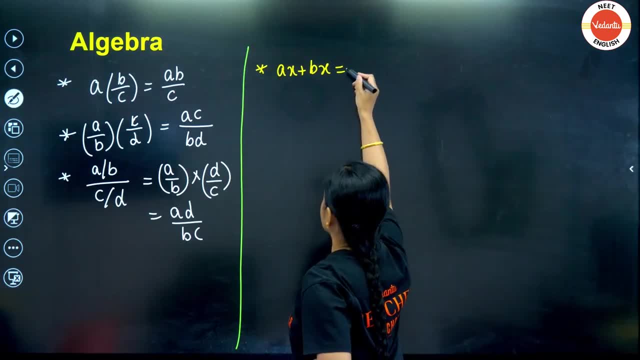 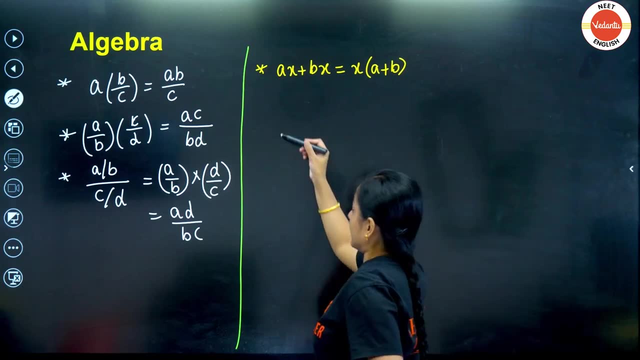 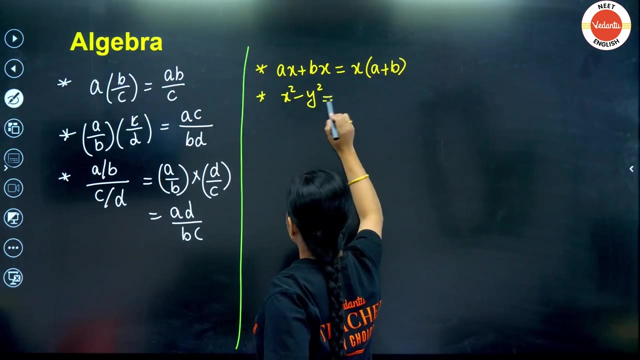 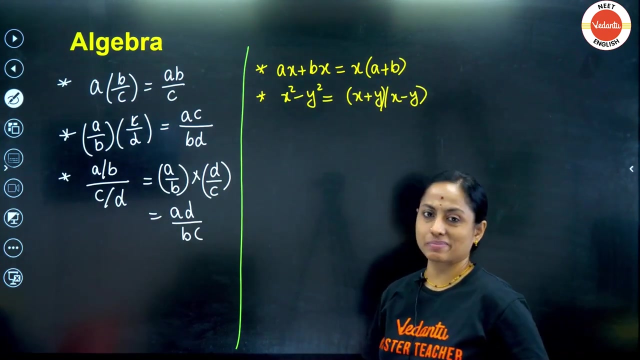 see how depth we can go. So AX plus BX. So we can always take X as common and this can be written as A plus B. Next, if you are given X square minus Y square, this can always be written as the fraction of X plus Y into X minus Y. So A plus B into A minus B. A square minus B square is equal to: 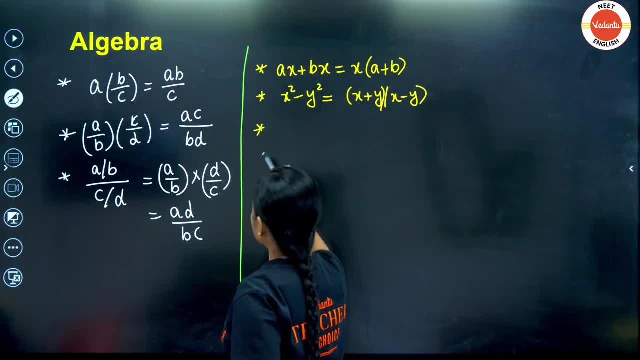 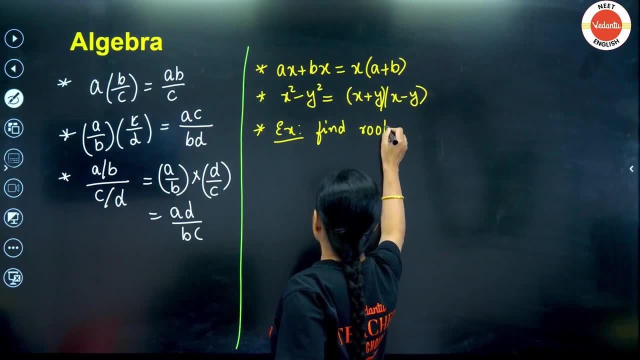 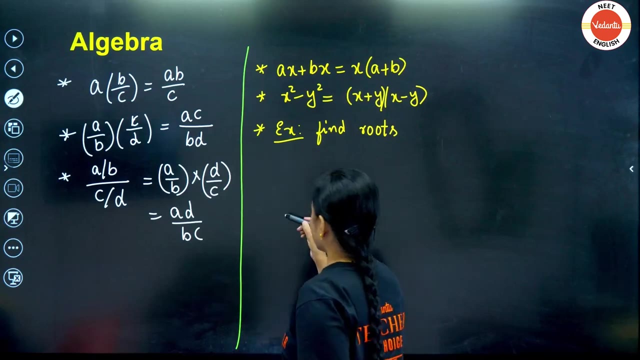 A plus B into A minus B. Next, if you are given- Let us take another example- How to find roots. How to find roots- This kind of problems we may find in our physics. So how to find the roots for that, Let us take an example. I'll explain with an example. For example, you are given: 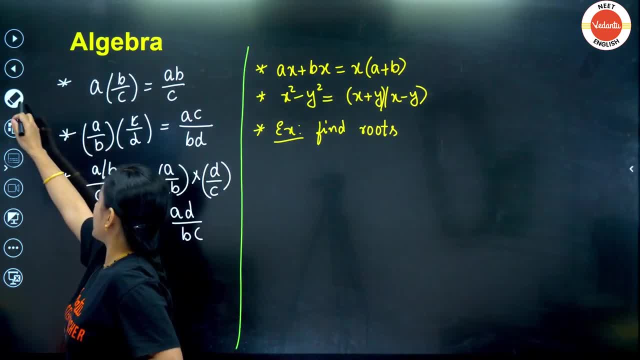 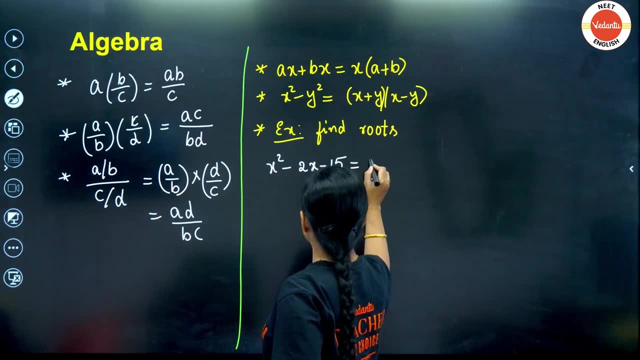 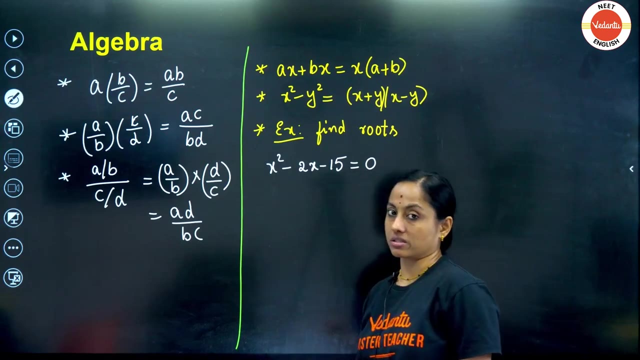 X square. Let us take, for example: you are given X square minus 2X, minus 15 is equal to 0.. Find roots for this. So the easiest part is you know how to find the roots. I'll tell you two methods. 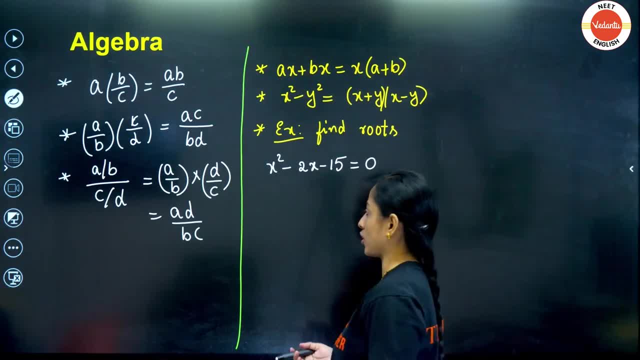 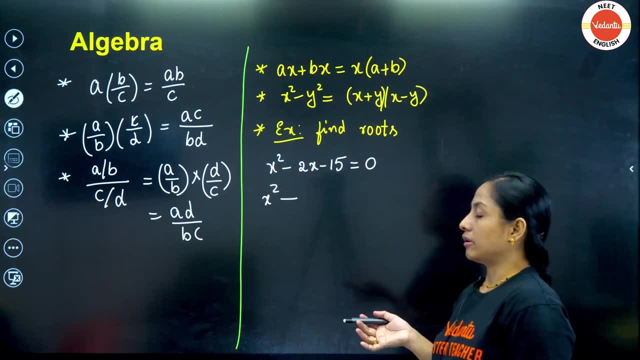 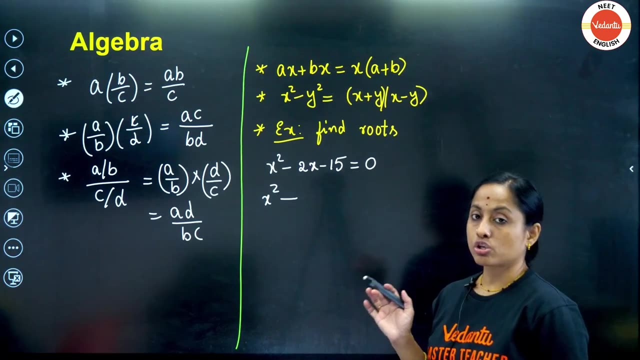 One is the common one and the other one is by using the formula. So here I can write: X square, It is minus 15.. So find the roots for 15.. So what are the 15 multiples? So 15 is a multiple of 5.. 3s are 15.. So that is the best thing I have, because here I 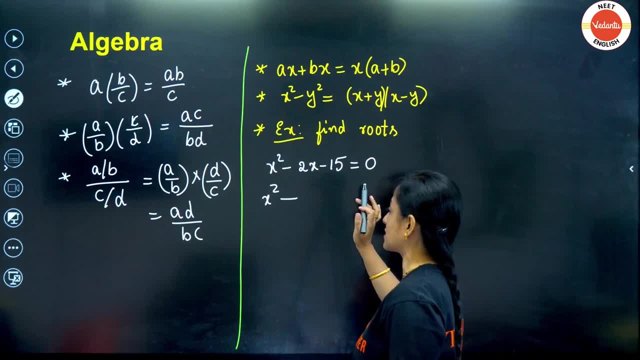 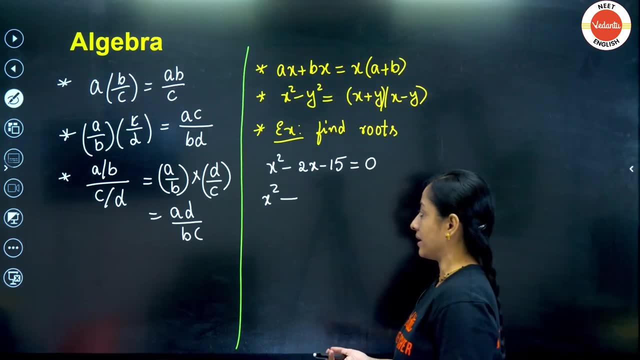 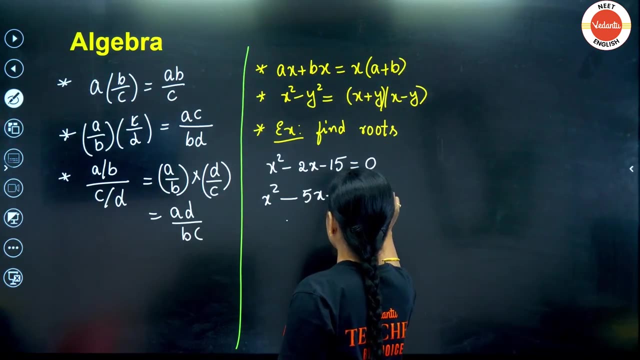 need to get 2.. 5 minus 3 is 2.. So it is very much suitable. And minus sign is dominating, So I have to get the minus sign as reminder. So big number minus small number. So minus 5X plus 3X minus 15. 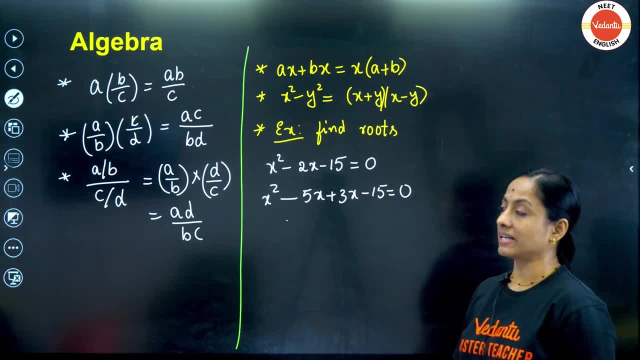 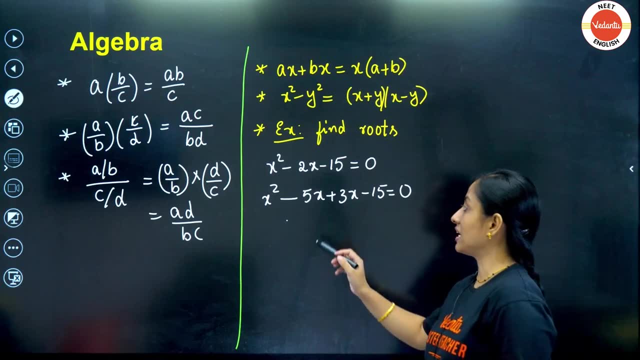 is equal to 0.. So first thing we need to find out for this constant: what are the multiples? Now, those multiples: if I add or subtract, will I be getting this answer or not? Select only those multiples. So minus 5 plus 3, I am getting minus. 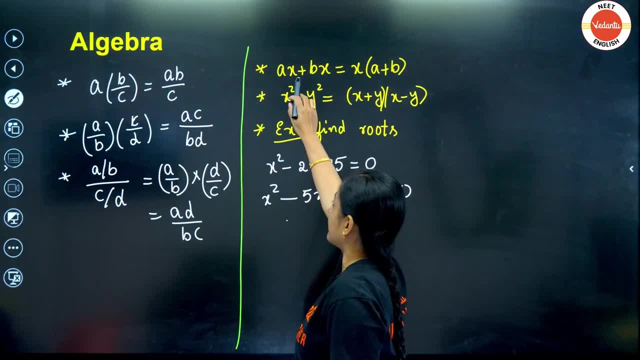 2X, So it is correct. Now take the common. However, we have written here the same thing. we are going to write, So X into X minus 5, plus here I can take 3 common. So 3 into X minus 5 equals to 0.. 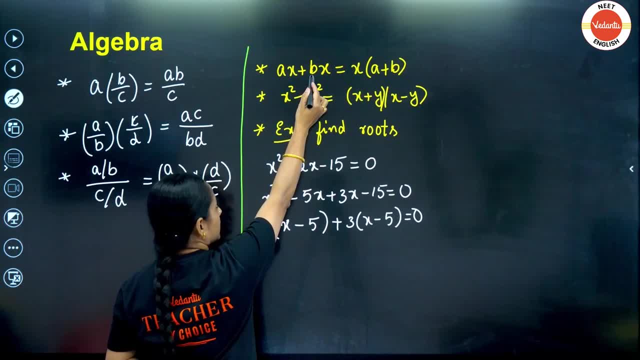 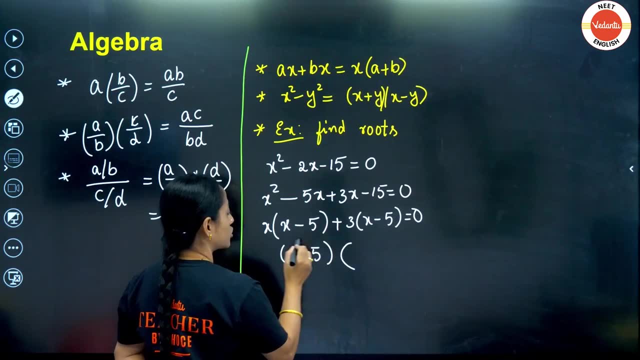 Now you can take out X minus 5 common. Same. this first thing only we are going to apply. Here there is an X minus 5.. Here there is an X minus 5.. Take out X minus 5 common, So you are left with X plus. 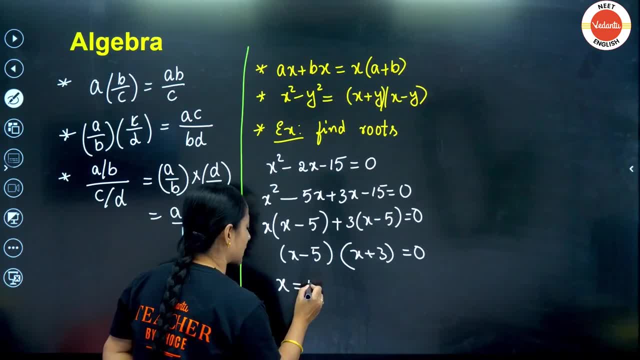 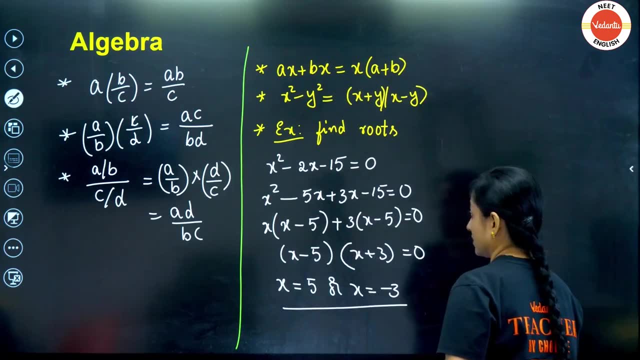 3 is equal to 0.. So what are the roots? Either X is equal to 5 or X is equal to minus 3.. So these kind of problems we will face in the physics solutions problem solving. So apart from this, there is one more method to find. 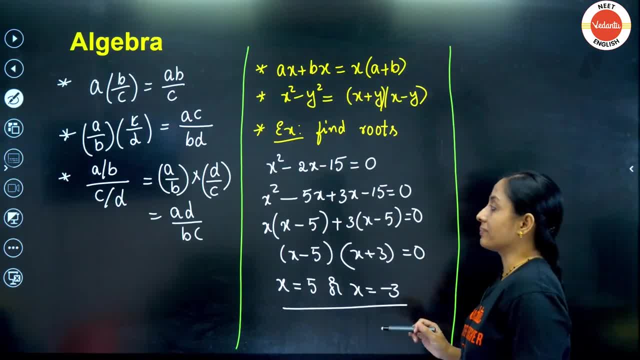 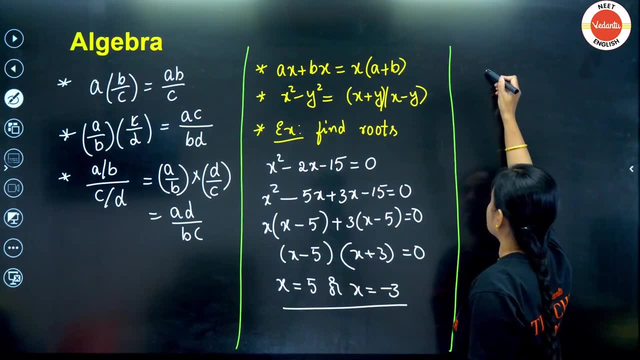 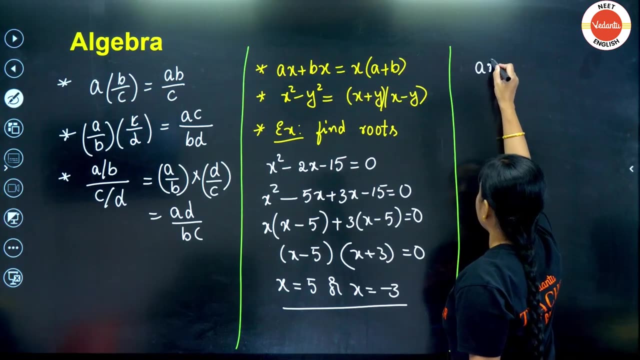 The roots. This is a general method, But apart from this, we have another method, that is, by using a formula- Direct formula is there- to find the roots. That formula is whatever roots you want to find out. For example, you are given equation like AX square plus BX plus C is equal to 0. So 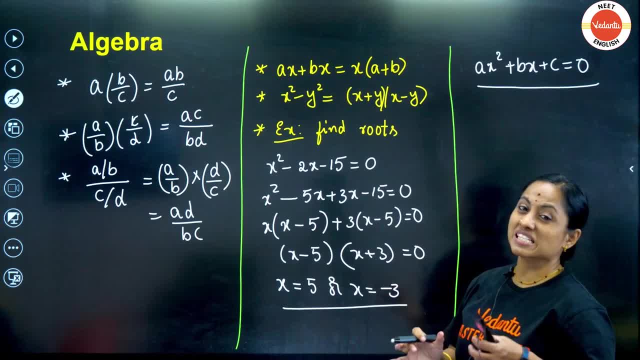 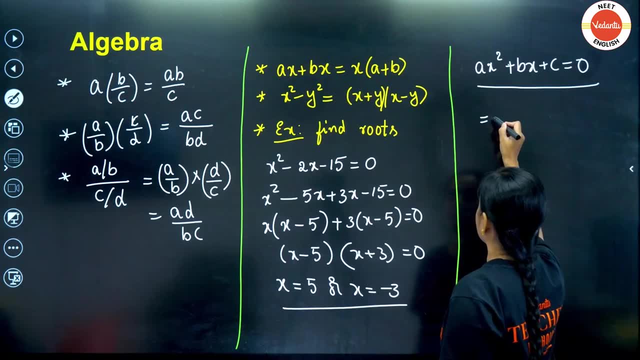 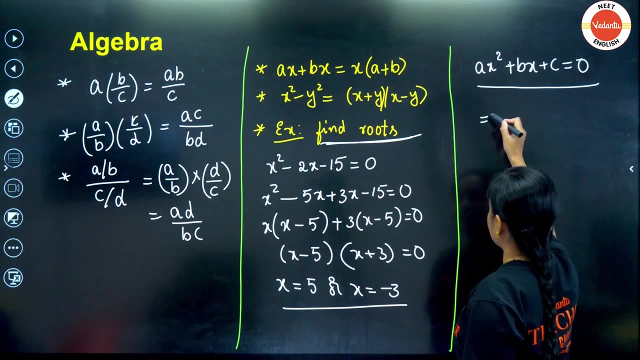 this is the same. See the method. the basic model is same. So the same thing, same formula. We have taken Now how to apply the formula. So how to apply the formula is to find the roots. Same thing. we are continuing to find the roots. What is the formula is? So the formula is X is. 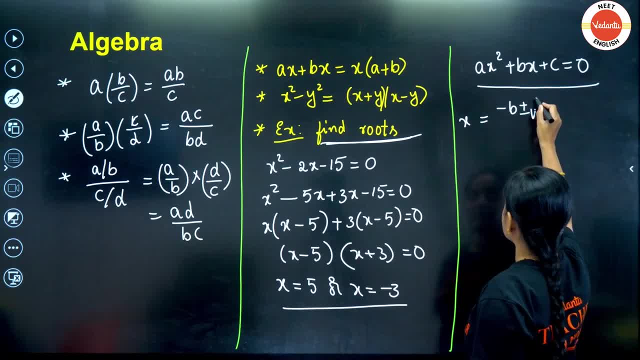 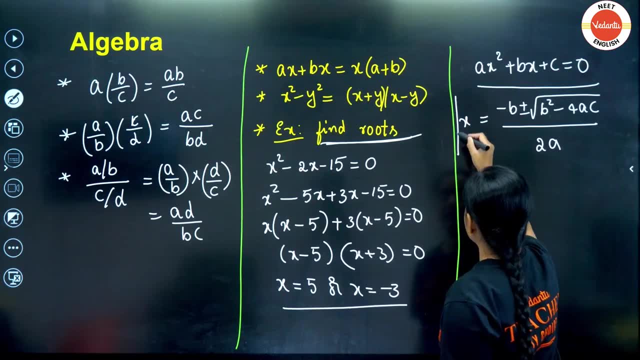 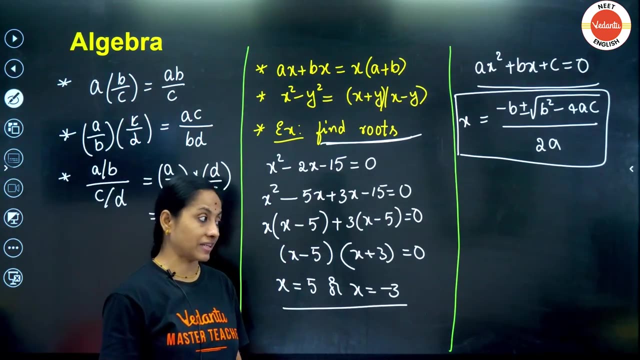 equal to minus B, plus or minus under square root B square minus 4AC by 2A. Very, very important formula, especially bio students. You might have learned in your lower classes but you might not know about it. But yes, do remember it because certain times, if you are not able to do this, 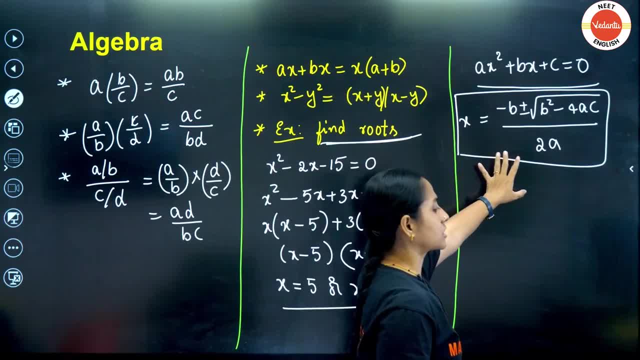 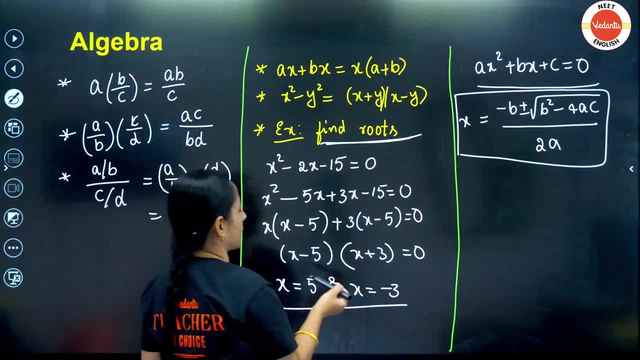 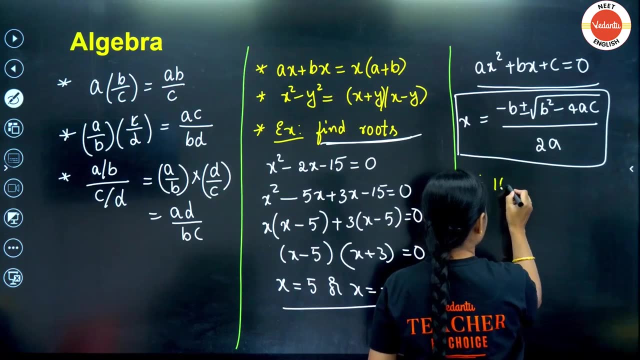 method, then no problem. Directly remember this formula and substitute. you will get very easily answers. So here, if I give you an example, if I want to give you an example, let us take an example and try. Can we substitute here or not? For example, you are given an equation like 10X square. 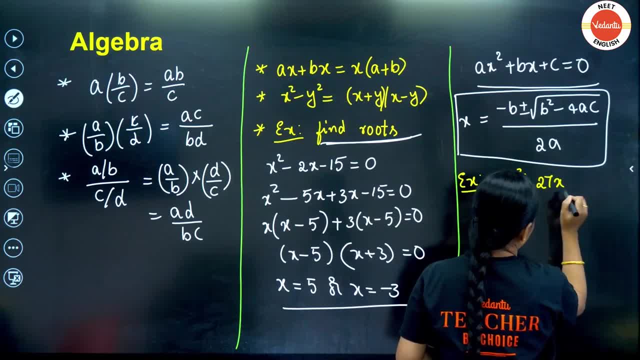 minus 27X, minus 27X plus 5 is equal to 0.. So this is the formula. So you have to find the roots. So this is the formula. So you have to find the roots. So you have to find the roots. So you have to find the roots, So 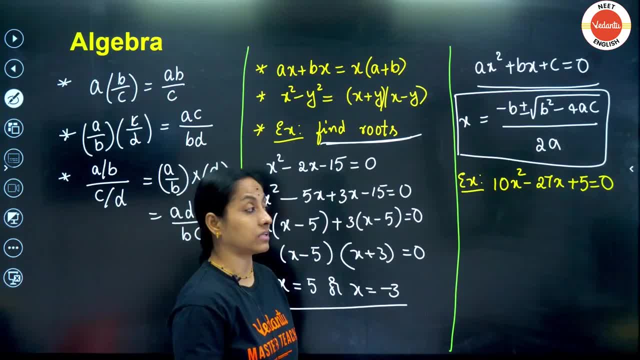 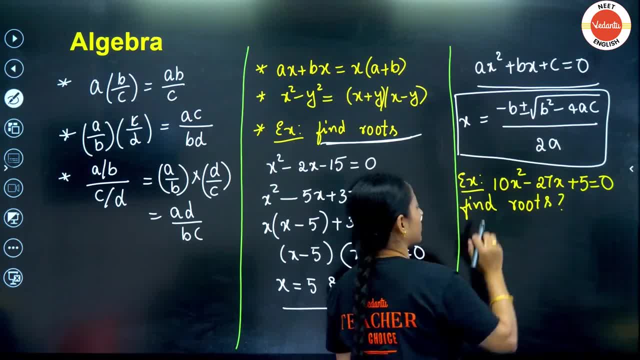 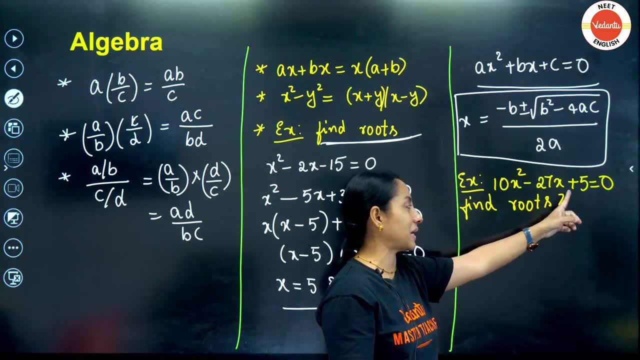 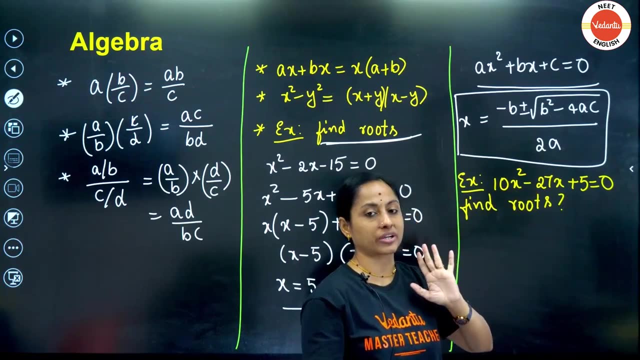 Okay, So find the roots. So how to find the roots? Direct formula. you can substitute, For example here, if you see this, for this: 5, if I want to find the multiples. this is not. I am not able to find the multiples of 5 as the addition or subtraction. If I do, I am not able to. 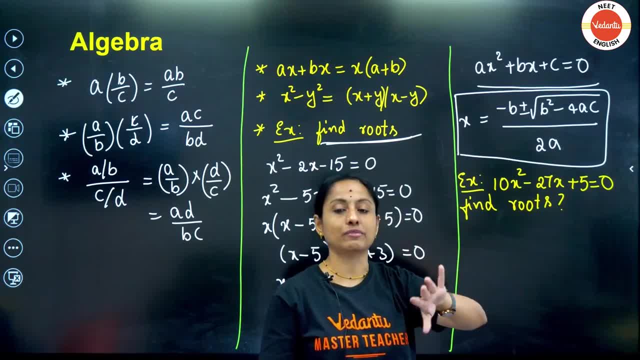 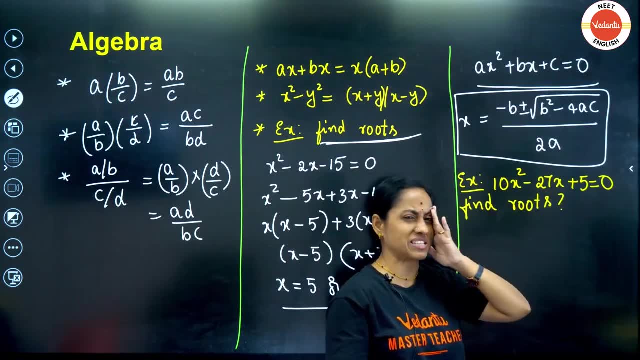 get 27.. 5 have multiples only: 1 into 5 or 5 into 1.. Right, But why is that? Why is that? Why is that 1 into 5 or 5 into 1, like 5 plus 1, 5 minus 1? i'm not getting 27, so it's very tricky, so let me use 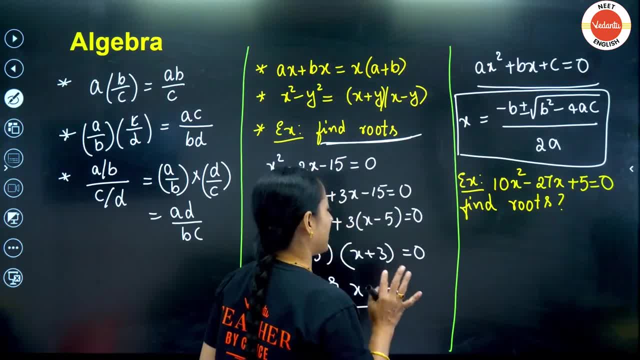 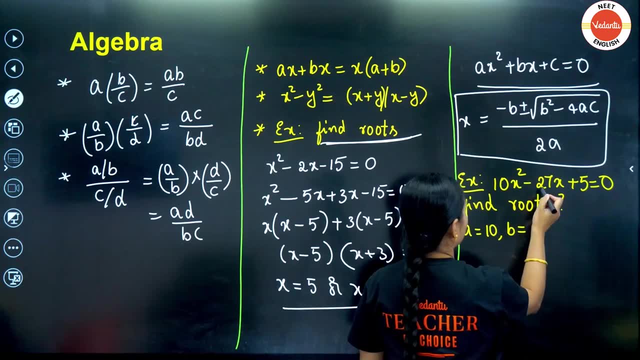 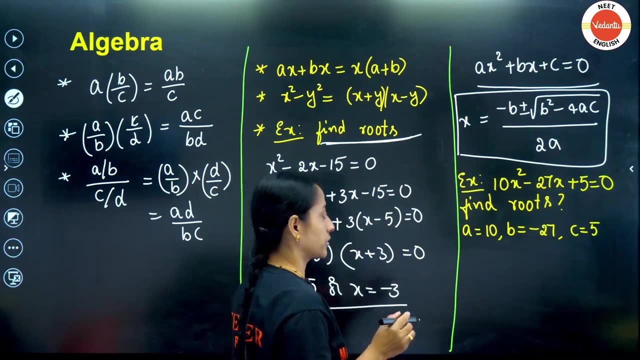 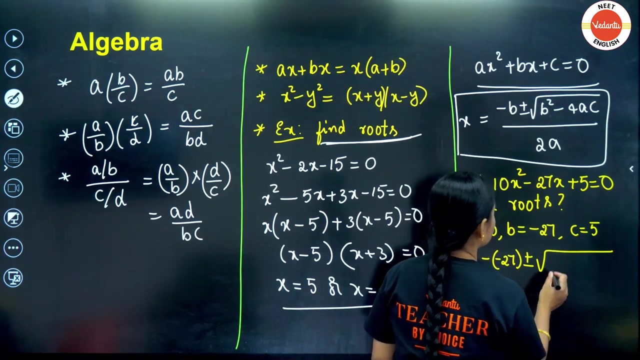 directly this formula. so just identify what are a, b, c in this formula. if you compare this with this: in this a equals to 10, then b equals to minus 27 and c equals to 5, just direct substitute. so x is equal to minus b. so minus of minus 27, plus or minus under square root: b square minus 27 square. 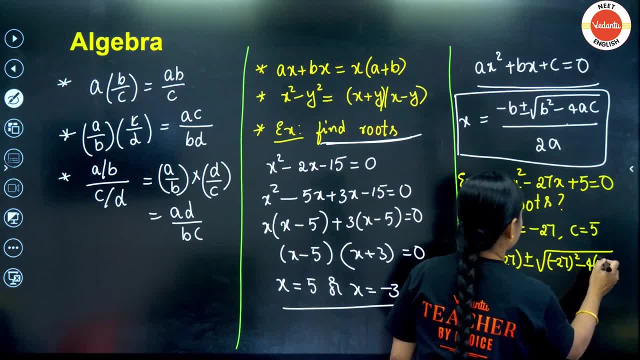 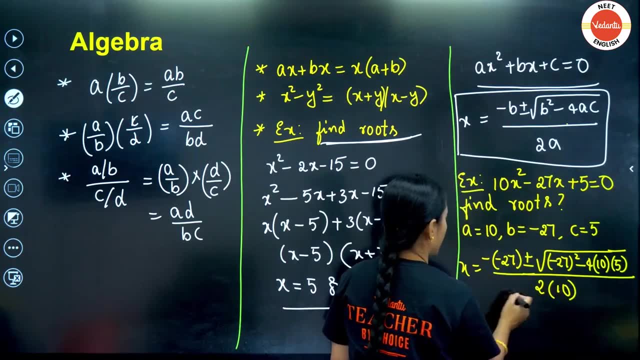 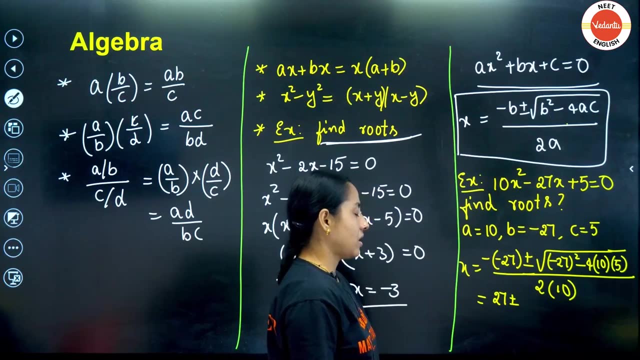 minus 4 a c, 4 into 10, into 5, by 2 a, 2 into what is a 10. so this we have to solve. so minus into minus, plus 27, plus or minus under square root, 27 square minus, how much? this will be 200. so 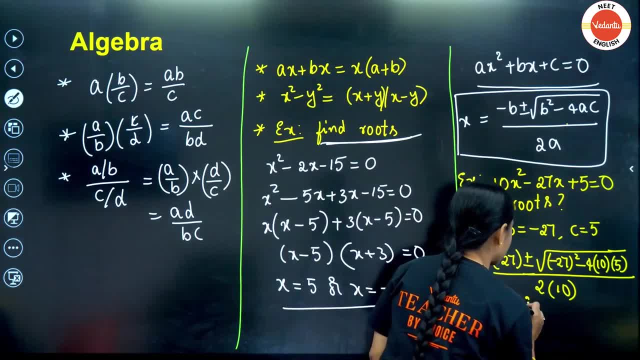 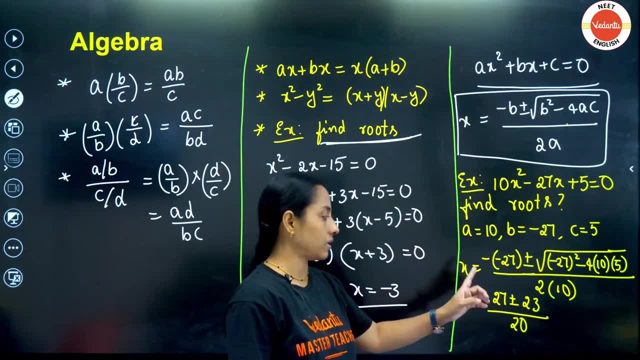 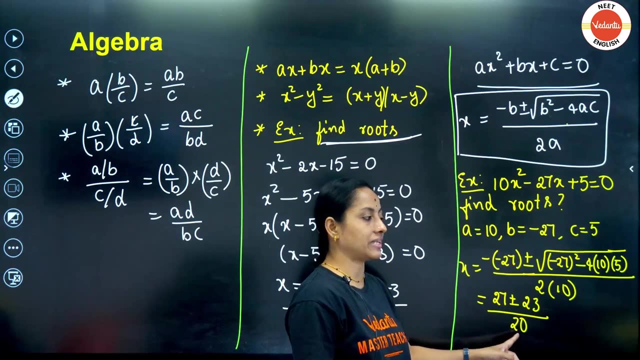 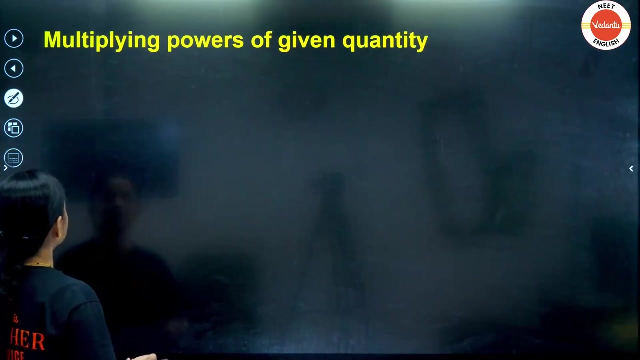 27 square minus 200 approximately, the answer will come out to be 23. by this is 20, so you will get plus one answer by using minus symbol. another answer if you are using plus 7, plus 3, 10, so 50 by 20. one answer is 5 by 2. so here, if i find the roots, i will get the answer as okay now. 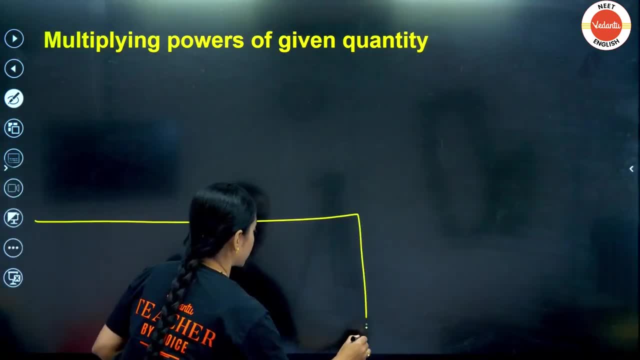 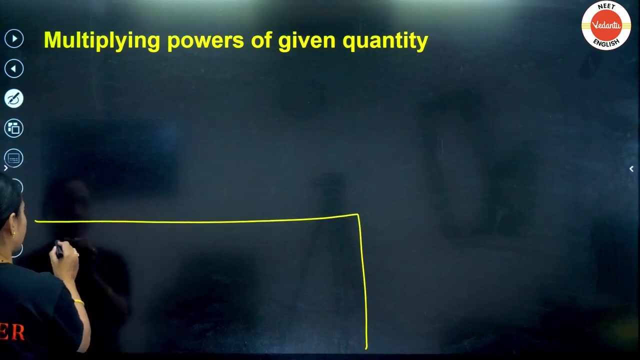 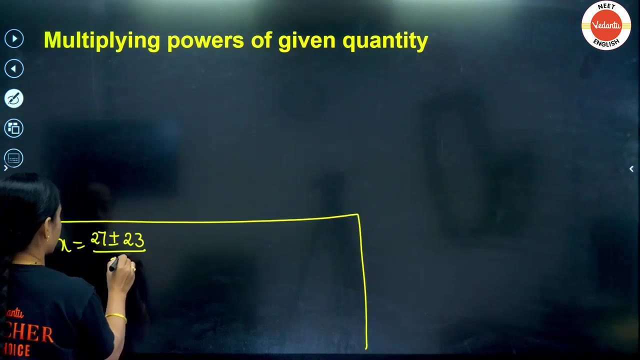 can i, can i solve here. so i'm just taking you this part. I am solving here the previous one only. So here, 27 plus or minus 23 by 20, right x is equal to 27 plus or minus 23. by what is the answer? we have 20.. So 27 plus 3, one root. 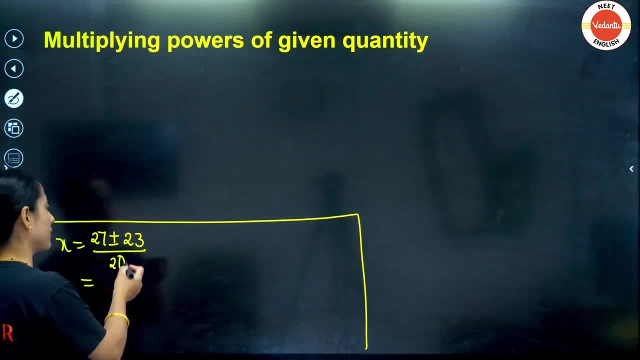 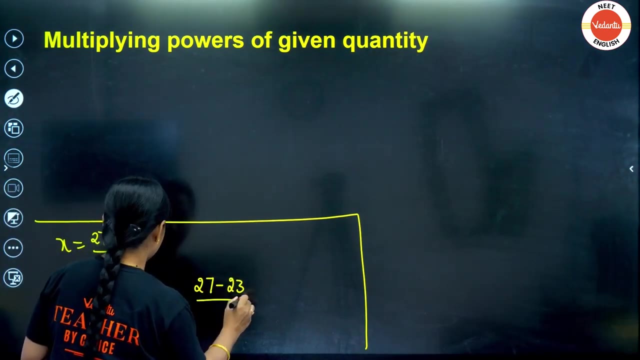 there are two roots right once. one root we will get by using plus symbol. another root we get by using the negative symbol. So by using plus symbol I get one root, 27 plus 23 by 20. another root I will be getting by using 27 minus 23 by 20.. Usually the roots are named as alpha and beta. 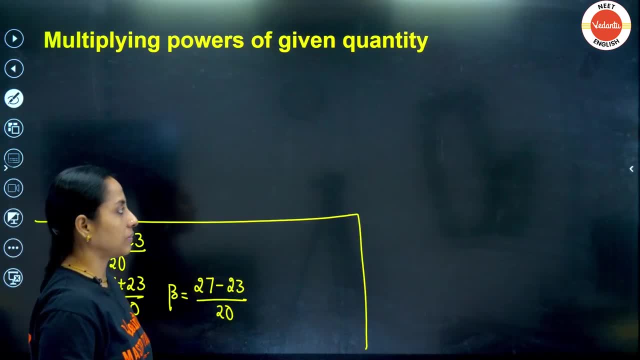 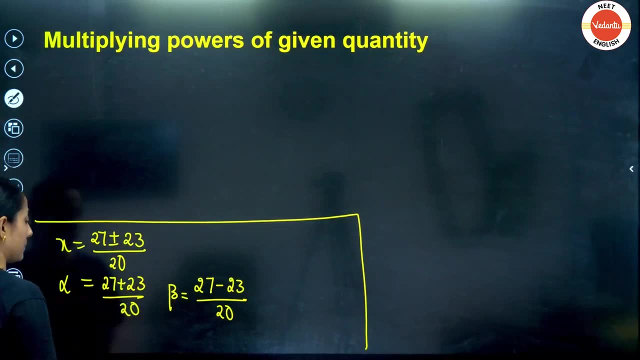 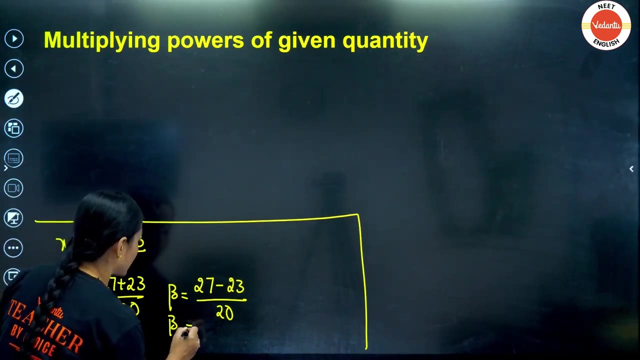 the roots. by using this formula, by using this formula, this formula, whatever roots you are getting those roots. usually they are named as alpha and beta. So alpha value you will get 15.. So 50 by 20, so 5 by 2, and beta value you will be getting 27 minus 3 is 25 by 20.. So it is. 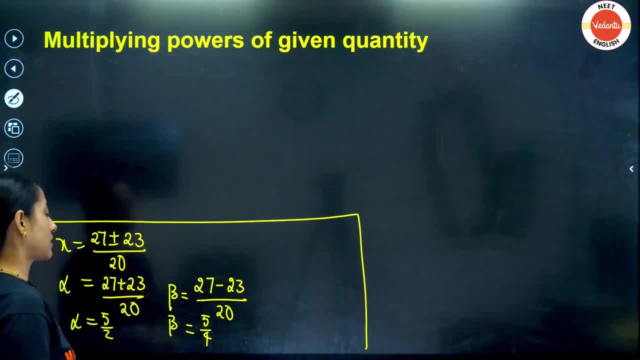 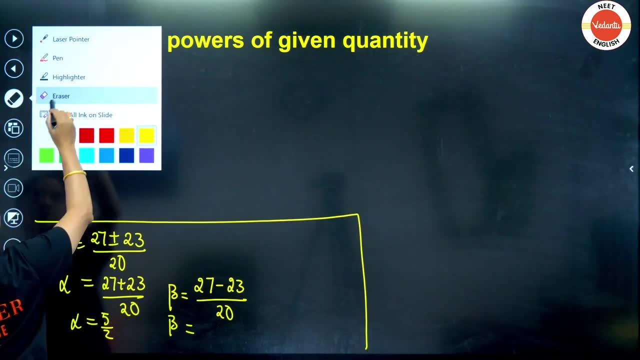 5 by 4, am I correct? So 7 minus 3, 4? no, I have got wrong, So this is not the answer. So, please, you can carry on with this: 27 minus 23. if you have a doubt, just check it: 27 minus 23 answer. 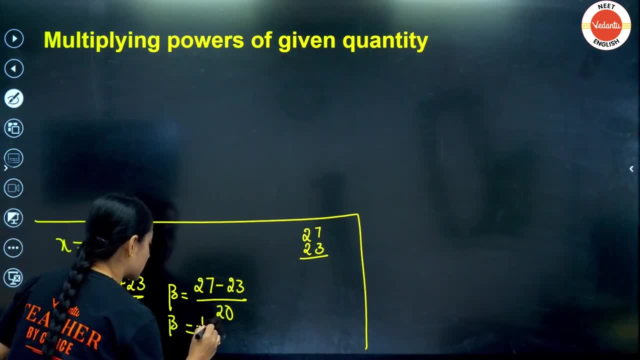 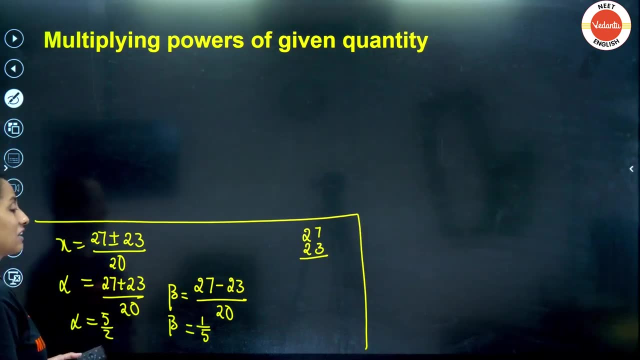 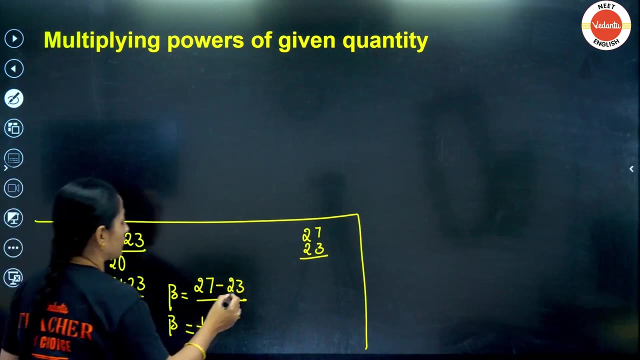 is 4. okay, 4 by 20.. So the answer is 1 by 5.. 4 by 20 is 1 by 5.. We have another checking also alpha plus beta value and alpha into beta value also you can check. So alpha plus beta value, alpha into beta value, alpha plus beta, if you do. 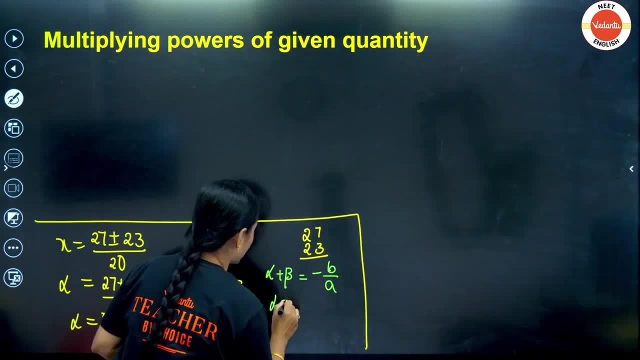 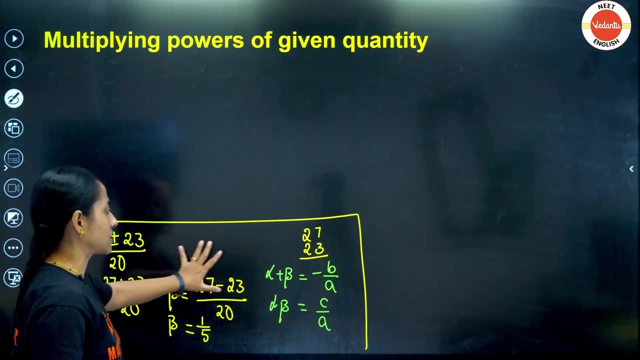 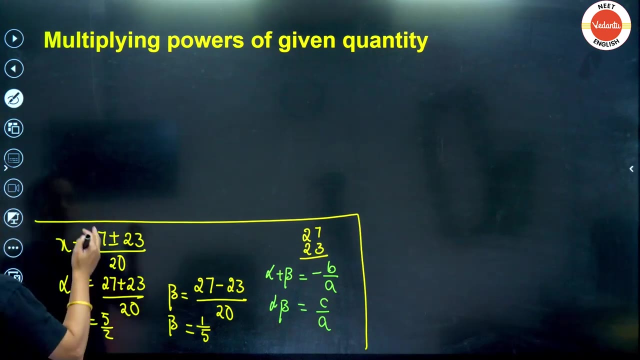 you have to get minus b by a and alpha into beta. if you do, you have to get c by a. So this is the checking part. So I hope you understood. this is the continuation part of previous slide. I did not take an extra slide, So please consider this Anyway. so next we will be going with another operation. 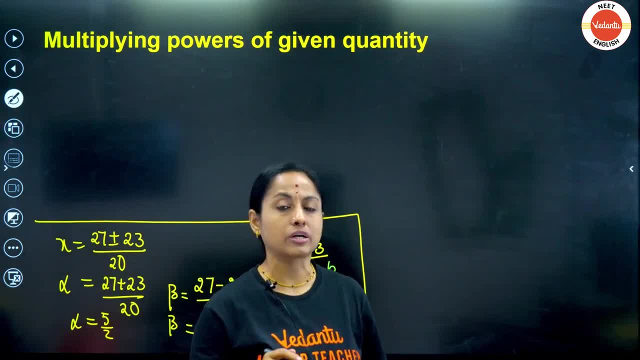 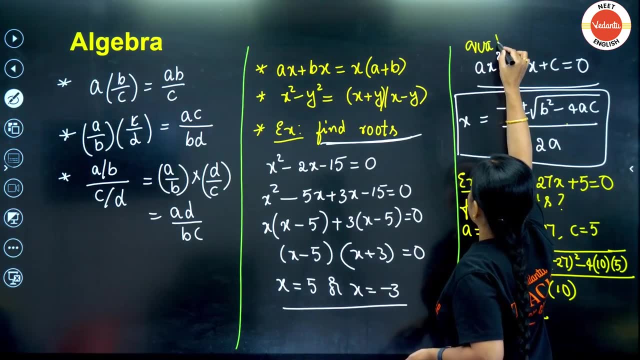 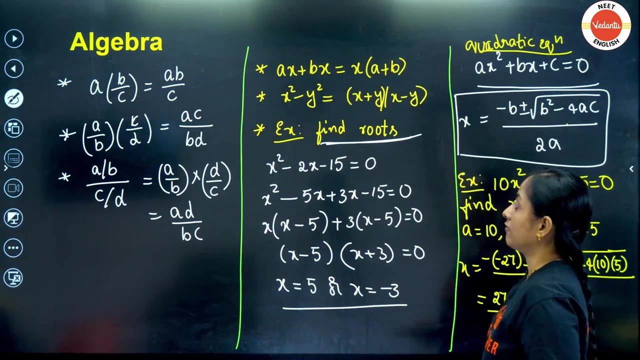 I hope now you are clear with algebra part. So how to find the roots of a quadratic equation. Whatever we have here, this is called a quadratic equation, So name also you can name, you can remember quadratic equation. So how to find the roots for a quadratic equation, either by using 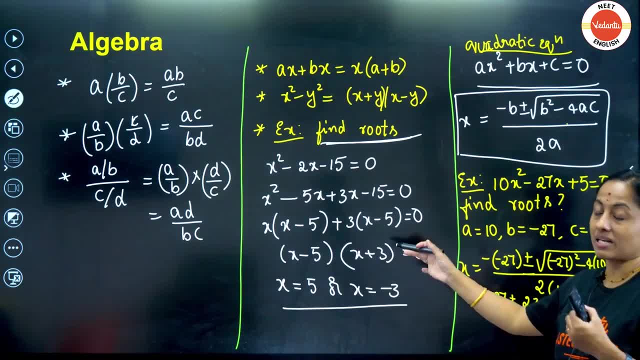 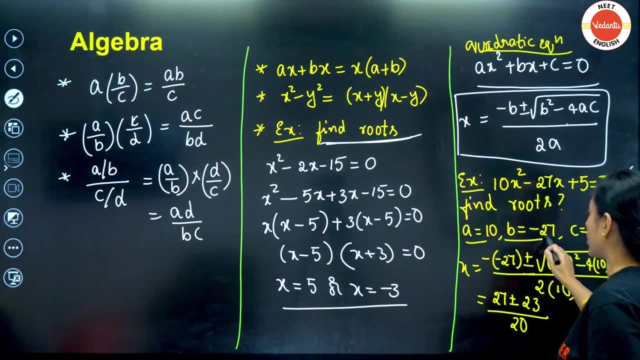 this method. If you are finding that this method is not comfortable- I'm not able to do it directly- go to the formula. So in the formula, first you think you need to do is identify what is a, what is b, what is c, then directly substitute in the formula. 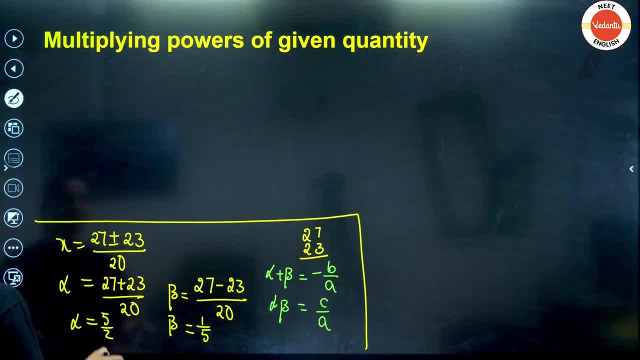 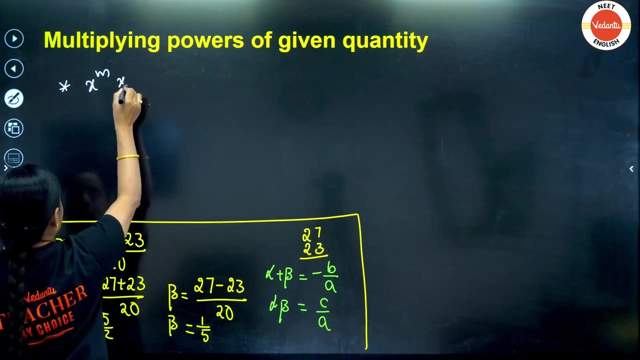 that will be done. Okay, moving on to the next mathematical operation: multiplying powers of given quantity. This is a very simple thing, you already know, but usually people get confused with the ten powers whenever they are. So multiplying powers is nothing, but if you have x power, m x power. 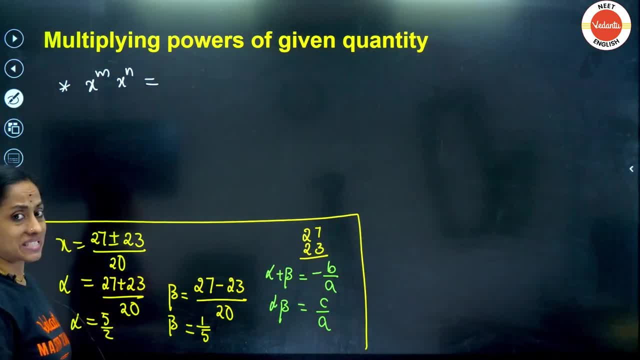 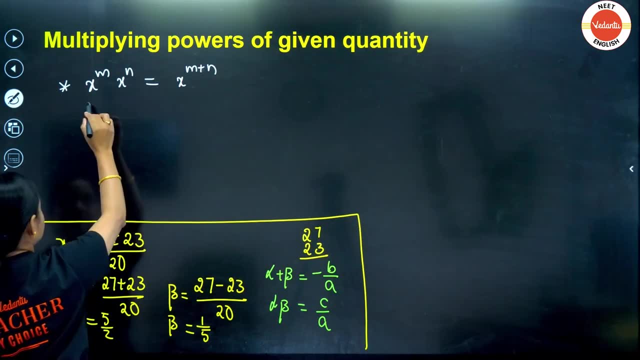 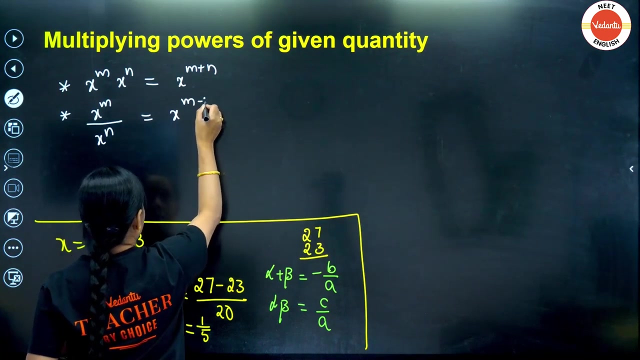 n bases are same. when bases are same, then the exponents get added up. x power m plus n bases are same and they are in product, then the exponents get added up. otherwise now x power m by x power n in the division, when bases are same, the exponents get subtraction, because you know, 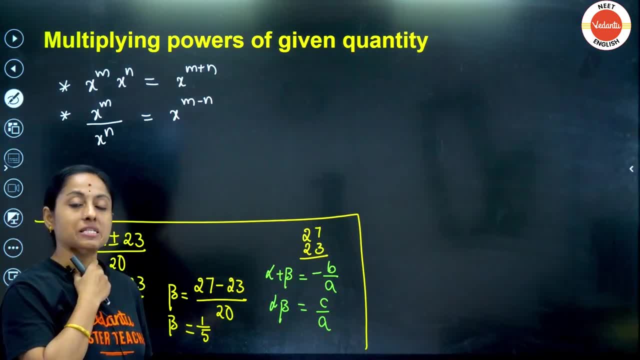 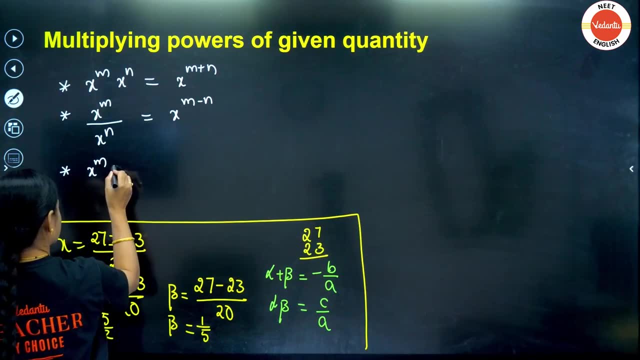 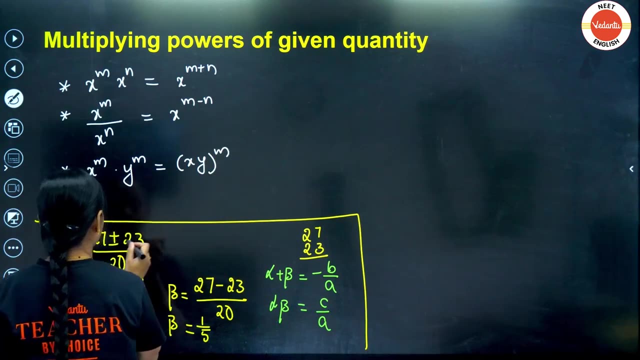 that when x power n is taken to numerator, it becomes x power minus n, so x power m minus n. similarly, if you have x power m into y power m, so we can simply write this as x- y whole power m. similarly, x power m by y power m can be written as x by y whole power m. so these all things you. 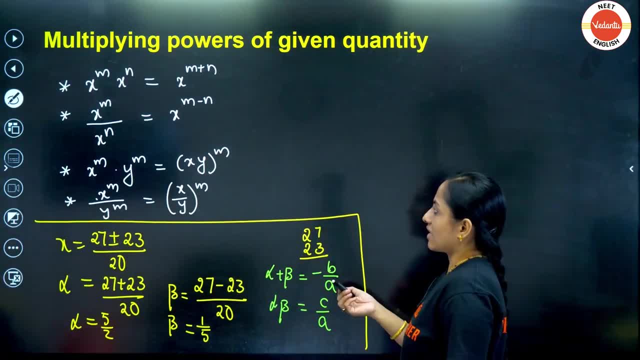 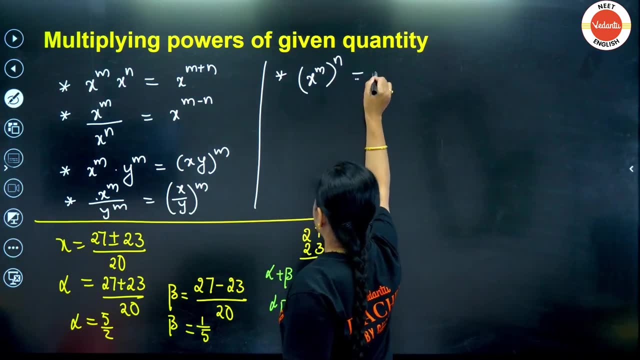 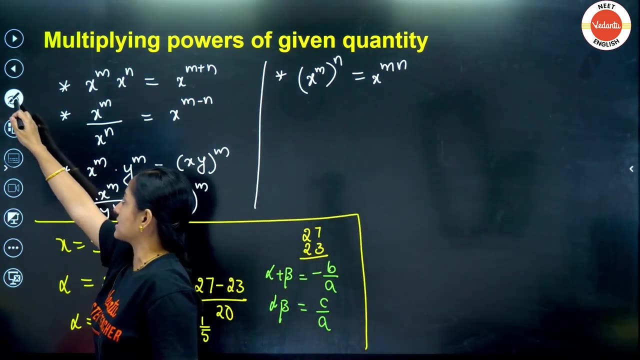 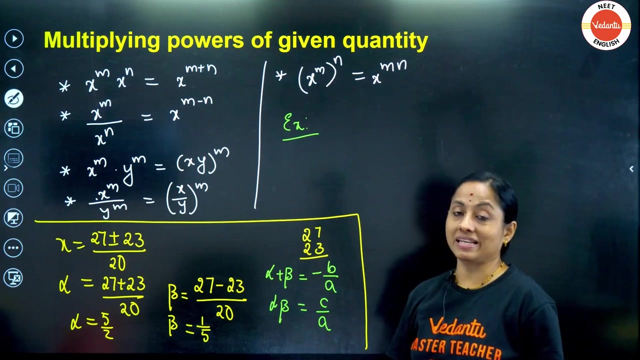 already know, but just a reminder kind of thing. so these are exponents we have. similarly, if we have x power m whole power n, x power m, whole power n, then the answer becomes x power m into n. let us take some examples and see how these works. the examples mostly: in physics. what we do is 10 powers. we deal with 10 powers. 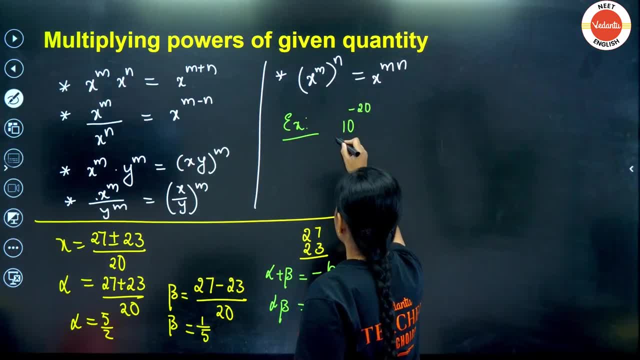 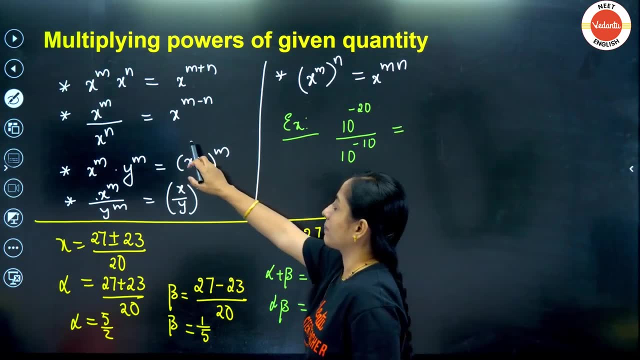 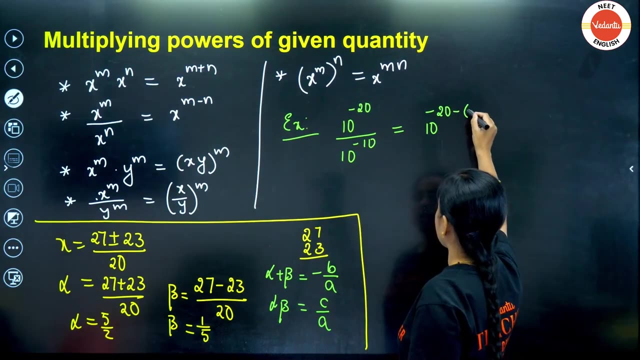 for example, you have 10 power minus 20 by 10 power minus 10.. so this, this you have to solve. so for that first thing, we need to apply this formula. so 10 power minus 20 remains the same when this comes up: minus of minus 10, because it is: 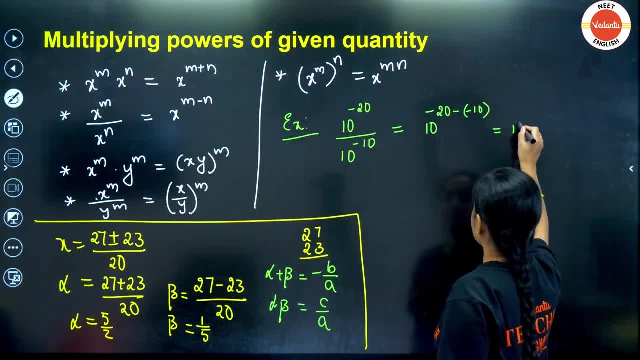 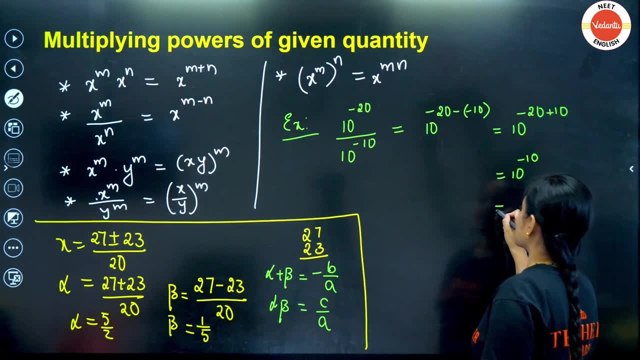 m minus n. so m minus n, the answer becomes 10 power minus 20 plus 10. the answer is 10 power minus 10. so 10 power minus 10 can also be written as 1 by 10 power 10. so this is how we use. 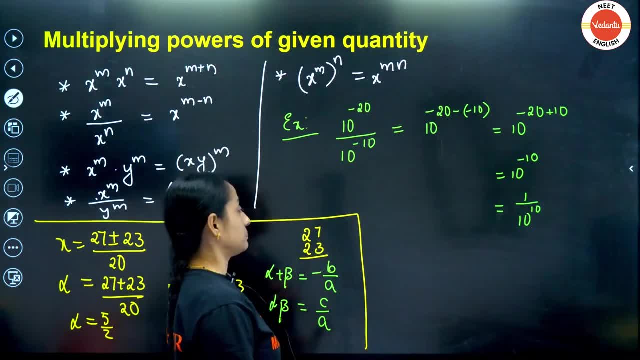 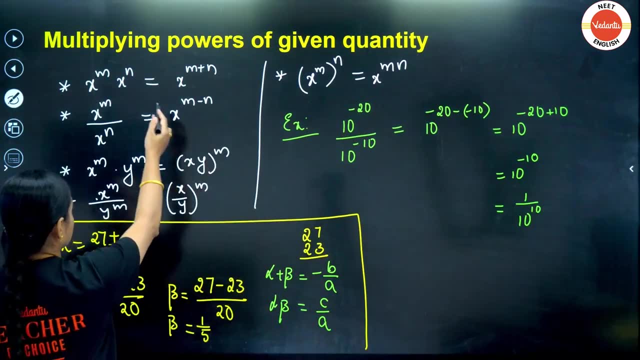 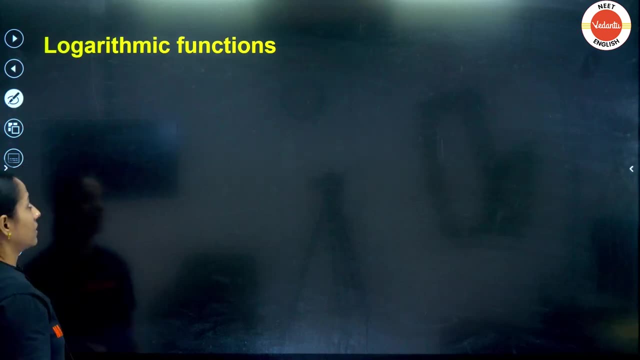 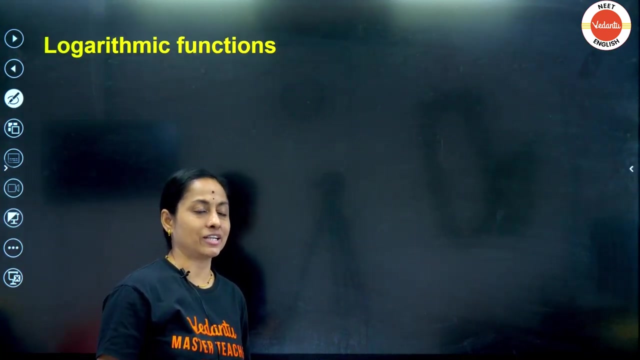 the multiplying powers in the given equation or given quantity. so, especially with the 10 powers, when you are dealing, be very careful. this part of mathematics is used now. moving on to next. yes, logarithmic, sorry, logarithms, logarithmic functions, logarithms logs, usually bio. people tend to forget because they don't use much of logarithms in their bio or anywhere: chemistry. 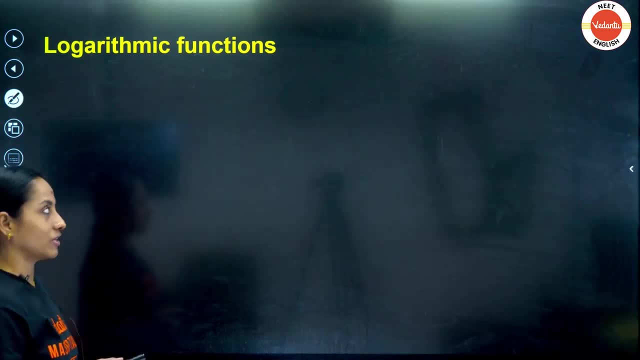 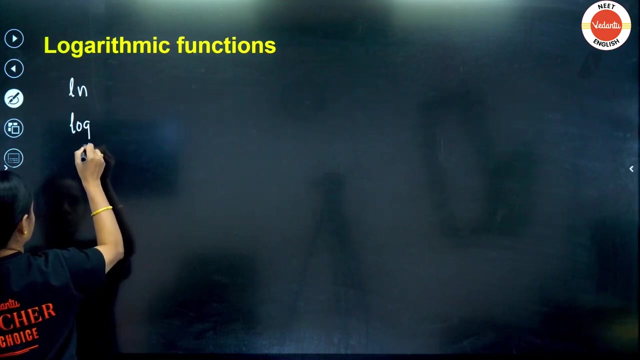 also very less, i guess, but yes, in physics we use a lot. so logarithmic functions. you have to learn now logarithmic functions, how there are two varieties. basically, we'll go with a very simple version. there are two varieties: one is ln and the other one is log. okay, how is ln written? as if it is. 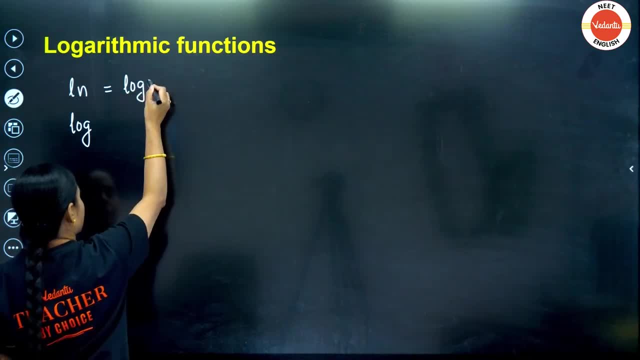 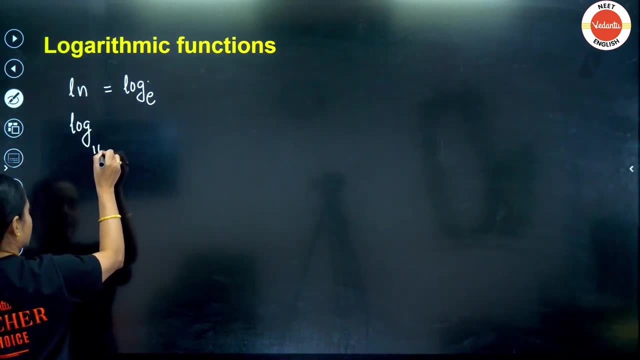 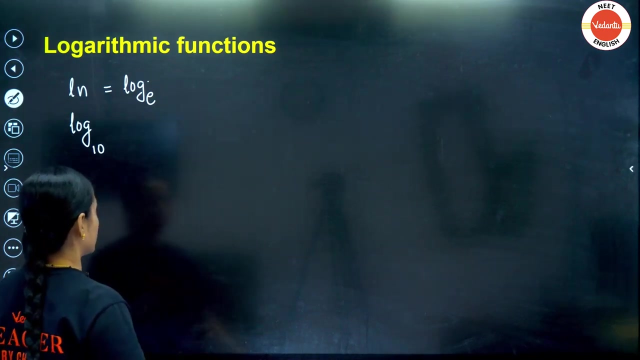 written ln. this means log some x, some whatever log to the base e. here some number will be given, so this line like this: this is base 10. okay, so we have two types of logarithms: logarithm with base e and logarithm with base 10.. so logarithm with base e is called as natural log. it is also called as: 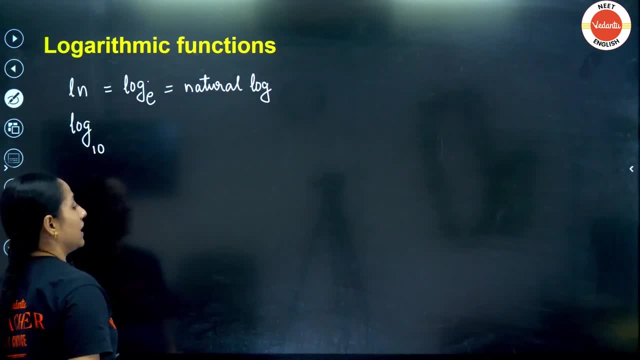 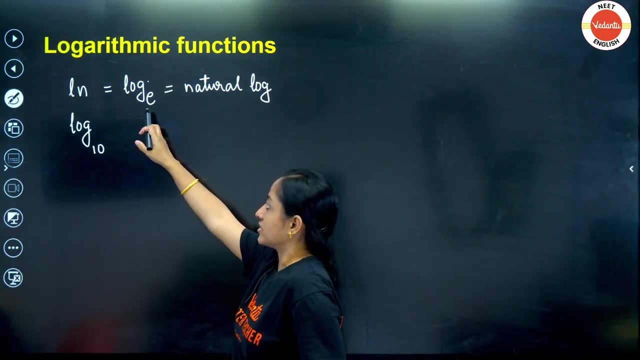 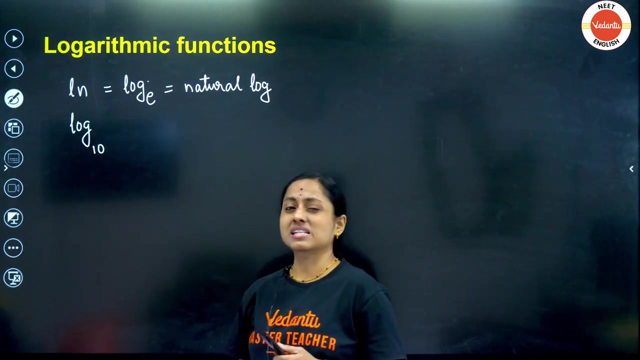 natural log. that is why it is written l n, l n, meaning natural log. okay, so natural log or logarithm with base e. this is written as natural log or logarithm with base e. both have same meaning: this. this is the point. see, that is how people usually feel that physics is. 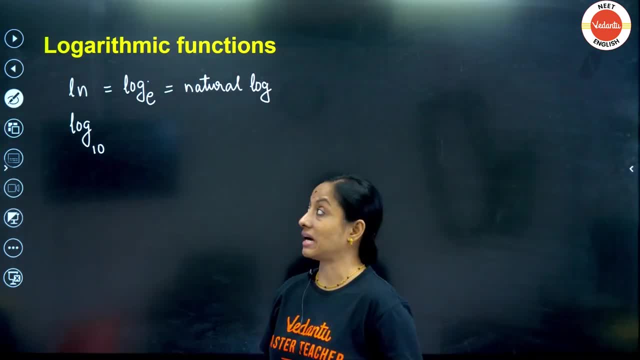 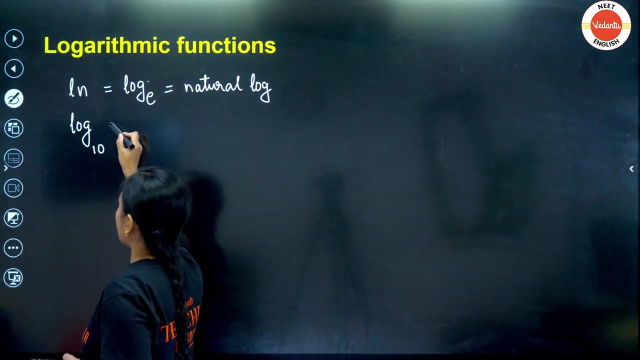 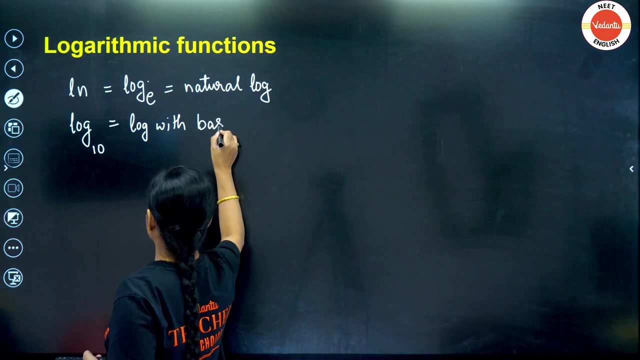 tough because many people don't even know the difference between ln and log e. there is no difference. first of all, they don't understand what is this ln used. so ln is nothing but natural log. okay, so natural log or log to the base e. next, log 10 is read as log with base 10, log with base 10. 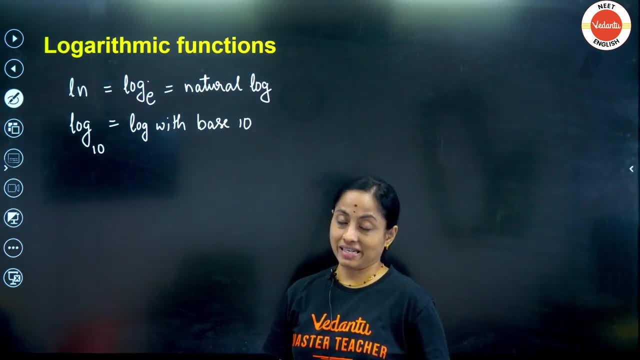 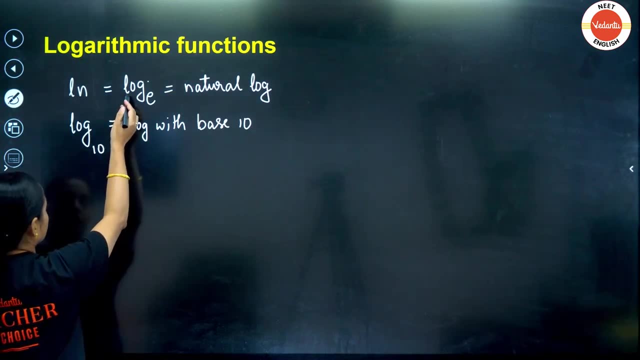 so we have two types of logarithms: logarithm with base e and logarithm with base 10. now if i want to convert these two, there is a conversion. also, how can i convert ln into ln? i mean log 10 as ln or log to the base e can be. 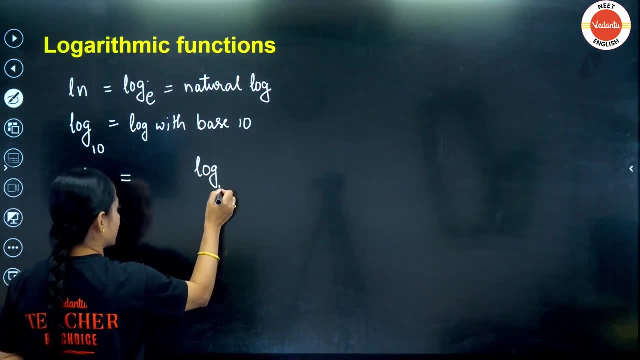 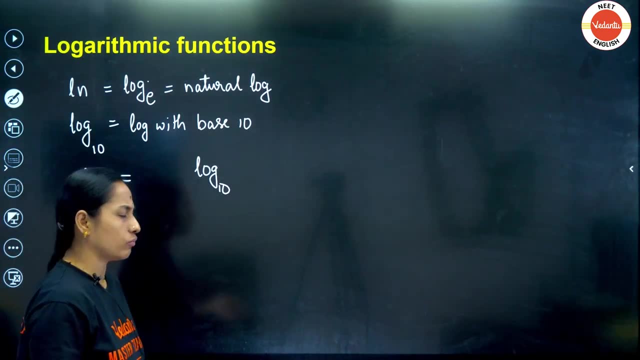 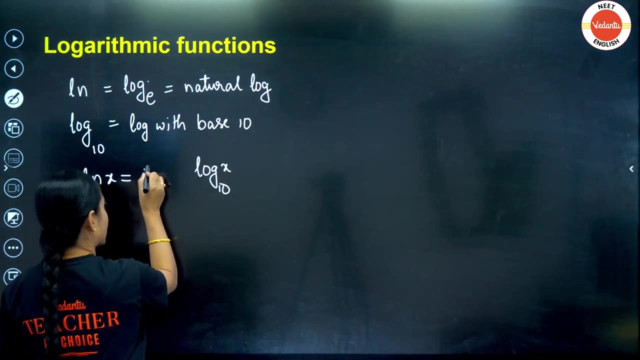 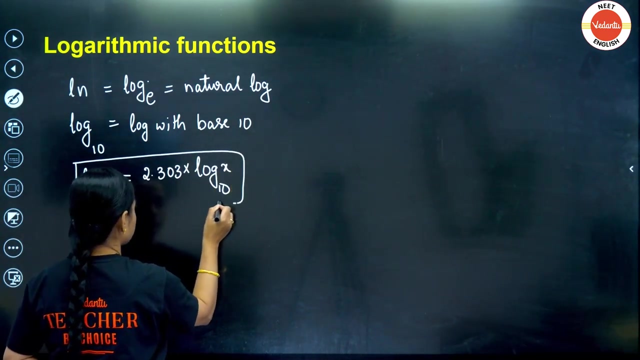 converted into log to the base 10, for example ln x. let us take some x quantity: ln 2, ln 5, ln 10, ln. whatever natural log of x can be converted into log x to the base 10 by multiplying with 2.303- it is a constant- by multiplying with the. oh, i have written the reverse way. 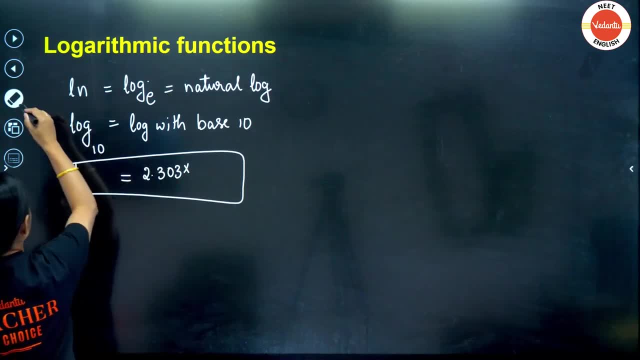 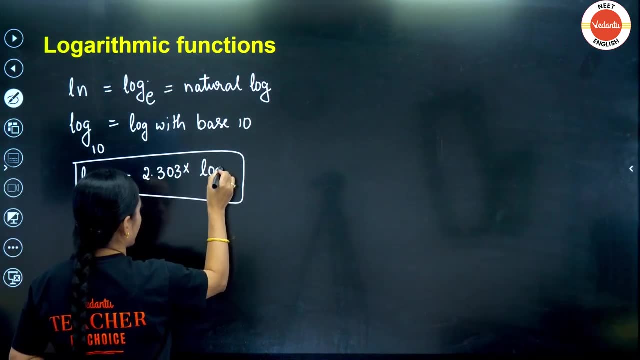 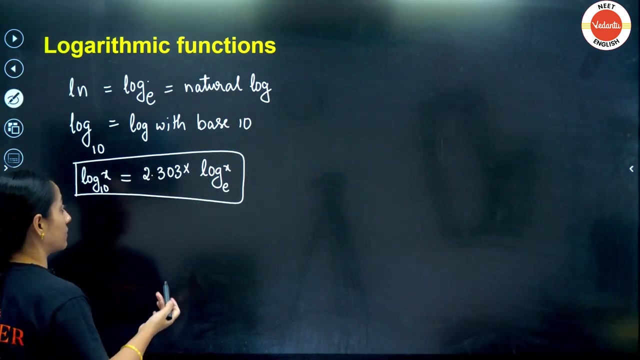 sorry, sorry, sorry. I have to convert it into log. then okay, log x to the base e by multiplying log mully. same thing I have written. log x to the base 10 can be converted by log x. base e: by multiplying natural log with 2.303 you can convert it into log to the base 10. so if you want, 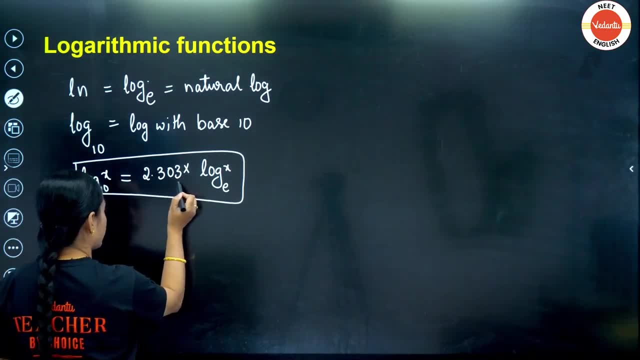 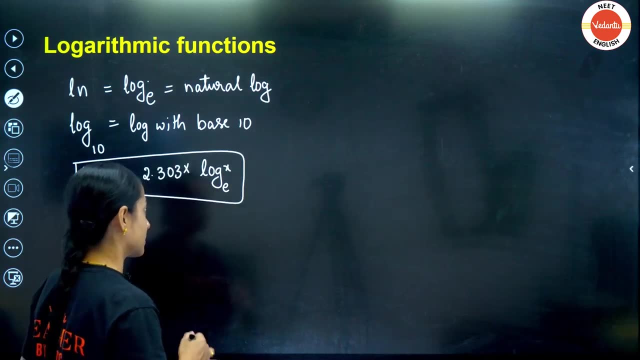 to convert to log to the base 10. this is a standard value. you can convert it to log to the base 10. this is a standard value. you have to memorize it. yes, many of today's class formulae. you have to memorize it, okay, so please. 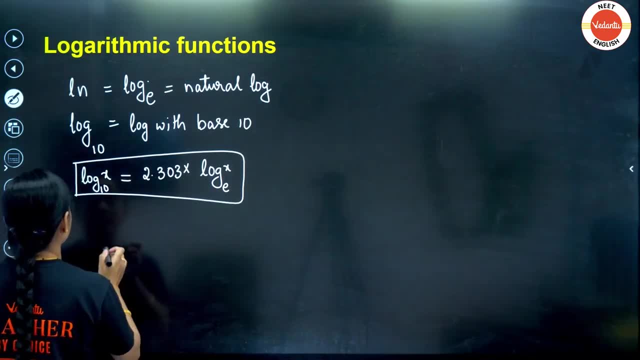 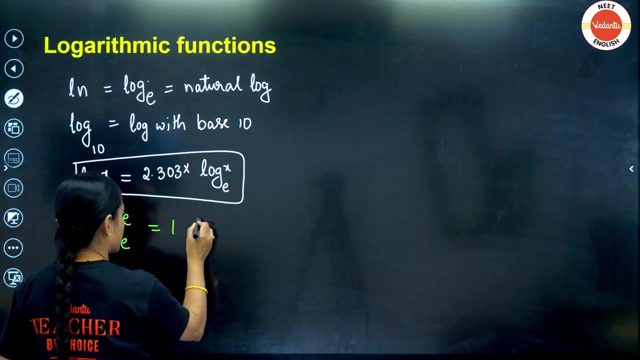 make a note of all these things. so this is a very important conversion. now, coming to other formulae, if you want to go with the other formulae, log e to the base e value is 1. log e to the base e value is 1, or simply, or simply, you can write ln. e value is 1, okay, next. 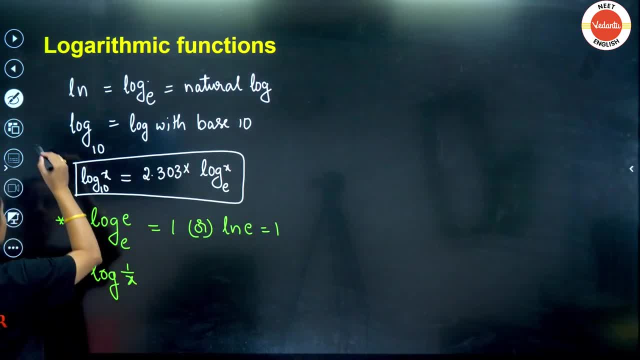 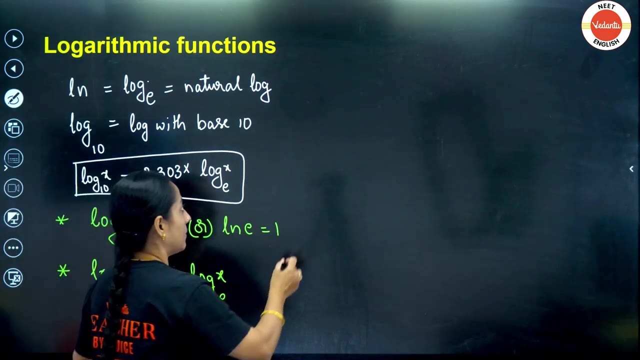 log 1 by x value. or I'll tell you first another formula that would be easier for you. okay, log x to the power n base e can be written as n into log x to the base e. whatever power is there, that becomes the multiplication. okay, these are all various formulae that we will be using. so how these? 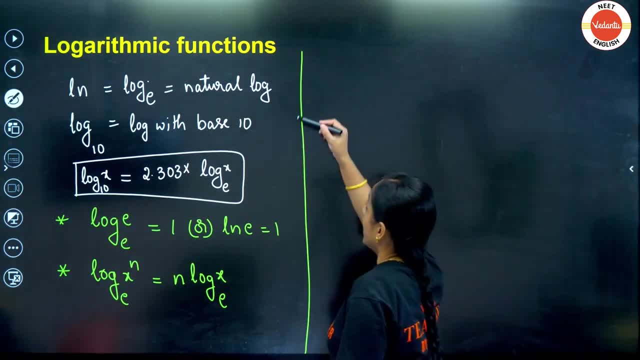 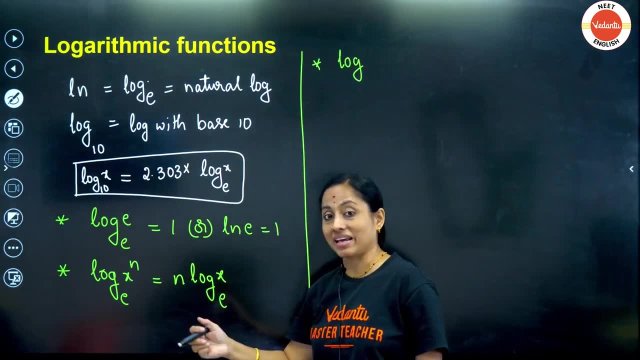 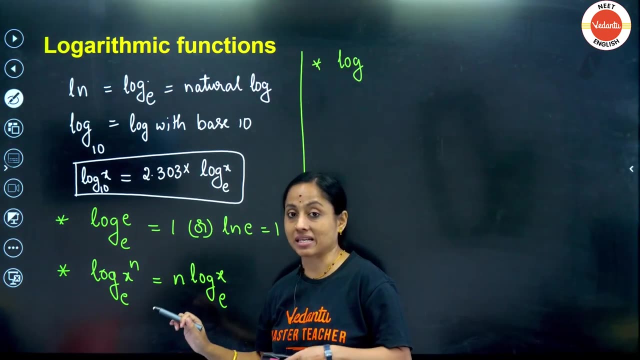 formulae have come into existence. all those derivations are not required. but yes, you do have to memorize all these things. Next, when I am writing for base e, the same is applied for base 10. also. when I am remember whatever formula we are writing for base e, the same thing is applied for base 10 also. next, 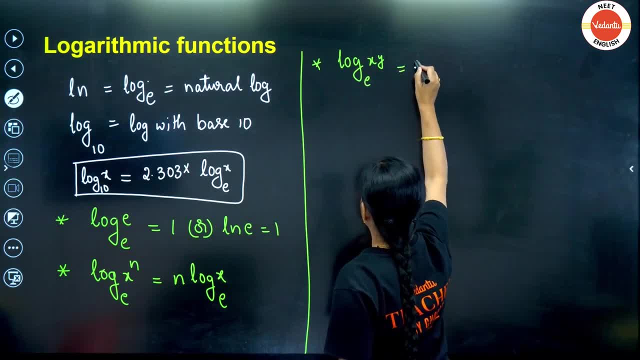 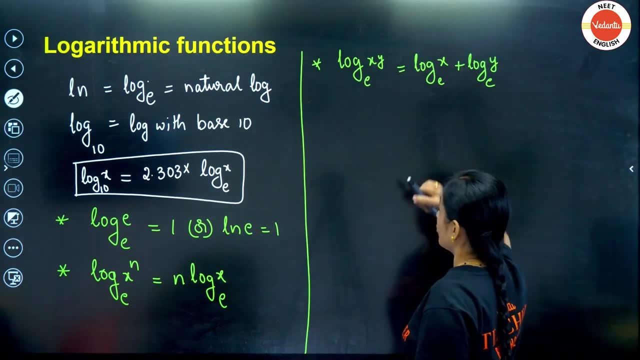 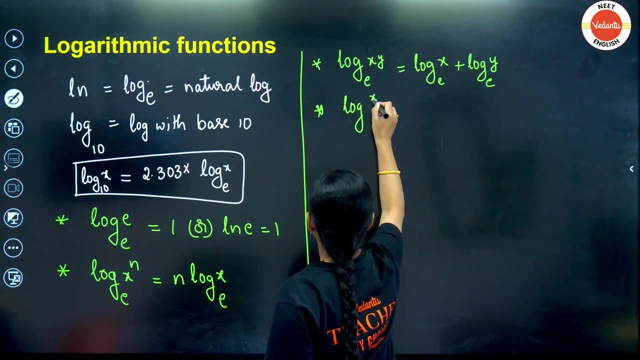 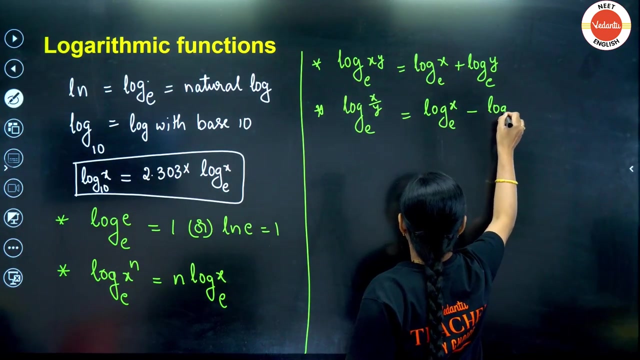 log x into y to the base e is equal to log x plus log y. okay, so we can. multiplication becomes addition and similarly, log x by y to the base e can be written as log x to the base e minus log y to the base e minus symbol. 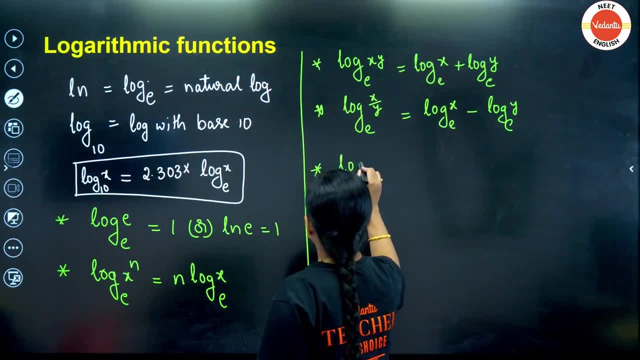 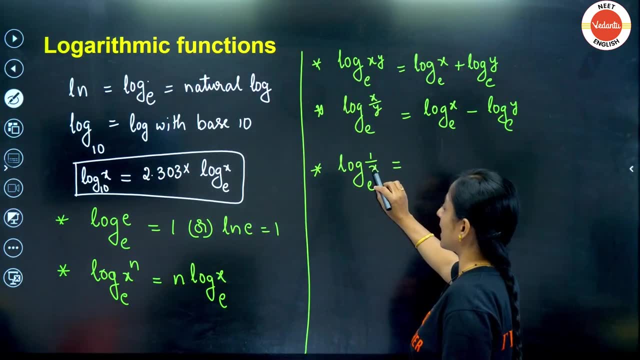 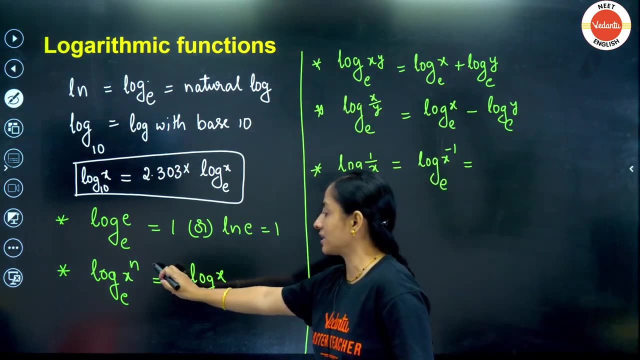 comes because the formula that you can apply here is log 1 by x to the base e. if I write the answer is actually how to convert: is log x to the power minus 1 to the base e. so minus 1 exponent becomes multiplication. so minus 1 becomes multiplication. so minus log x to the base e. 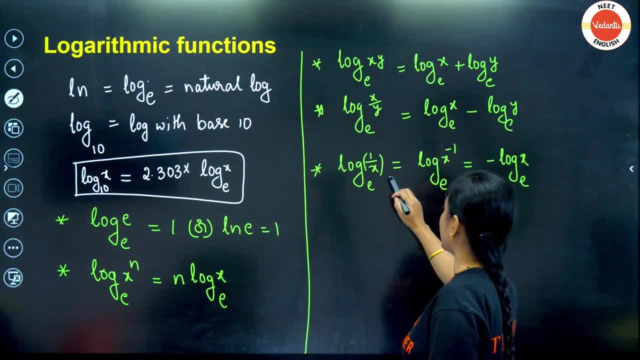 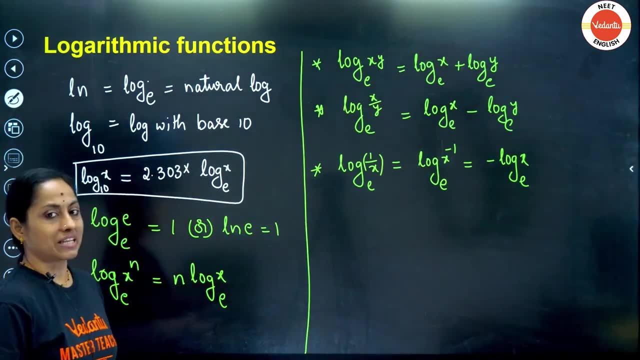 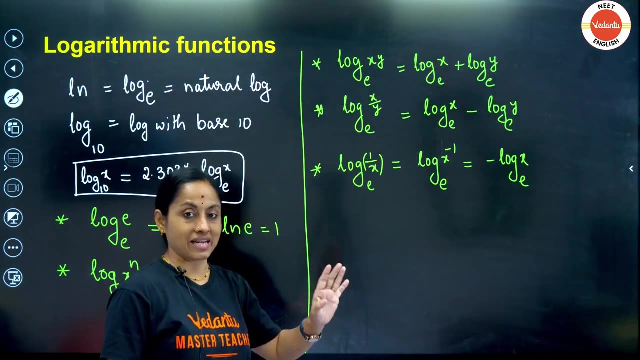 so whenever 1 by x, you can see, simply you can directly write this formula. so these are various formula we have in logarithm, so these are all. see. please do remember that whatever formula I have written for base e, the same formula is applied for the base 10 also, okay, so if you just remember that. 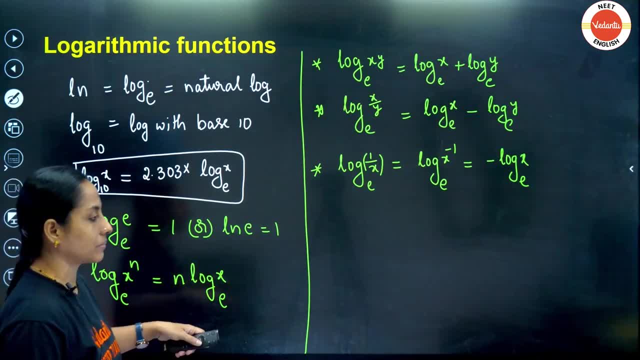 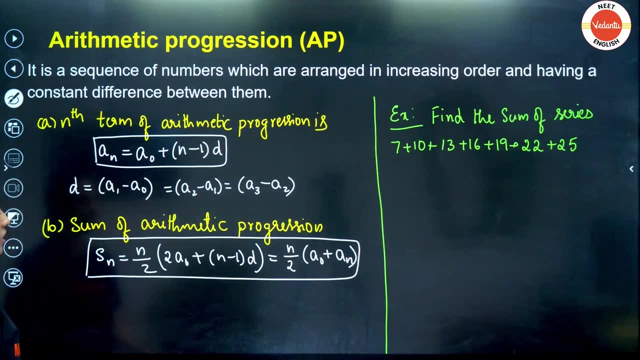 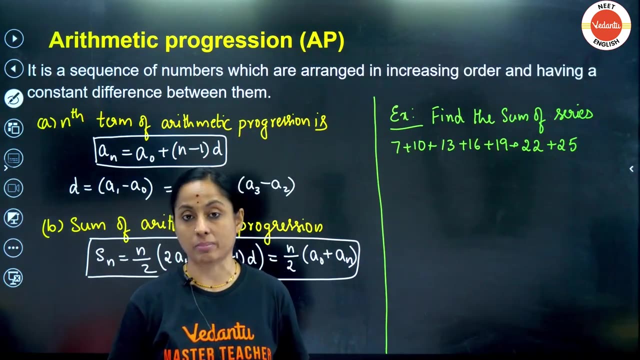 any logarithmic function you can operate. so these are the logarithmic functions you have to remember. next, moving on to arithmetic progression. so arithmetic progression, geometric progression, are the two things we will be using, especially when you are doing gravitation problems and electric charges and fields potential. these 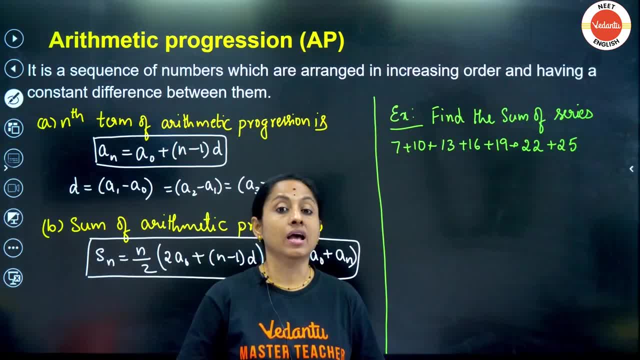 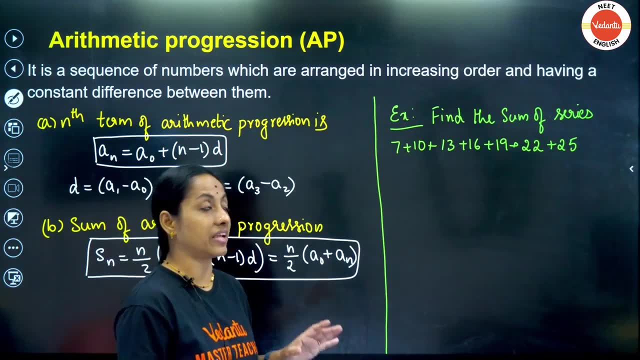 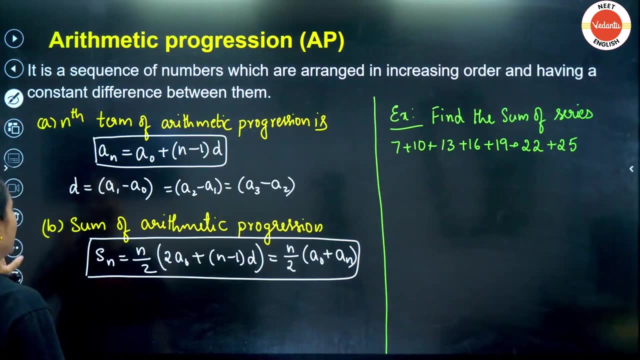 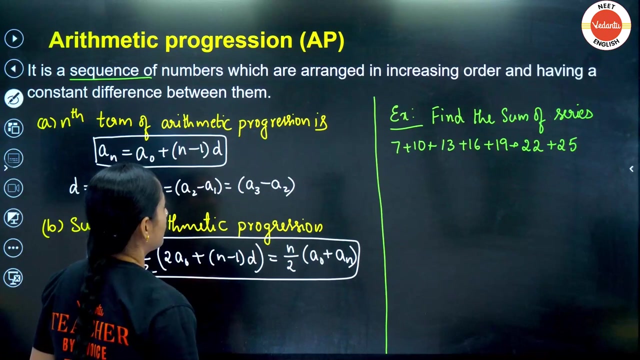 areas in first year, gravitation, especially in second year, electricity problems. you can take static electricity. so there, when you are solving certain problems, we have to use this arithmetic progression and geometric progression. so let us see what is arithmetic progression. it is a sequence of numbers, first of all progression, whenever the word comes. it is a sequence of numbers which are: 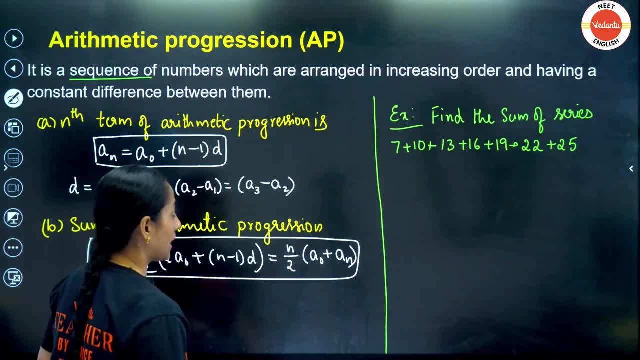 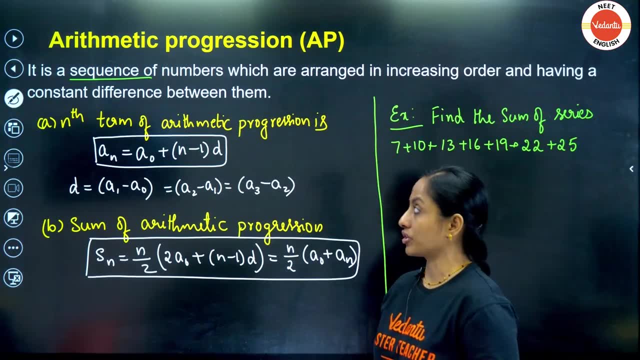 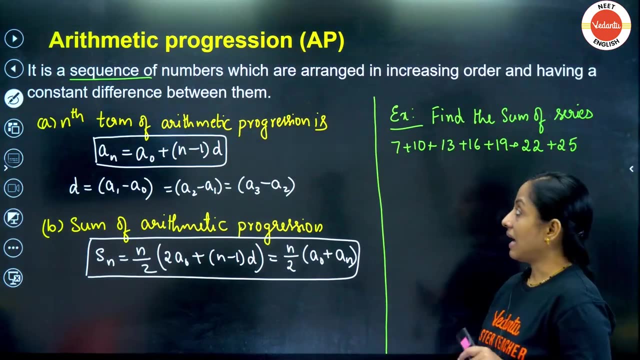 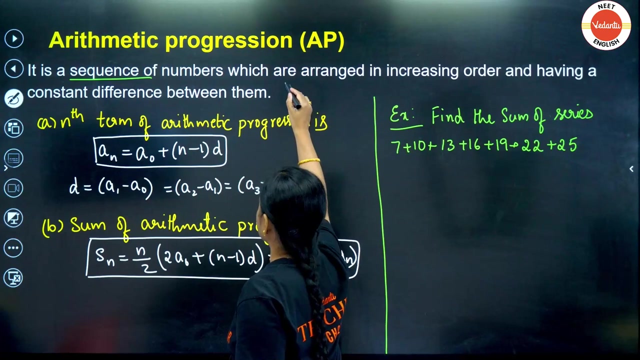 arranged in increasing order and having a constant difference between them. so that is the rule. when can you apply the arithmetic progression? you can apply arithmetic progression only when the numbers are in a sequence and they have to be arranged in increasing order and there should be a constant difference between them. let us take an example. 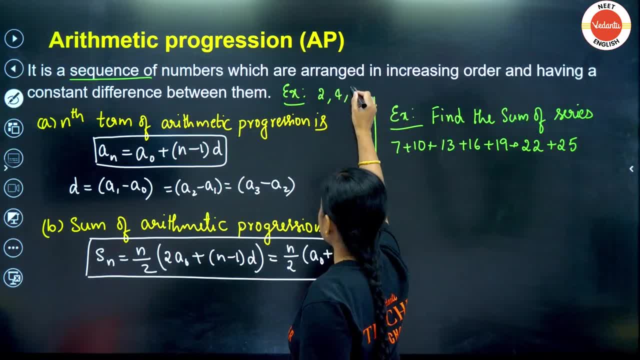 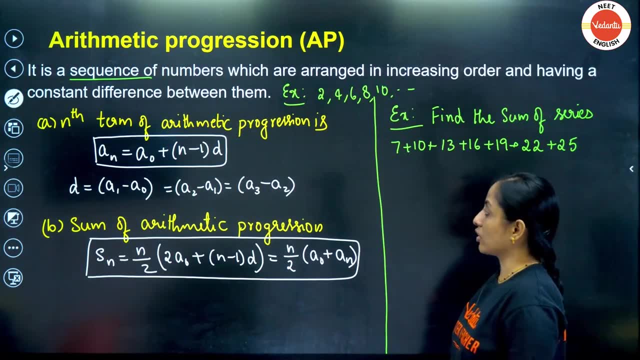 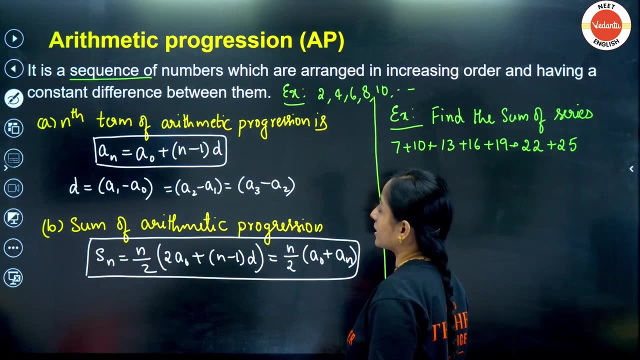 for example, if i am given numbers like 2, 4, 6, 8, 10 and so on, can i find uh ap for this? yes, because you can see that they are in increasing order. they have a sequence. are even numbers. this is a sequence and there is a constant difference. four minus two, two. 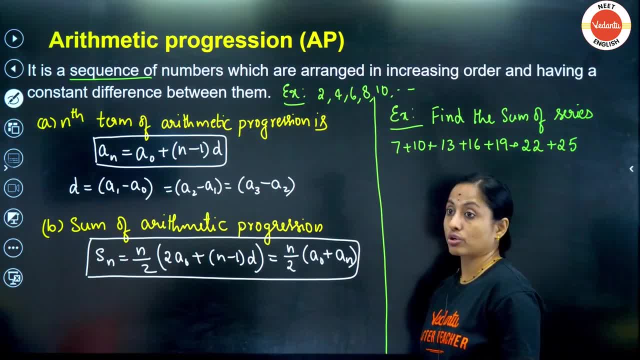 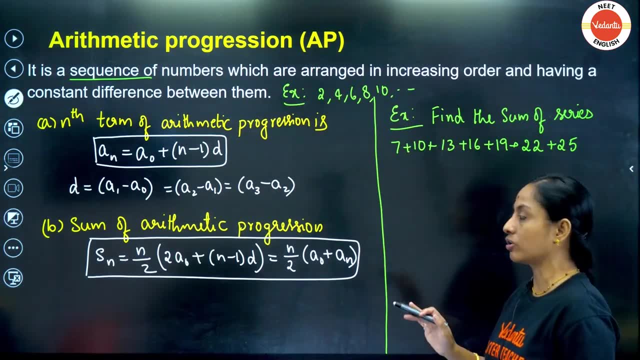 six minus four, two. eight minus six, two, so constant difference is maintained. so then i can find the arithmetic progression. so please note down the statement in your mind, or you can make down a notes of it. and what i'm going to do is this class. whatever i have made, 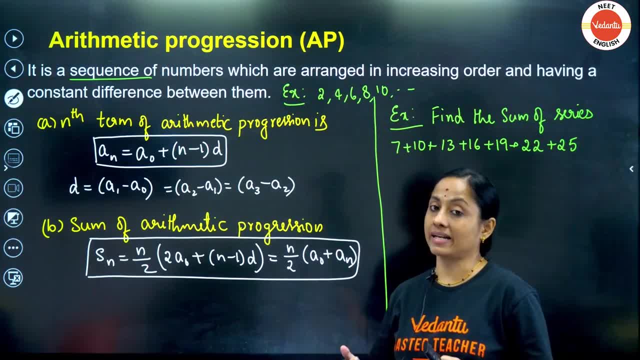 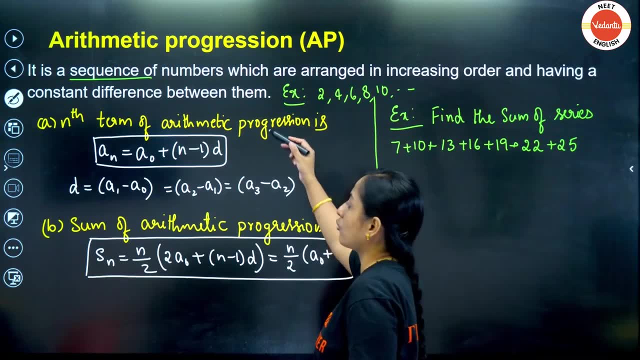 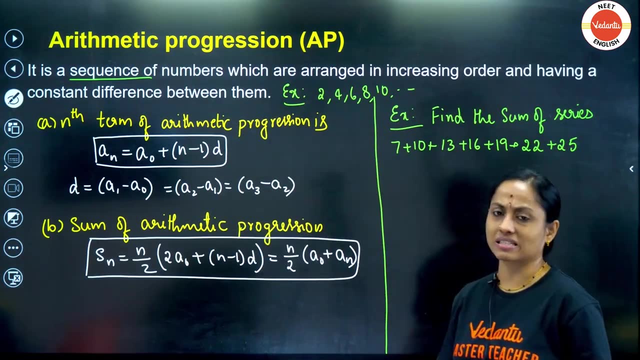 the pdf of this class will be available in neat english telegram channel. i'll make it available to all of you by clicking on the arrow Nos in trigonometry and using the mouse in trigonometry and the pdf of this nasa feminin quest 2018, so you can refer the notes from there also. okay, so. 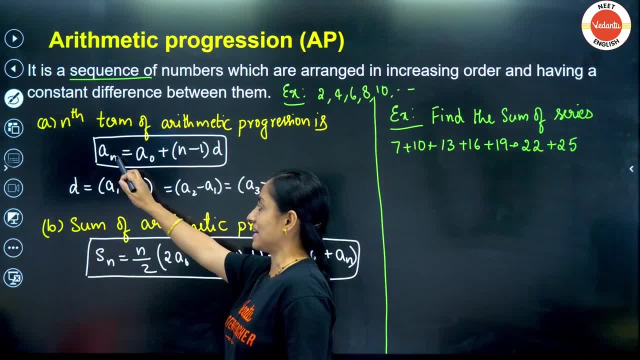 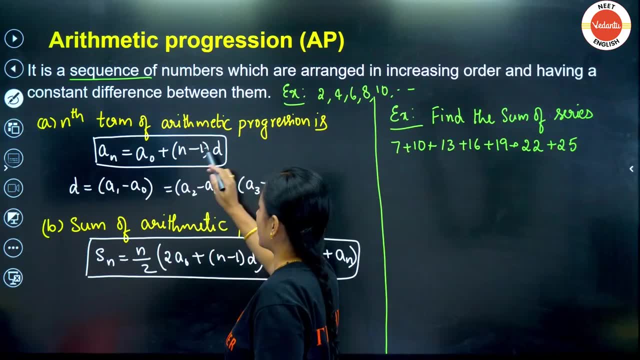 there are two formulae that you have to learn: nth term of the arithmetic progression and sum of arithmetic progression. so this is- this is how the questions are asked- to find the nth term of arithmetic progression. the formula is: a: n equals two. a knot plus n, minus 1 into d. let us 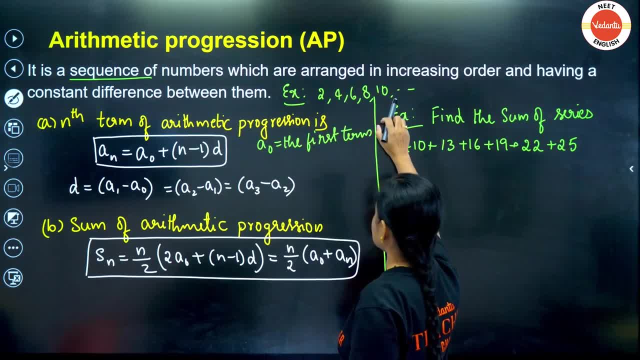 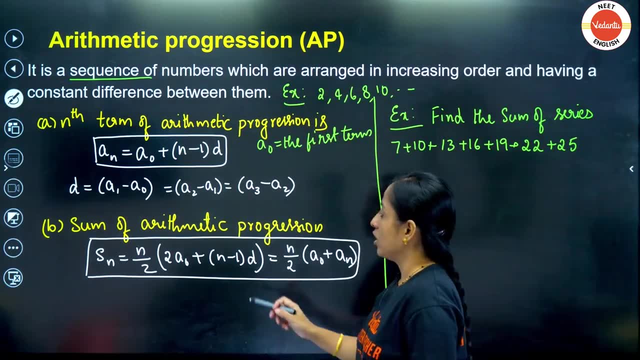 that is called a naught. So, if I consider this example, what is a naught to be considered as 2?? 2 is a naught in the given example. Next, what is n? n is number of terms. How many terms? 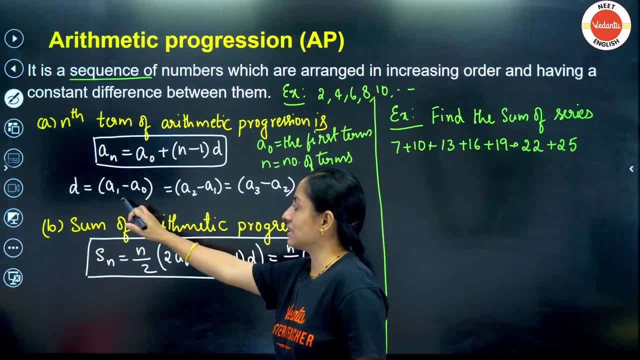 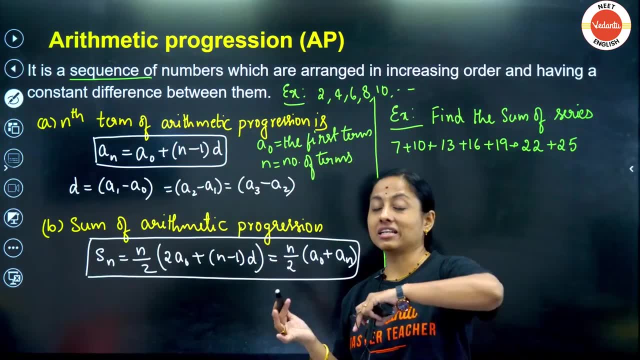 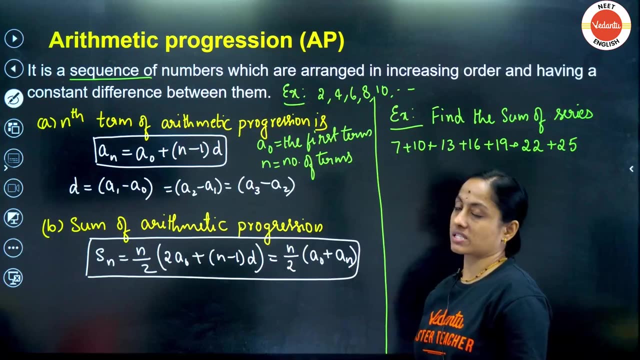 are given, That is n and d is the difference between, because here you can see that constant difference is maintained. So how to find d is Find the difference between any two successive numbers: 4 minus 2, 2.. 10 minus 8, 2.. So any two successive numbers. So in this example, 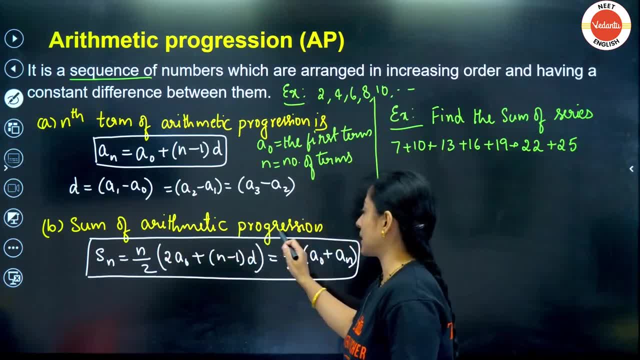 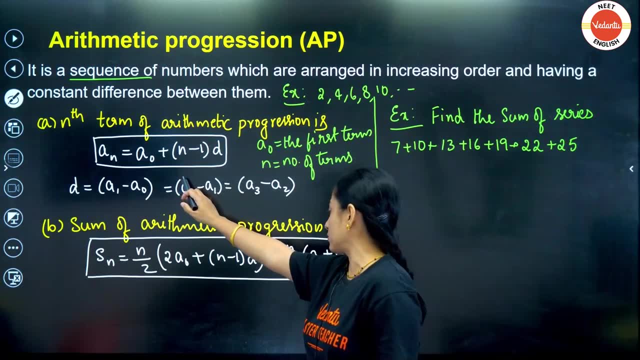 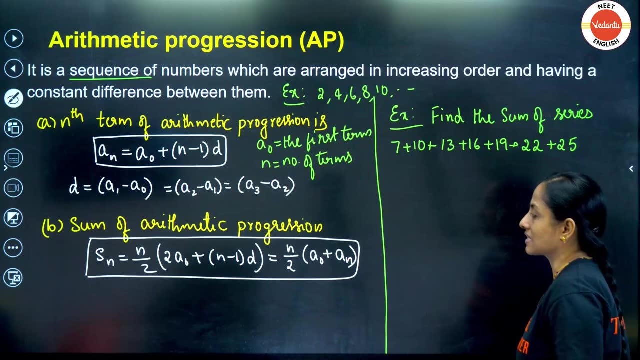 d equals to 2.. Next, sum of arithmetic progression: The formula, any formula you can remember. this is the easier formula because anyway you can find out a naught and a n by using this formula and just do n by 2, that would be easier. So just memorize these two formulae, along with. 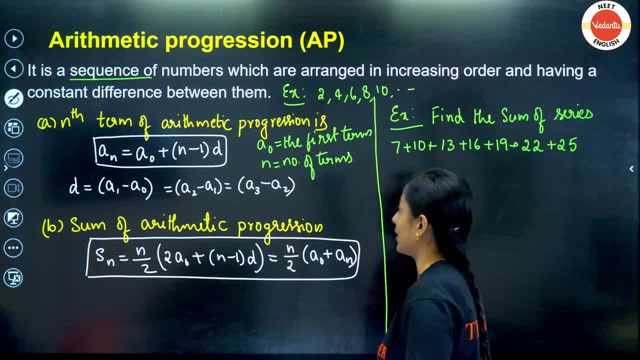 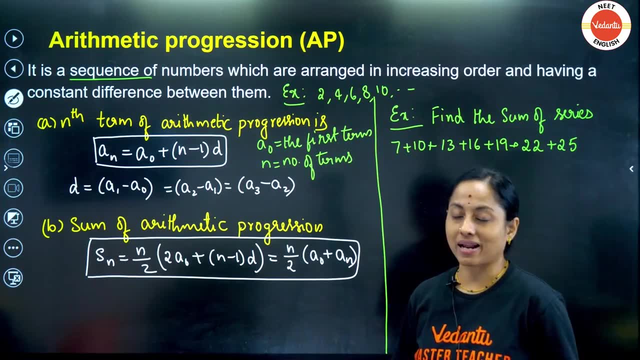 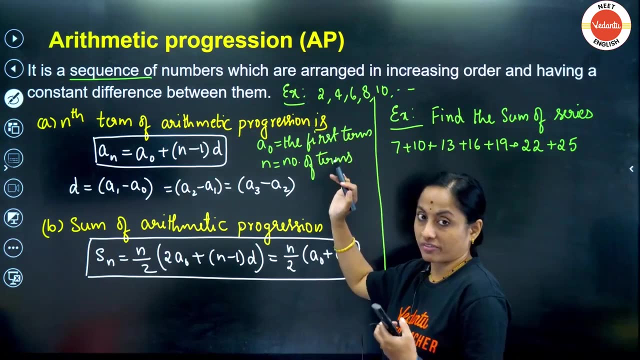 question. Question is important. formula is also Important because certain times it so happens that we remember the formula, but to which situation? which formula have to be applied? So for that purpose, please remember the heading. I mean the yellow color line, whatever I have written. that is the question and this: 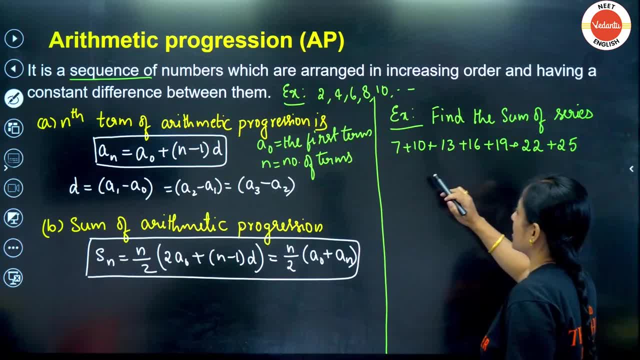 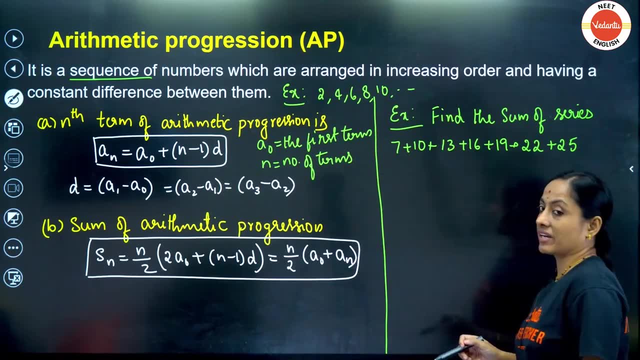 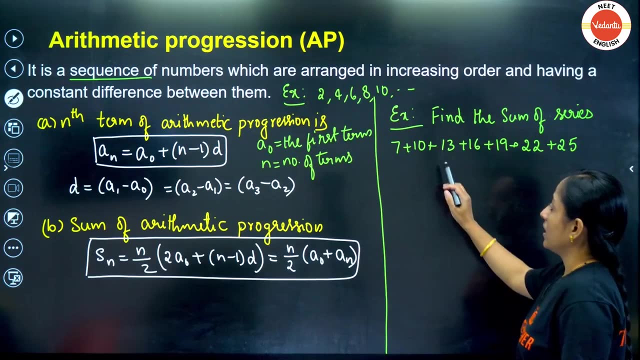 is the formula. Now let us take an example. Find the sum of the series. You are given, a series plus. you need to find out. Okay, first of all, identify the series given is obeying all the what, Whatever conditions are. See they are in increasing order: 10 minus 7, 3.. 13 minus. 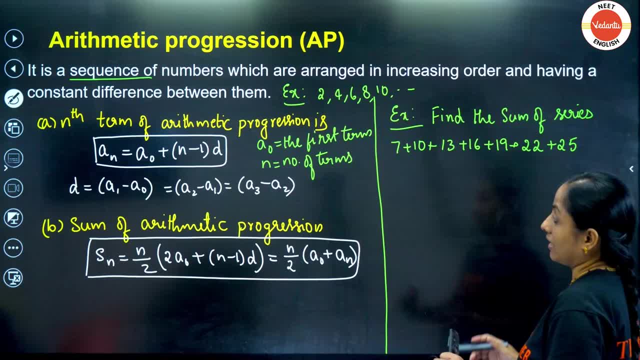 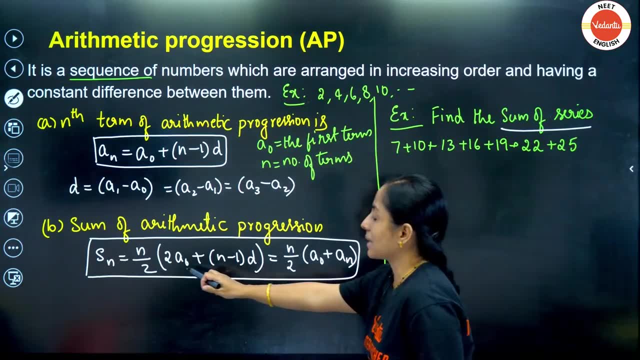 10, 3.. 16 minus 13, 3.. So there is a constant difference between the terms. So now first what we need to find. Find the sum of the series. Find the sum of the series, So which? 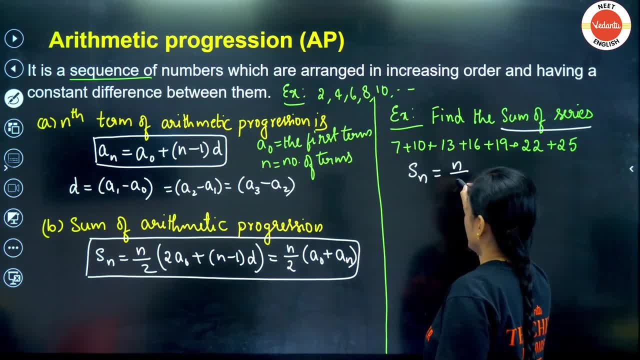 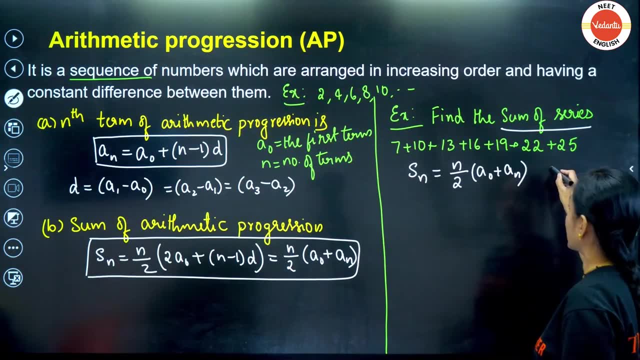 formula I have to choose. Sn equals to n by 2 into a naught plus a n. So first of all, let us identify what are the given terms. What is a naught? A naught is the first term given in the series, So 7.. Next, what is n? n is number of terms. 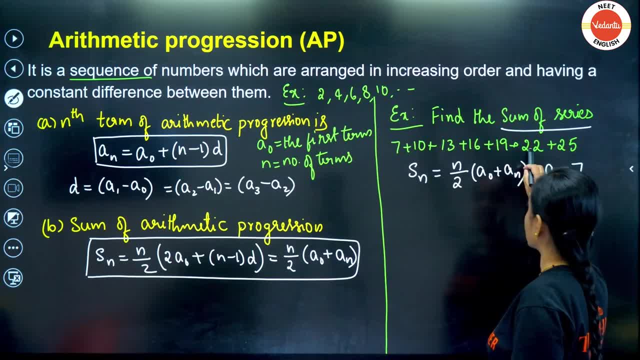 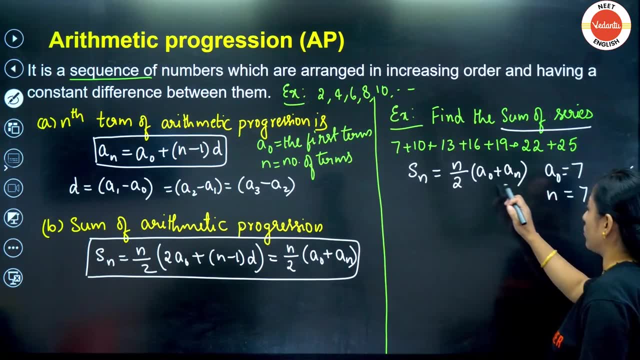 How many number of terms are there? 1,, 2,, 3,, 4,, 5,, 6,, 7.. So that also 7.. This is just a coincidence. Next, how to find a n? a naught, I know n. I know a n I have to find. So. 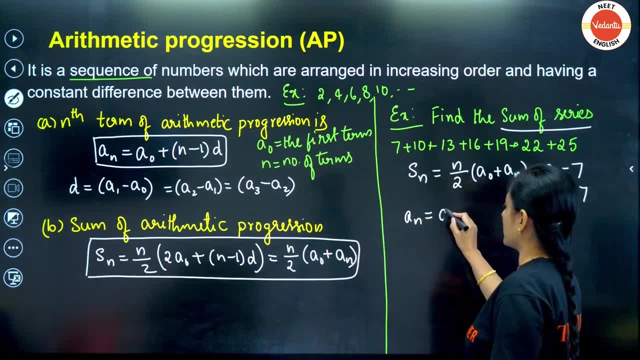 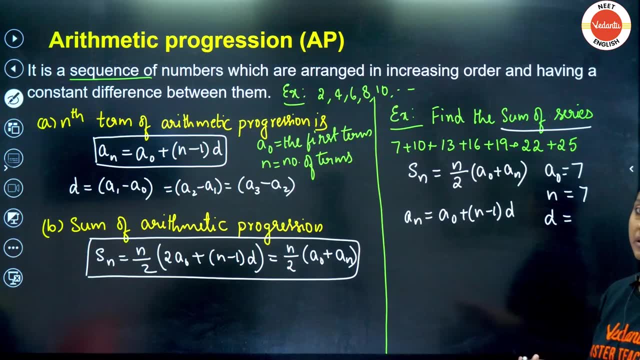 how to find a n. You can see the formula here: a n equals to a naught plus n minus 1 into d. How do you find d? d is nothing but the difference between Any two successive numbers: 13 minus 10,, 7 minus 10 minus 7.. Anything you do, you are. 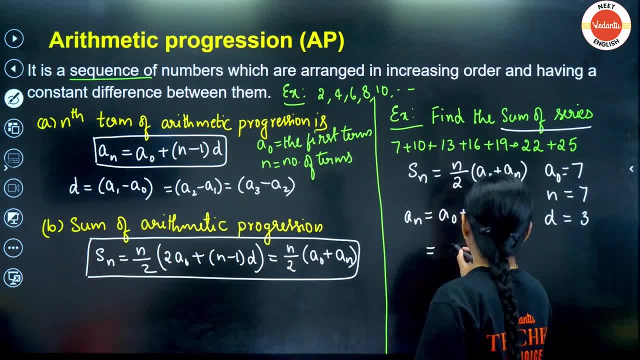 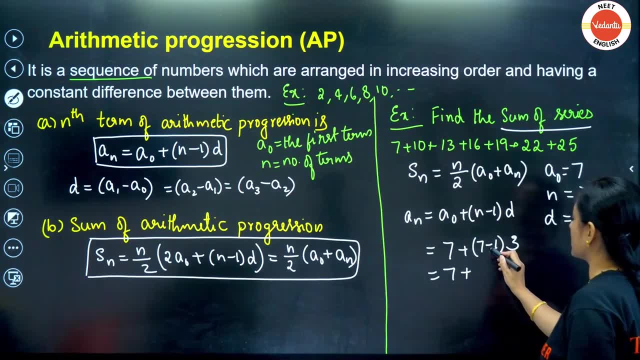 getting the answer 3.. So substitute What is a naught. a naught is 7 plus n, is 7 minus 1 into d is 3.. So 7 plus 7 minus 1, 6.. 6, threes are 18.. So the answer is 8 plus 7,. 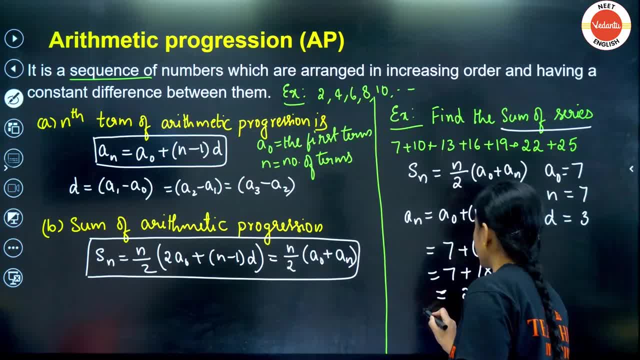 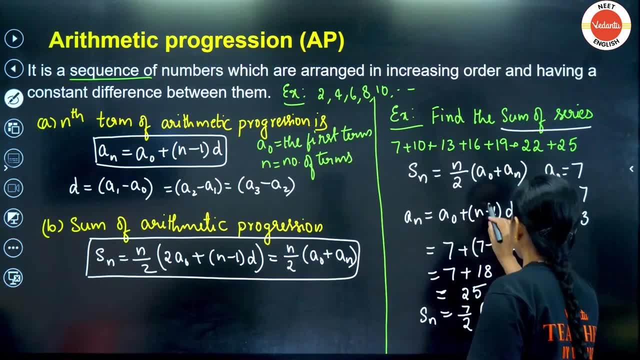 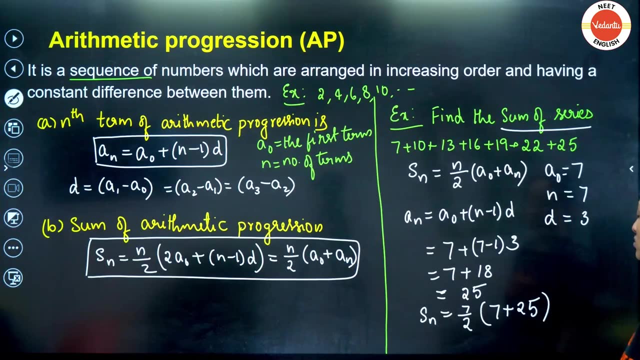 15. So it is 25.. So substitute here Sn equals to n by 2. n is 7.. So 7 by 2 into what is a naught 7 plus what is a n 25.. So can you solve this? You can. 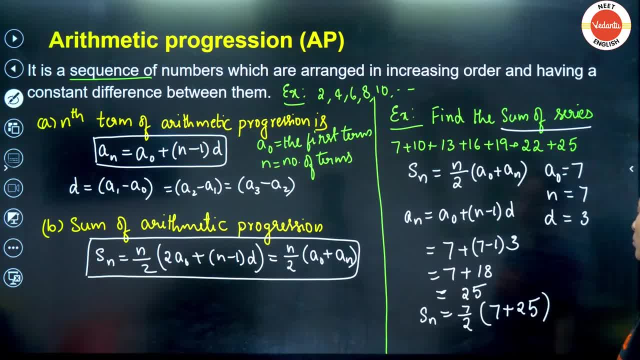 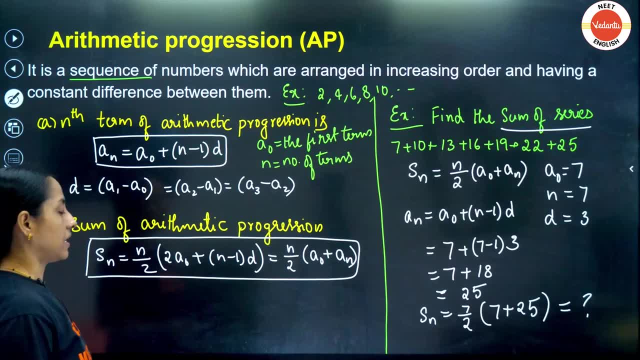 solve this, I guess. So 7 plus 5,, this is 32.. So 16 plus 7.. So this you can solve. from here You can find out what is the answer. So this is how the AP is done. Now moving: 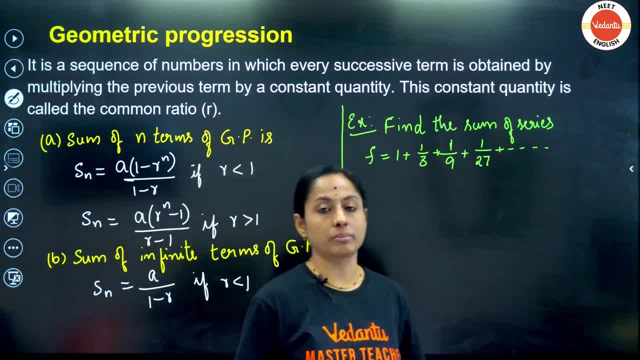 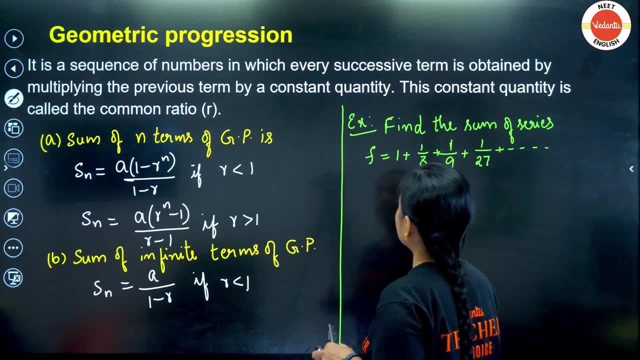 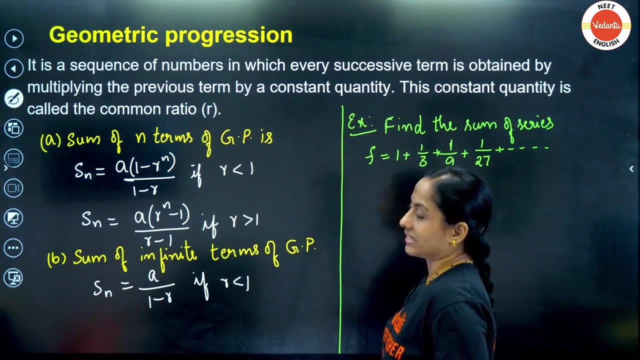 on to GP geometric progression. So when do you apply geometric progression? Read the condition. It is a sequence of numbers. Again here also sequence of numbers which Sound. Every successive term is obtained by multiplying the previous term by a constant quantity. 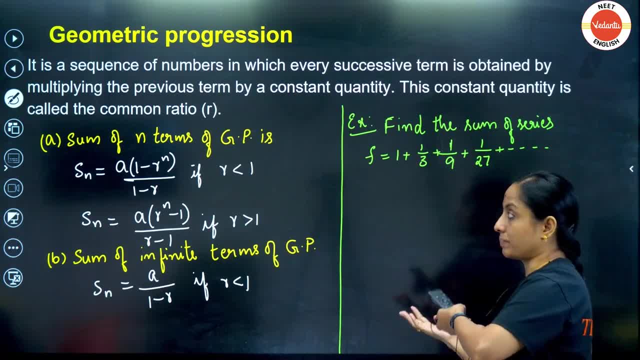 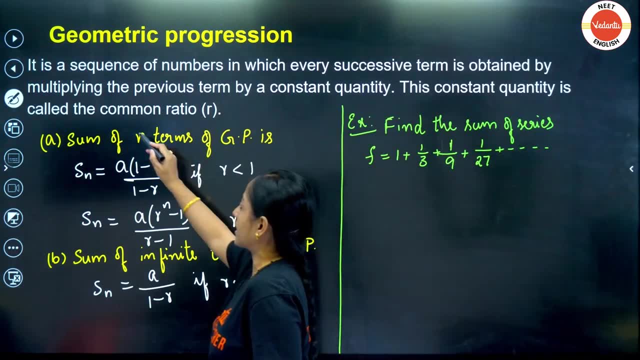 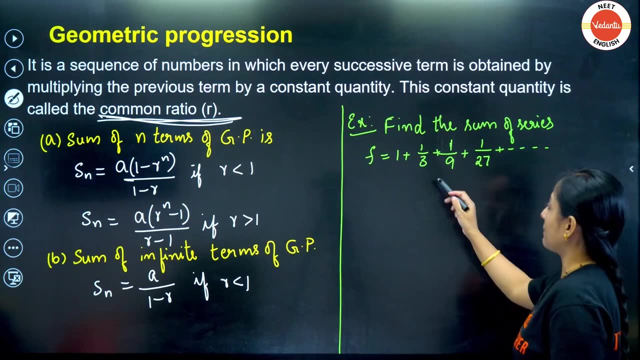 Every successive term. the next term is obtained by multiplying the previous term by a constant quantity. This constant quantity is called a common ratio R. So how do we find the common ratio R? How do we find the common ratio R Now, for example? you take this example here: If you see, this is the succesive first term minus 1592.. So now we will write this term: 1 by 1 times 5 plus n divided by 223. Then we add 3.. So what is the IVjes score? 2 in. 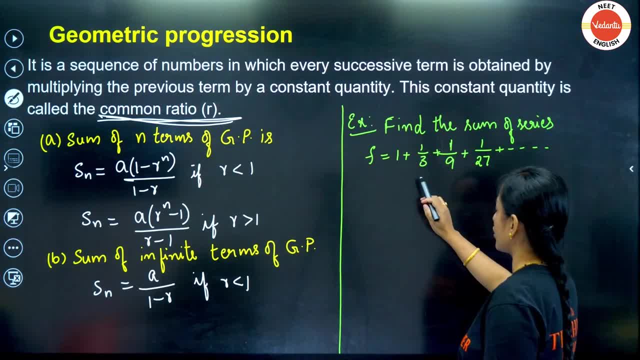 8?. Can I carry it out there with me? To a simple number, a 24, 242 r. Can I carry it out there? 1.. This is the successive number for 3.. So if I multiply 1 with 1 by 3, am I getting 1 by 3?? 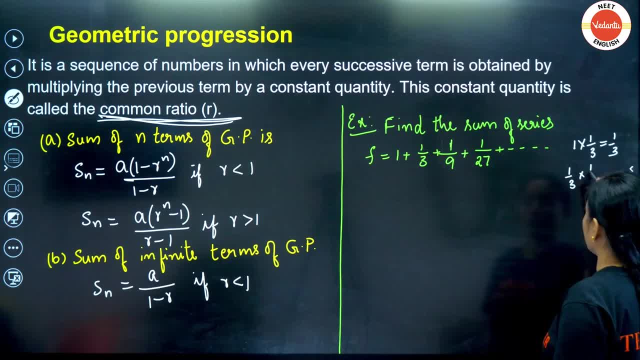 Next, if I multiply 1 by 3 into 1 by 3, am I getting 1 by 9?? If I multiply 1 by 9 with 1 by 3, am I getting 1 by 27?? So here, what is the common ratio in this given example? In this given example, 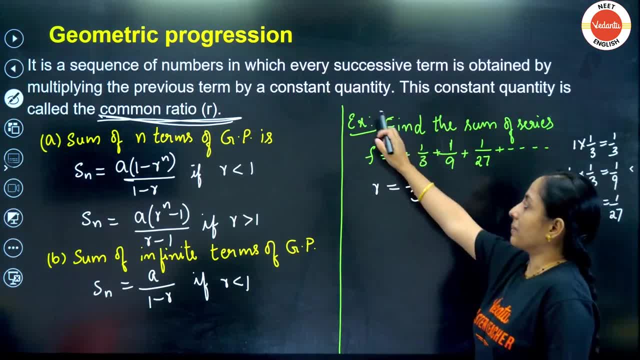 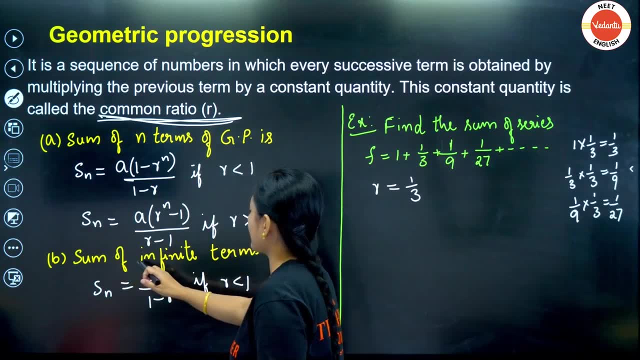 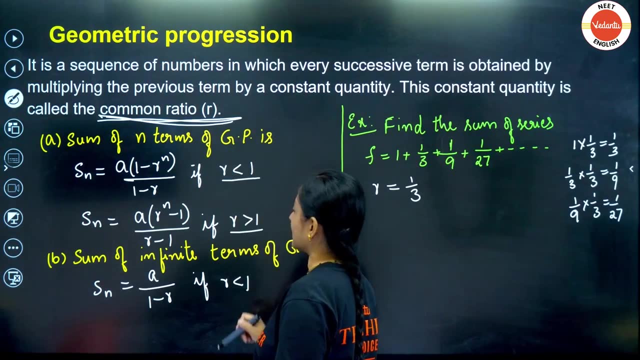 the common ratio is 1 by 3.. So that is the meaning of this sentence. So here also we have two formulae: sum of n terms of gp and sum of infinite terms of gp. So for the n terms of gp, again we have two conditions: r is less than 1, r is greater than 1 just because we will not get a. 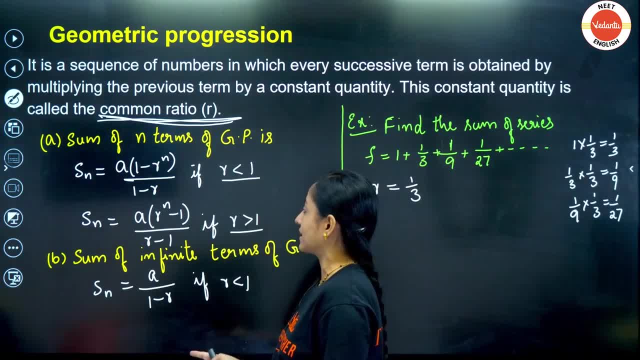 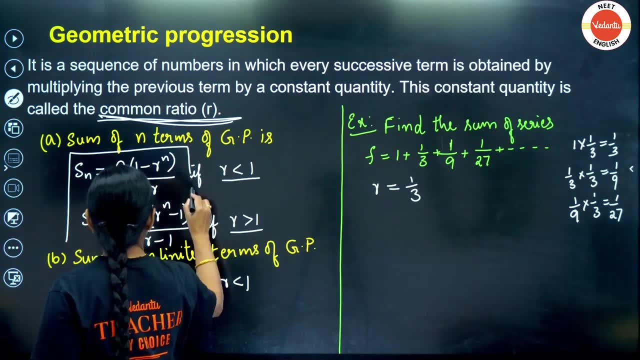 negative term. So you just have to see r is less than 1 or greater than 1 and select the formula. Okay, so this is the formula you have to memorize. Yes, you have to memorize these formulae, along with condition. Remember the question and formula. 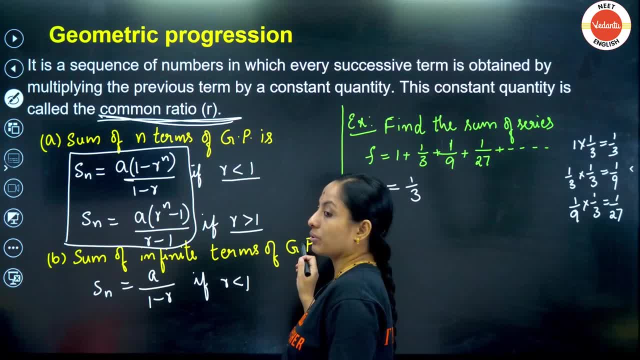 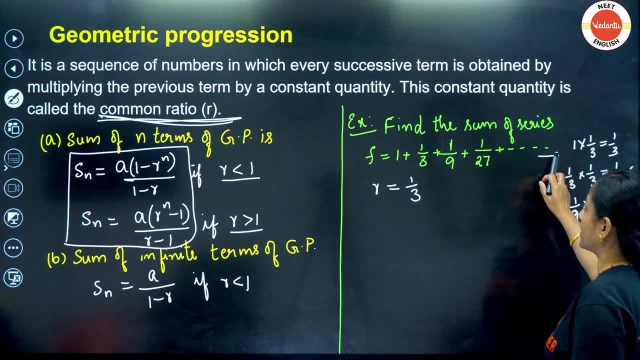 also Sum of infinite terms of gp. when you have to go for infinite terms, a by 1 minus r. Okay, so for example here, if you take the condition this is an infinite term, you can see that dots are going on. that means this is an infinite term. So how to find infinite term? What is a here? 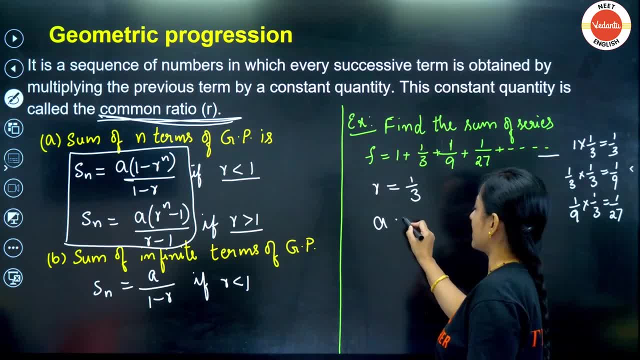 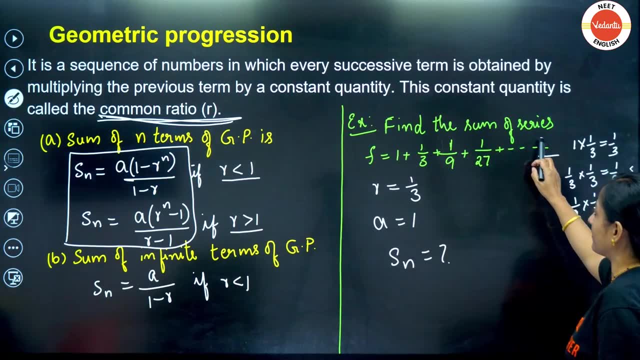 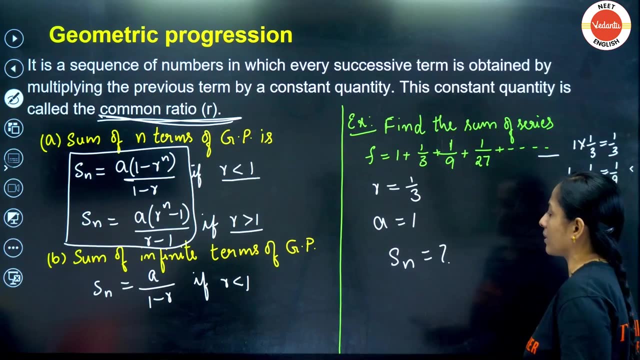 a is again the first number. So what is a here? a is 1.. So just find out Sn, Because find the sum of the series and you can see that the given series is infinite series. So we need to use this formula. So that is how you need to select. I hope you can solve the problem. 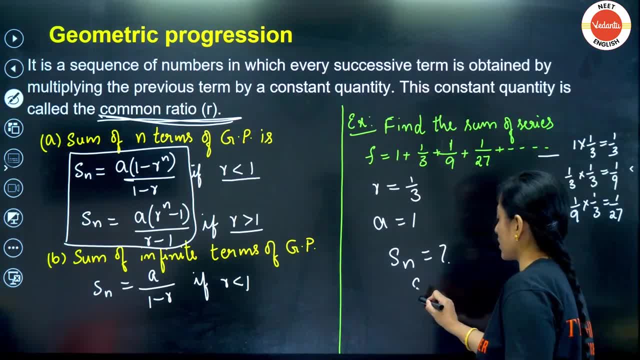 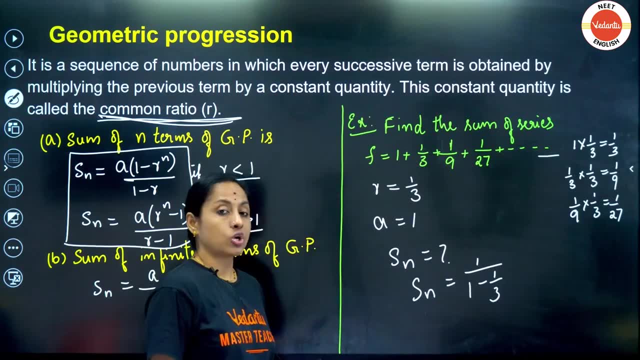 now, I guess, because 1 by 1 minus 1 by 3.. What is the answer? Sn is equal to 1 by 1 minus 1 by 3.. So solve it and find the answer. So hope ap and gp are clear for you. Now, moving on to trigonometry. 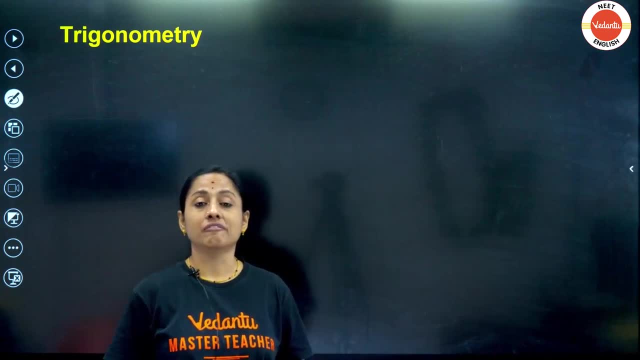 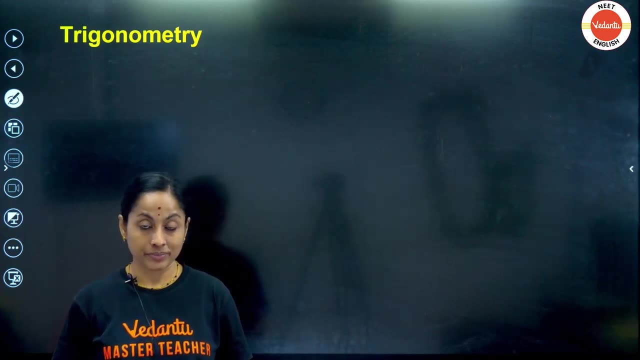 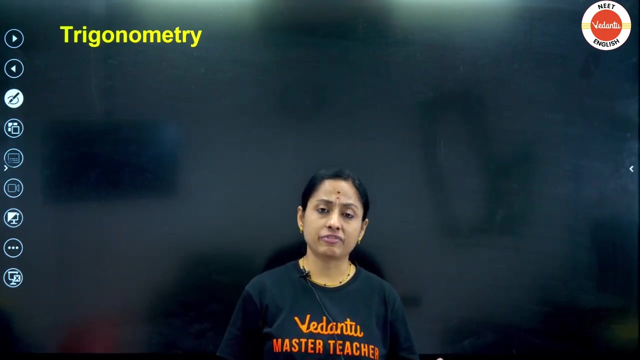 Yes, one of the most important, Very important, and from here you can see n number of formulae. See my MPC people like mathematics people. they will have trigonometry right from their 10th class. They will continue learning trigonometry in intermediate So they will be very much comfortable with the trigonometric. 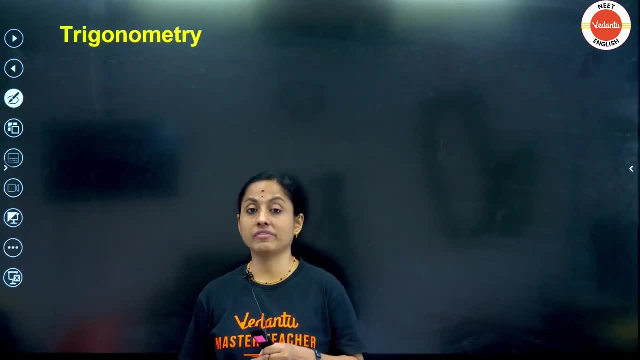 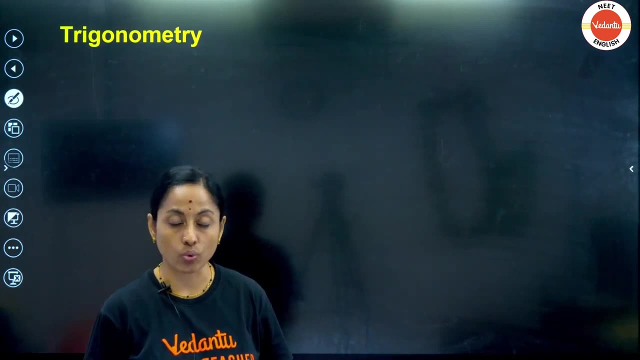 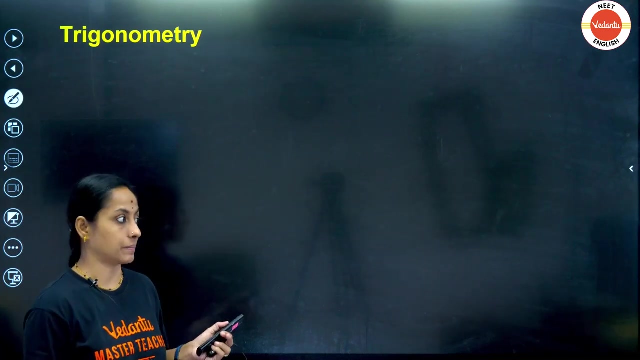 operations. But being a bio student, whatever you have learned in 10th, that is not sufficient. Intermediate, you are not going to continue with the mathematics. So here comes the bit difficulty level for the bio student. So what I recommend you is: I will be see, I will be giving. 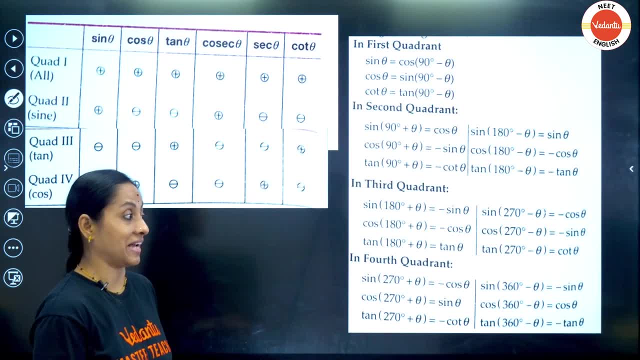 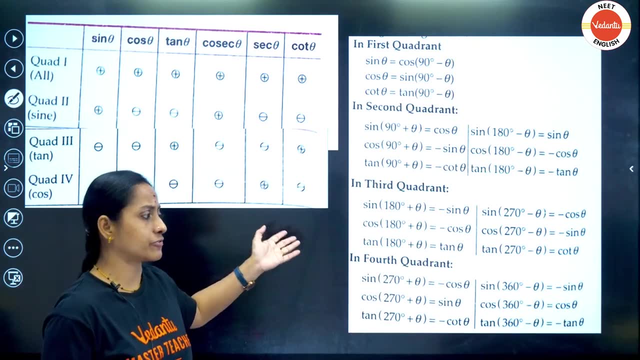 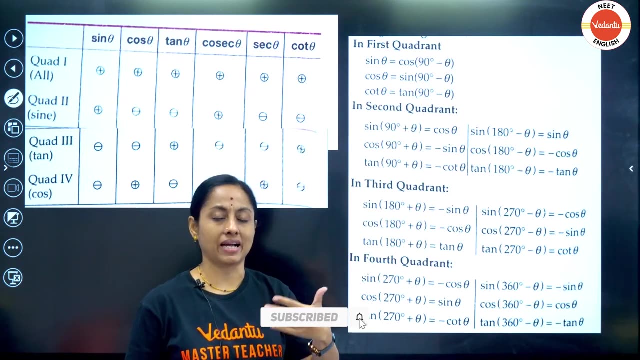 you many formulae. Don't get worried or don't get scared that, oh my god, these many formulae I have to memorize. No worries, You are going to memorize these formulae by the end of the year. So every day, just open the formulae and learn them by hand, So you will be able to learn them by hand. So. 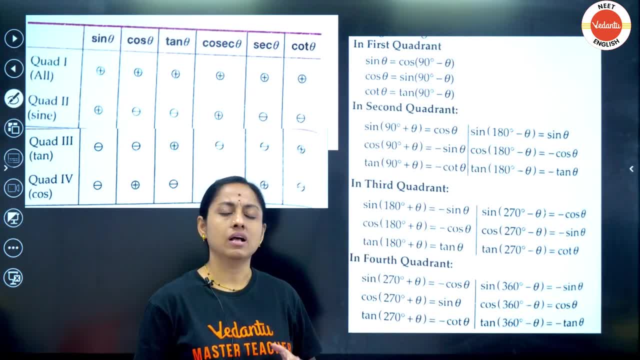 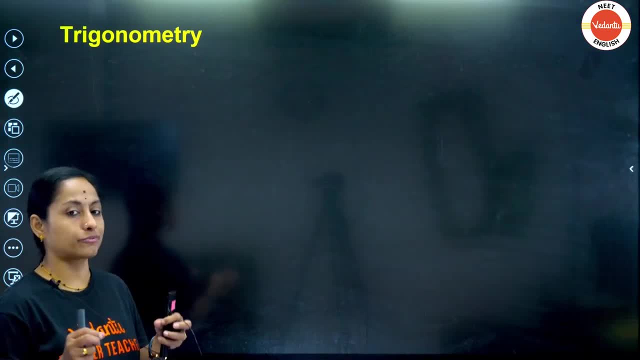 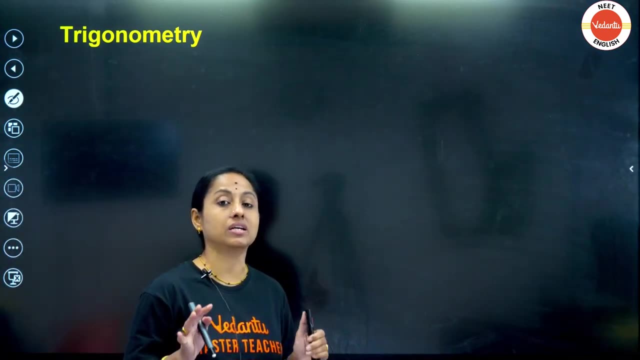 like select two, two formulae and learn them by hand. That would make your preparation very easier. But there is no alternate at all. You have to have to have to learn the formulae of trigonometry. So, starting with first of all, what is trigonometry? Trigonometry always deals with? 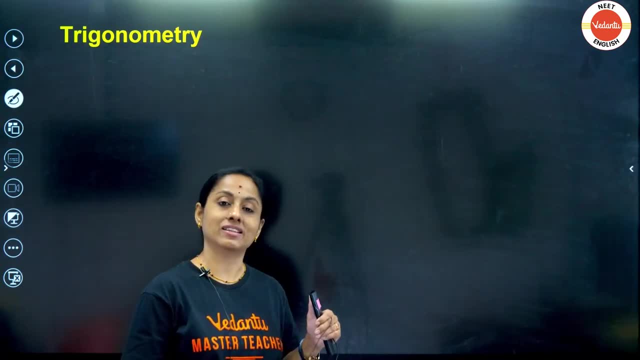 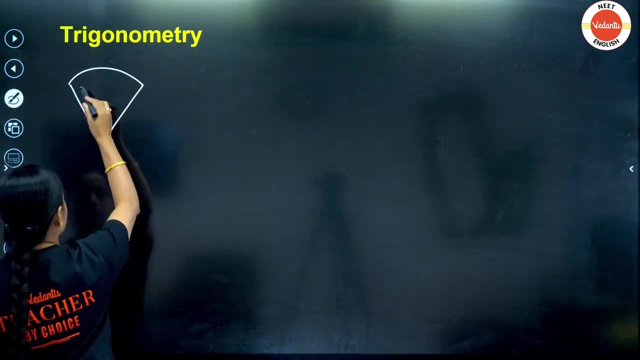 the theta. Everywhere in trigonometry you find theta. Yes, what is this theta? So here it all deals with like this: There is an arc, The arc length is L, The radius is R and the arc is making like it is a sector. The arc is making an angle, theta. 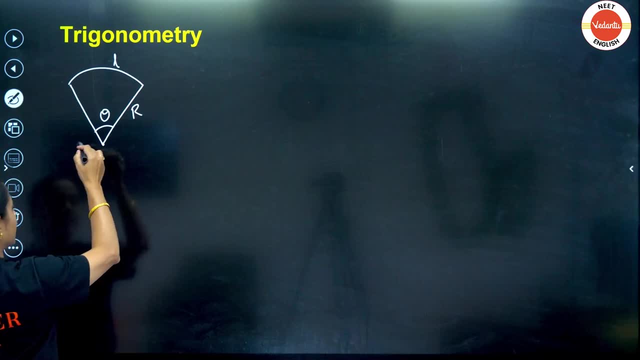 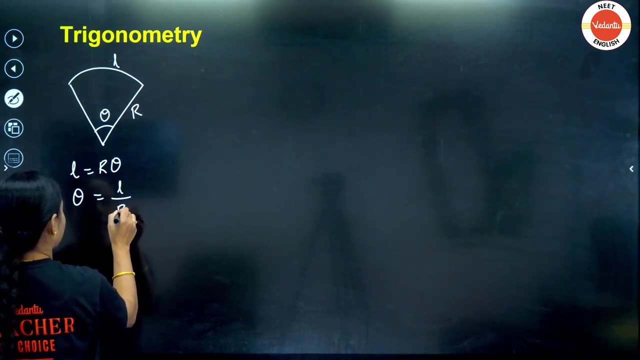 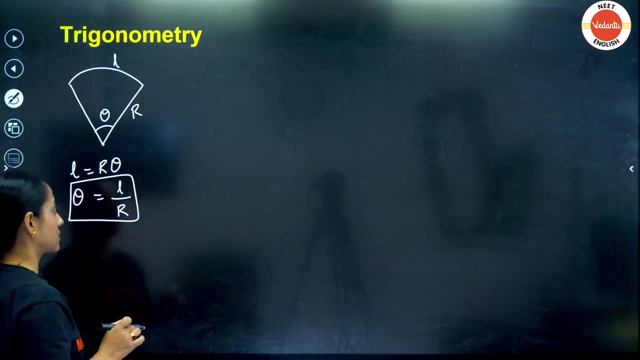 at the origin. So what is the relation between L, theta and R? is L equals to R, theta, you can write, or theta is equal to L by R. This basic information, if you know, if you understand, from here only our trigonometry starts Now, what if I take complete circle? What if I take complete circle whose? 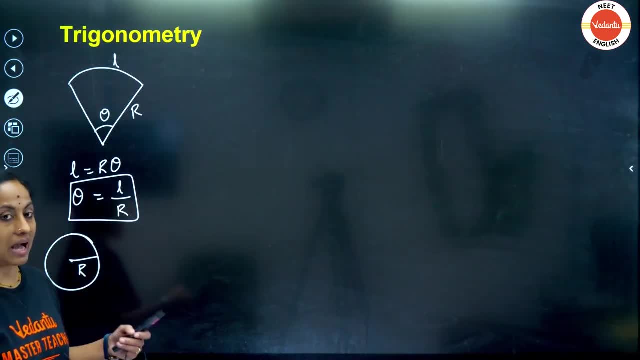 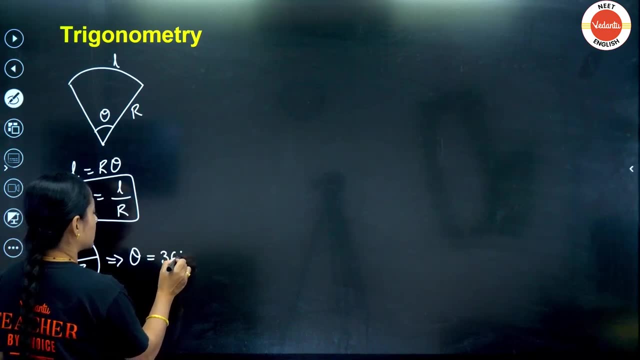 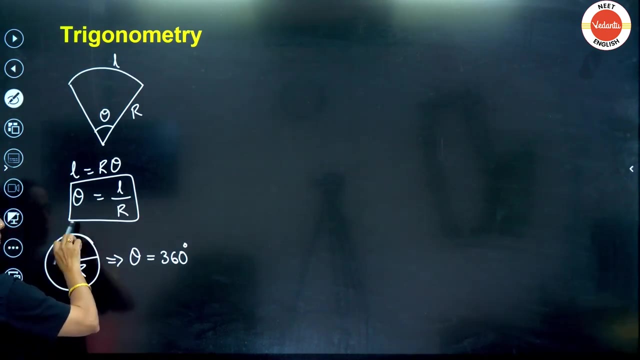 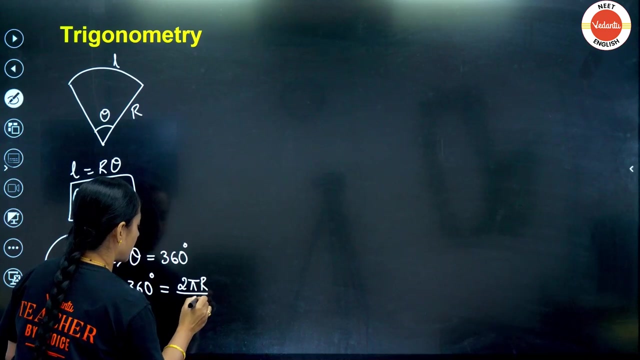 and we know that the circle makes the angle at the center is 360 degrees. here, In this case, what is the theta value? Theta value is 360 degrees. Okay, so 360 degrees. So from there, what is L here? L is nothing but 2 pi R, right? So 360 degrees is equal to 2 pi R by R. R has killed R, So 360 degrees is nothing but 2. 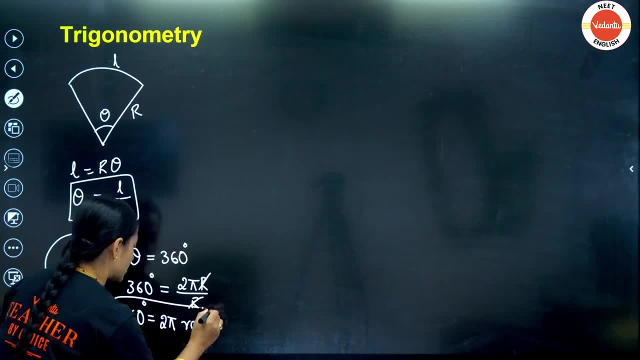 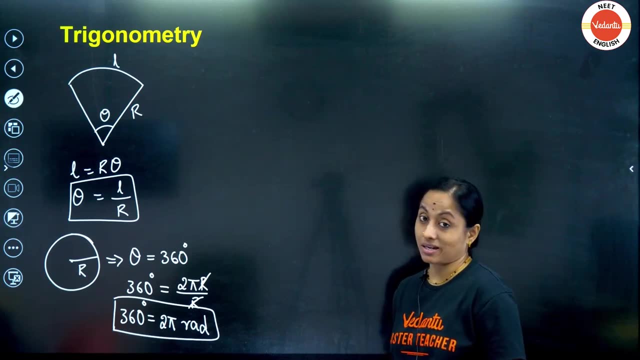 pi radians, Because theta is always measured in degrees and radians. So how to convert degrees into radians? That is the toughest part. Actually, you ask mathematics people also. Many of them have a confusion. Many of them have a confusion how to convert degrees into radians, Because they lack. 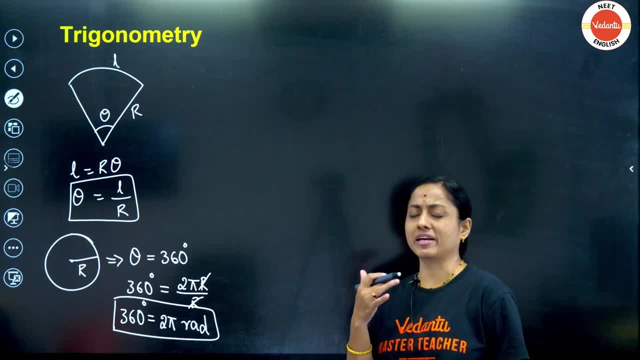 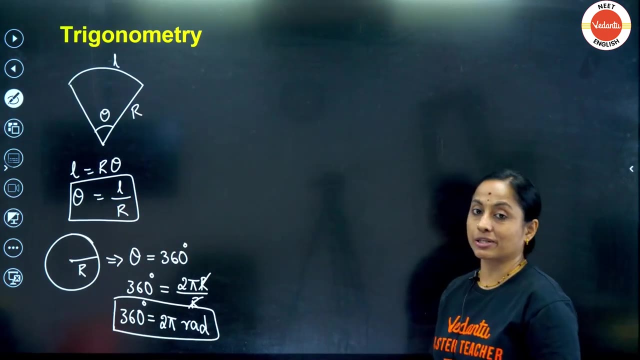 of basics, Very much basics, Lack of very much basics, And physics do need all the basics, right from zero to zero level. So please do remember all this discussion. It's very, very important. Now, you can convert easily any degrees into radians, Can you convert or not? So how can you convert degrees into? 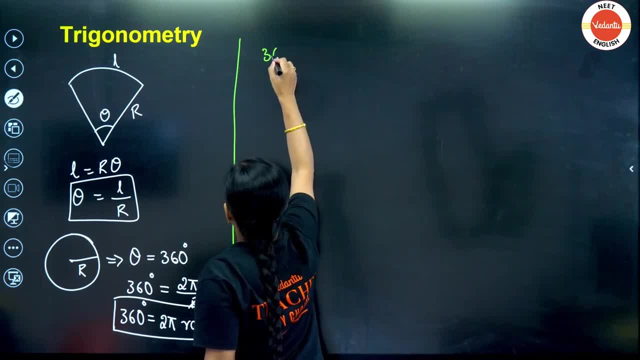 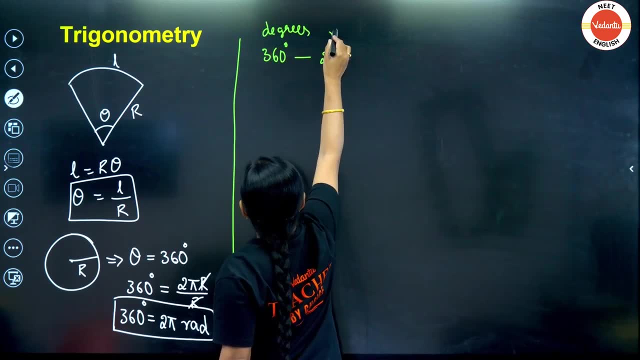 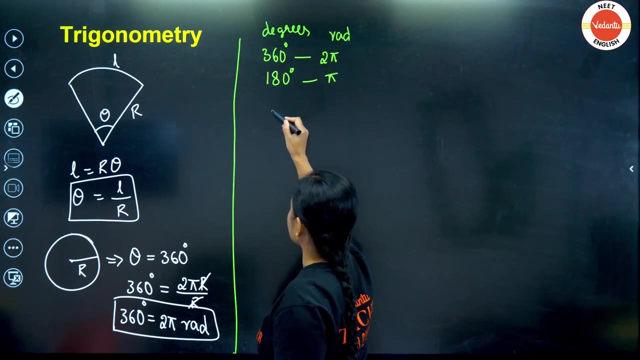 radians. Very simple: If 360 degrees equals to 2 pi radians, I'll write degrees here. If 360 degrees, this is radians. If 360 degrees equals to 2 pi radians, How much 180 degrees equals to pi radians? 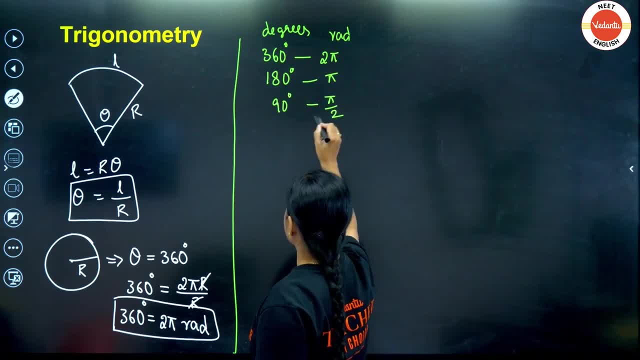 How much 90 degrees equals to pi by 2 radians? How much 45 degrees equals to pi by 4.. How much 30 degrees equals to pi by 6.. How much 60 degrees equals to pi by 3.. Anything you want, you can go on converting. 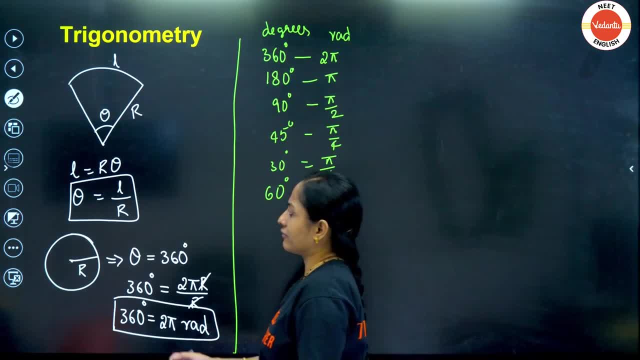 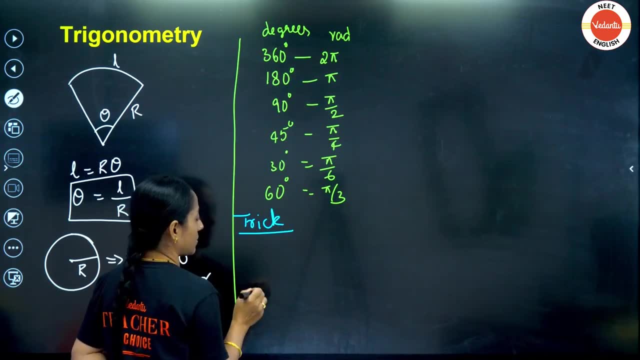 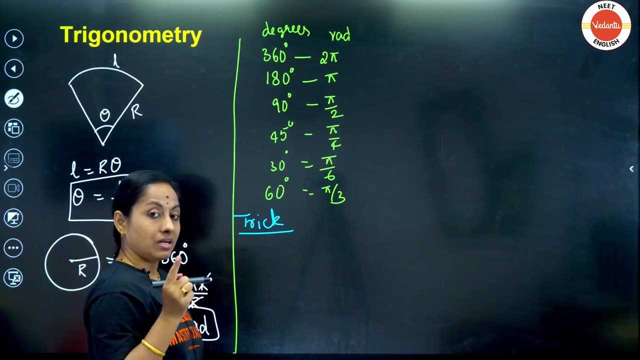 or not. It's very simple. So here I can give you a problem solving technique. also, If you want a small trick, If you want a small trick or formula, you want to remember To convert. To convert degrees into radians and to convert radians into degrees. Both we can write. So first I'll write. 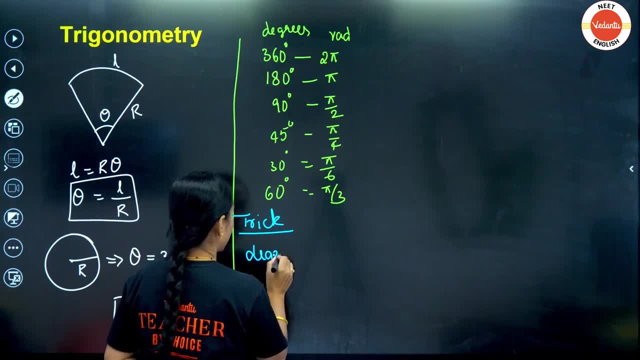 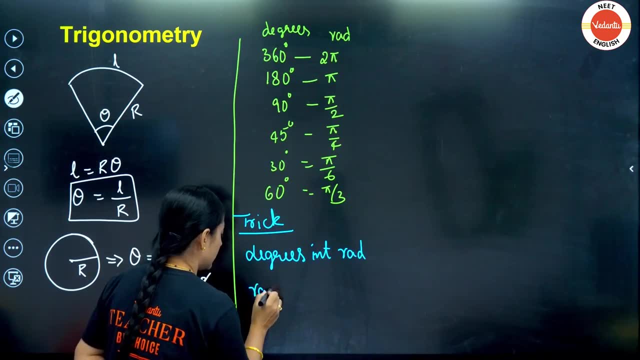 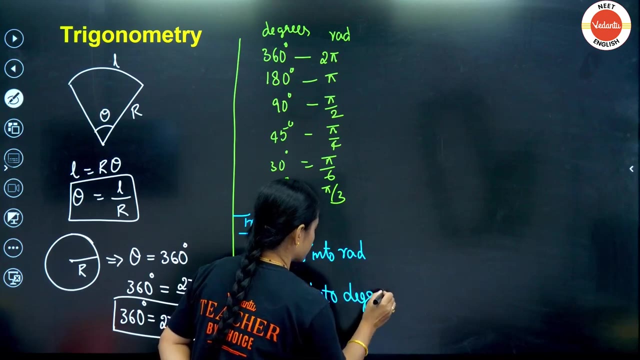 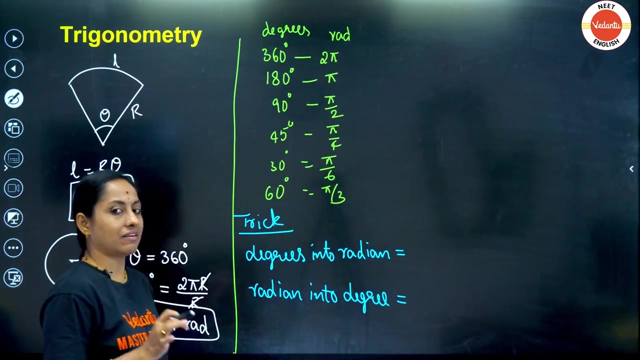 the sentence to convert degrees into radians. The next thing is to convert radian into into degrees. Okay, So radian. Let us write the full form. So how do you think I have a value, Some x value. I need to convert the x degrees into radians. 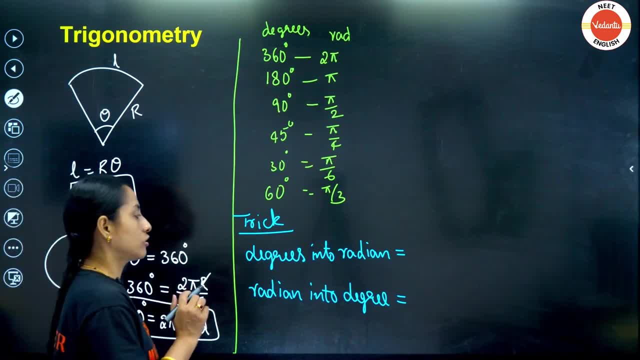 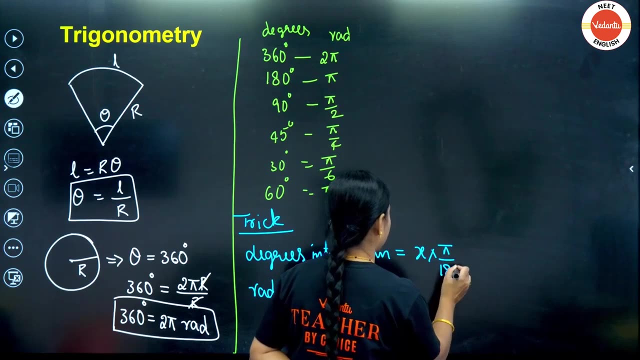 I need to convert x radians into degrees. So for example, some x degrees I have, I need to convert it into radians. So to convert into radians I need to have pi in the formula. So just multiply with pi by 180.. To convert degrees into radians, 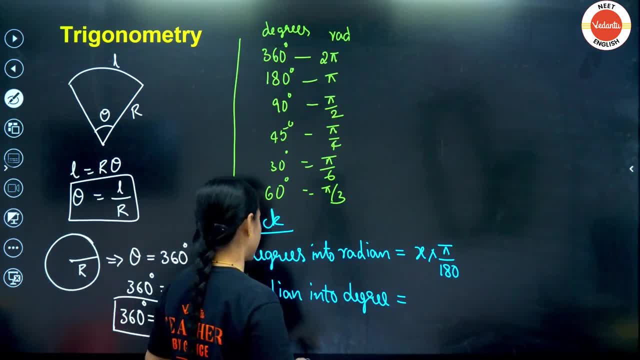 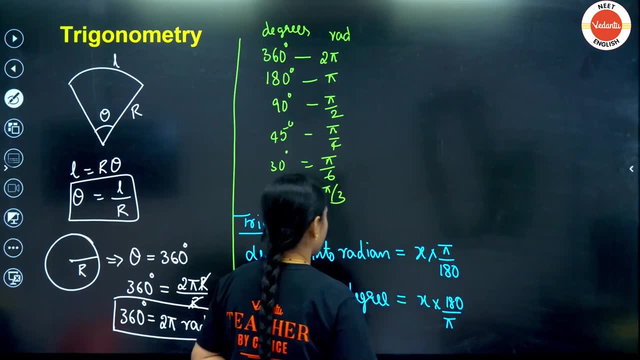 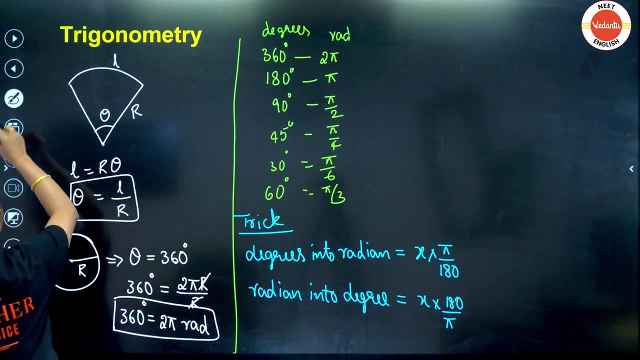 Multiply whatever value you have, Multiply with pi by 180.. Next thing is again very simple: reverse, No, So reverse is x into 180 by pi. So this trick you want, you can find out, or simply this concept, if you remember also it will be done Now. in trigonometry we use certain functions. 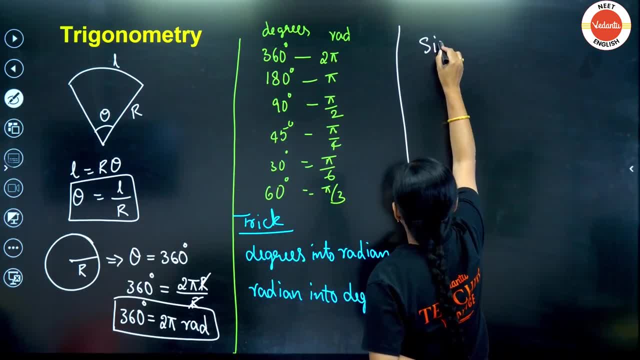 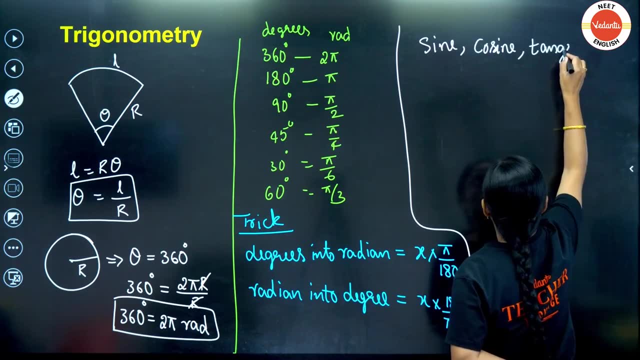 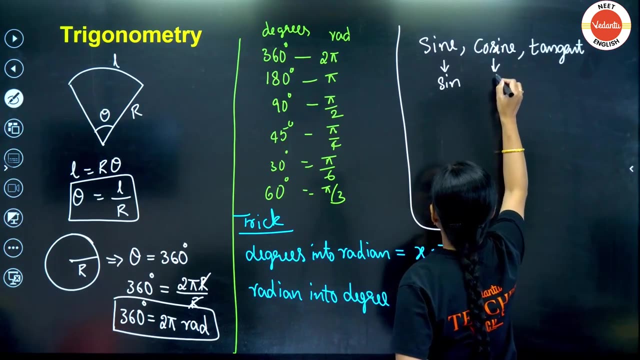 Trigonometric functions we use. What are those? Sine, Cos, Cos is also called as cosine And tangent. So these are the basic functions we will be using. Sine short form, we will write it as sine. Cosine short form, we write it as cos. Tangent short form, we will write: 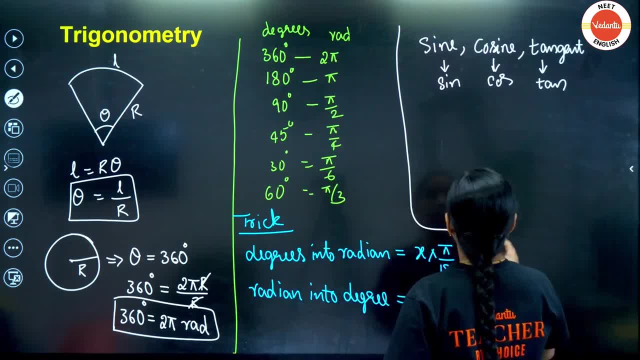 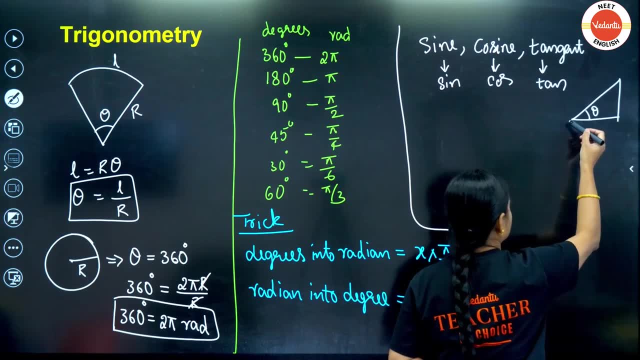 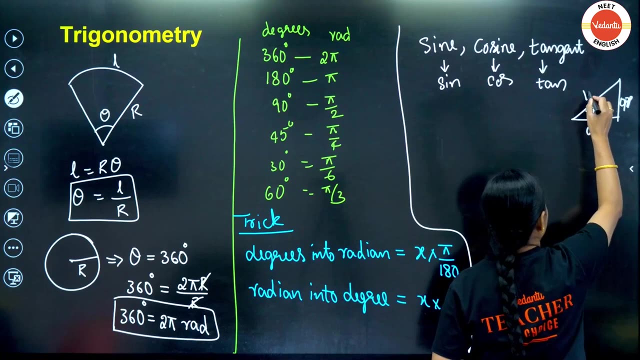 as tan. also, What are the formulae for sine cos tan? Do you remember? Sine cos tan are always applied to a right-angle triangle. So if teta is present here, then this is called hypotenuse, This is opposite side, And this is called adjacent side, And this And also. 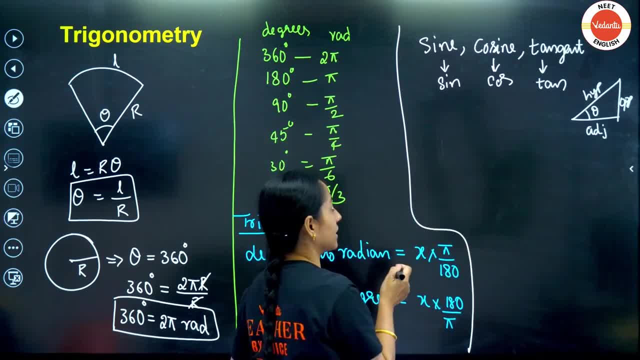 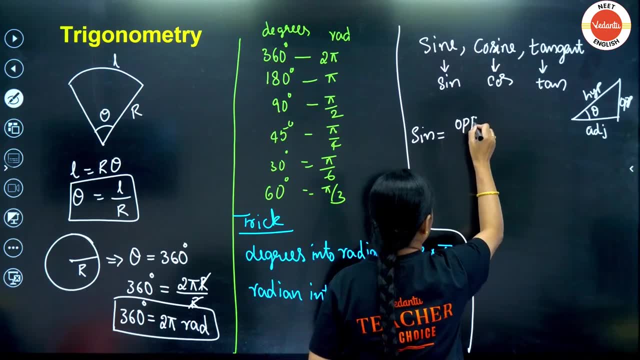 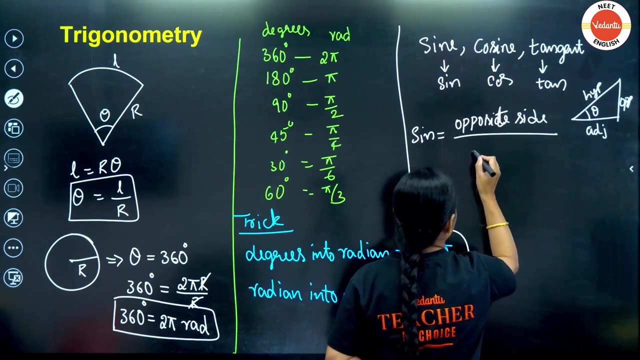 this is calledpadded sides. So, if applicable, theokes log, if and when plus or minus sponsor is the hypotenuse. So, basing on this, we can write the formula for sin cos tan. Sin is always written as opposite side by hypotenuse. Similarly, if you want to write for cos cos. 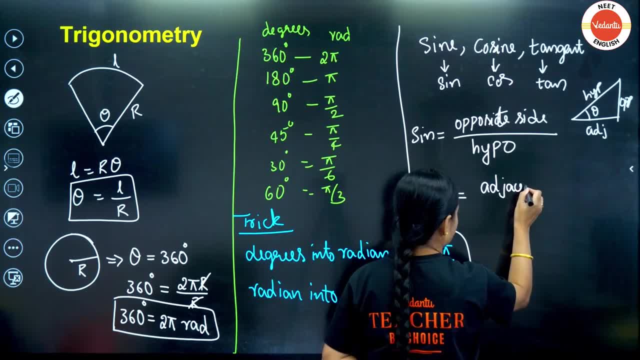 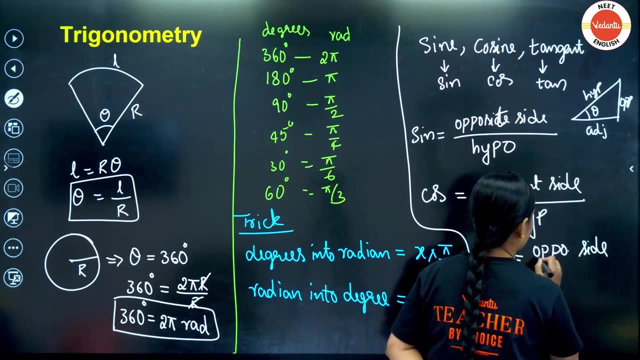 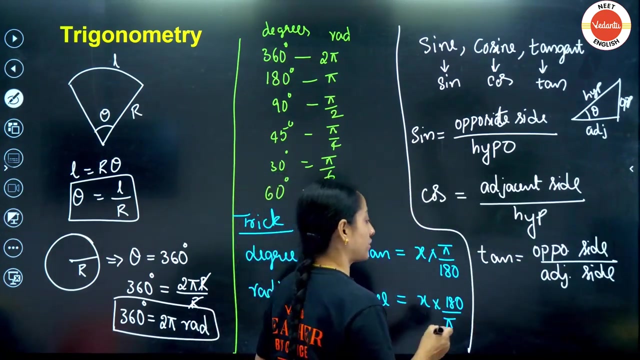 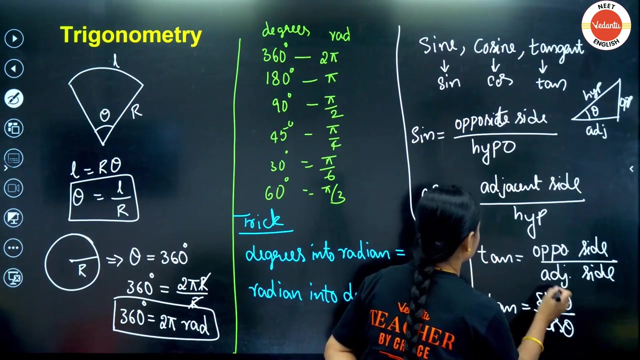 is always adjacent side by hypotenuse and tan. very simple, actually. we can write it as opposite side by adjacent side. but the easier version of tan is always: tan equals to sin by cos, Sin, cos Tan, theta by cos, theta, Theta. always I have to write theta here: Sin theta, Sin theta. 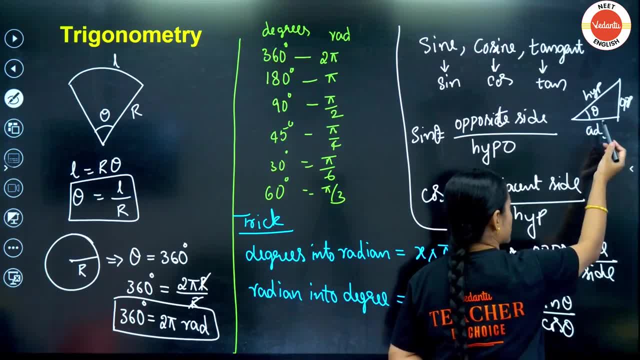 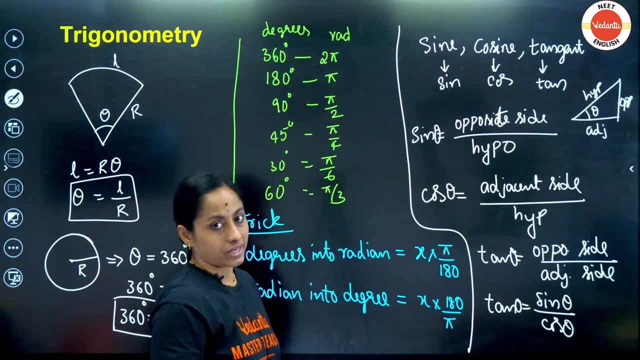 is equal to opposite side by hypotenuse Cos theta is equal to adjacent side by hypotenuse Tan theta is equal to opposite side by adjacent side. So tan theta is equal to sin theta by cos theta. This is more easier version to remember, and the other parts also, you know. 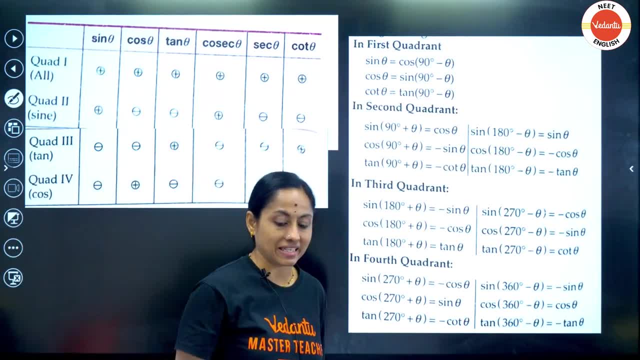 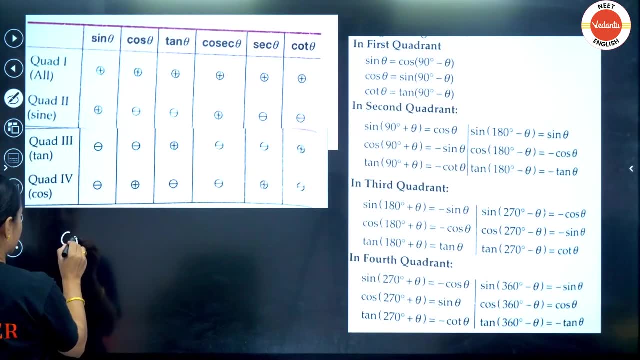 we have cosecant theta, secant theta and cot theta. These are all just reciprocals, So I can write it here: What is cosecant theta? Cosecant theta is reciprocal of sin theta. Secant theta is reciprocal of. 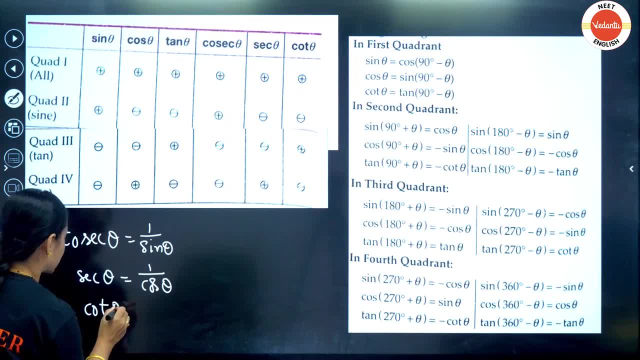 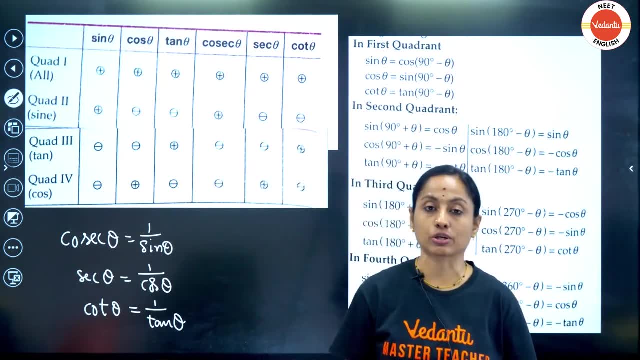 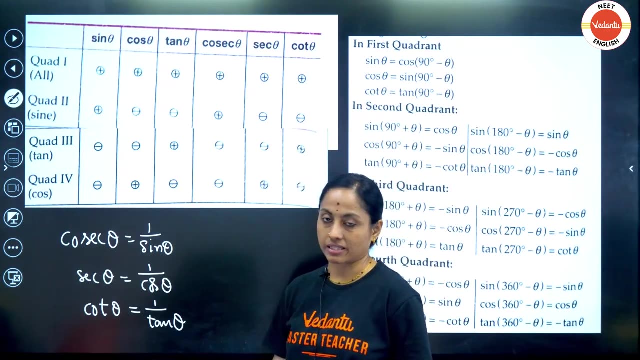 cos theta and cot theta is reciprocal of tan theta, So when you are solving problems you need not to remember separate formulae for cosecant, secant and cot. What I recommend you is remember formulae for sin theta, cos theta, tan theta. Solve the problem for them. 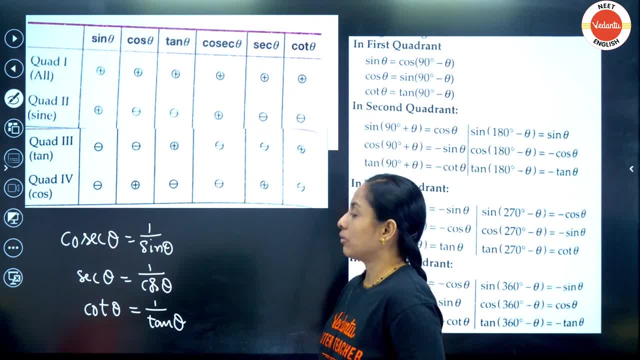 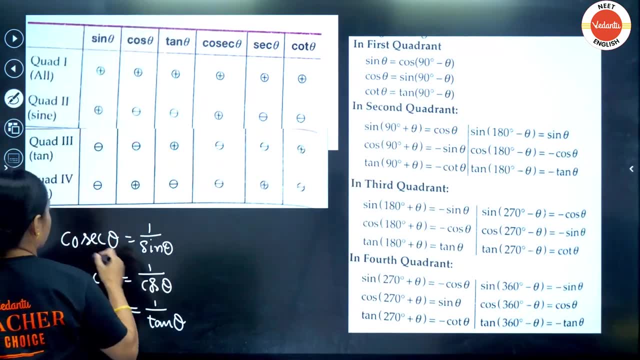 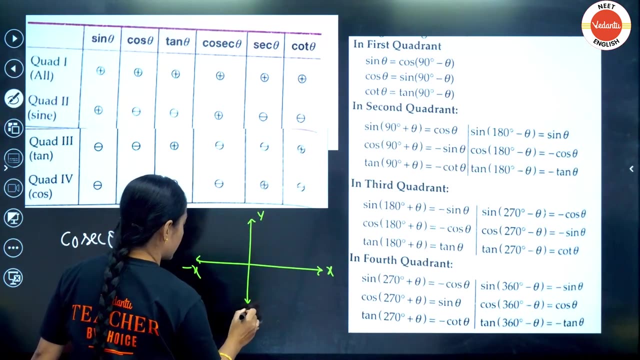 And then just do reciprocal. That would be easier version. Now in mathematics we have 4 quadrants, right, So quadrants- this part is very important because we have 4 quadrants: x axis, y axis, negative x axis, negative, y axis. This is called quadrant 1.. This is 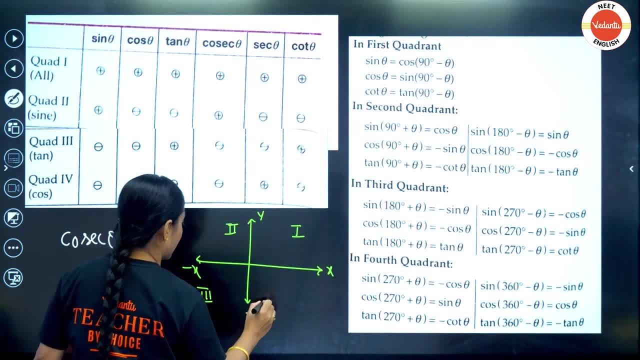 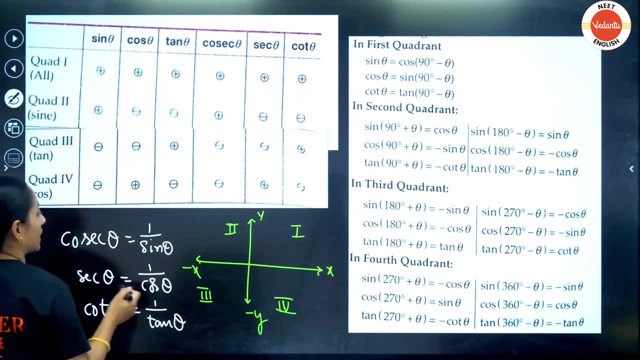 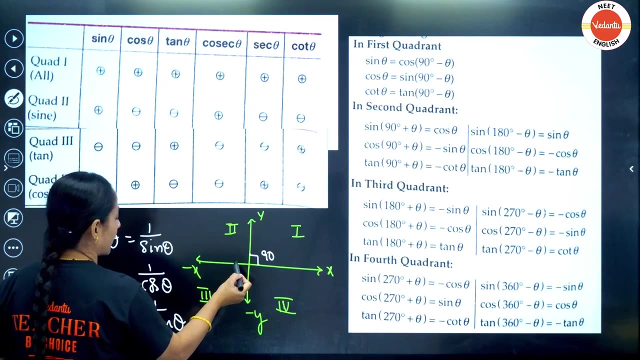 called quadrant 2 and this is called quadrant 3 and this is called quadrant 4. ok, Quadrant meaning 1. fourth, So here you can see that this is 90 degree, because the angle between x and y is 90 degree, then this is also 90 degree. So what is the total angle from x to here? The total angle: 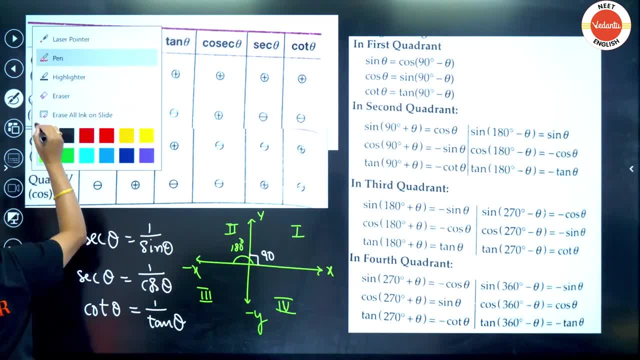 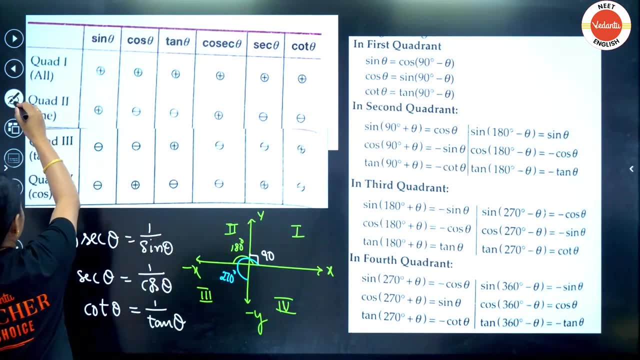 from here to here is 180 degree. Next one is the total angle from here to here: 3 ro quadrant, that is 270 degree. and the next angle is the total angle from here to here is 360 degrees. I hope you understood this here. He's sheet and haft as well, So I hope you understand. 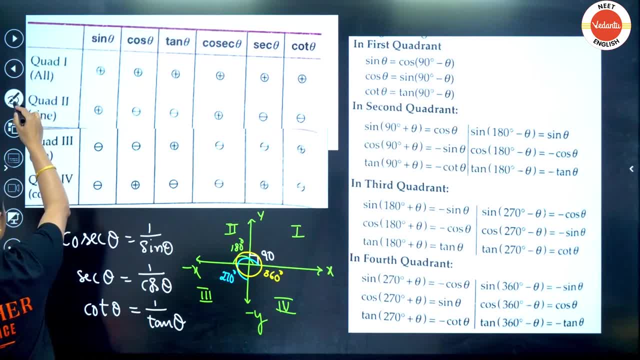 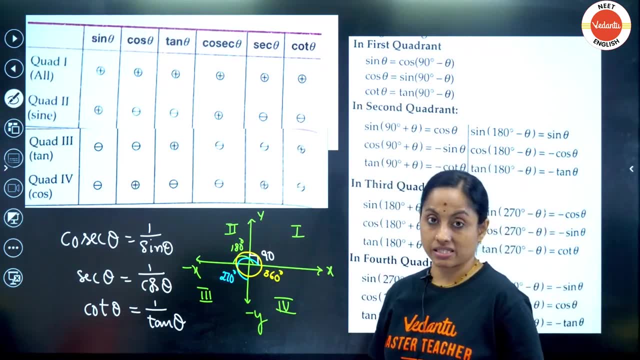 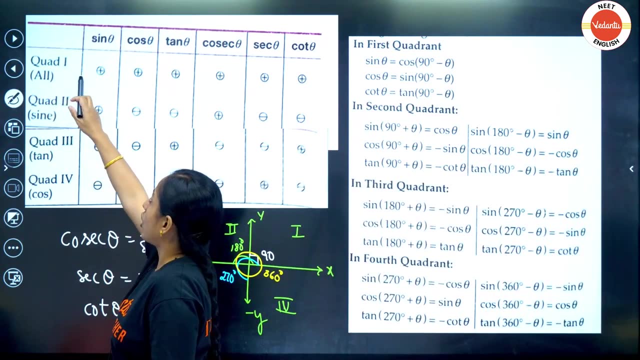 this you know okay. so now there is a problem actually in problems physics, how do we get, is find the value of sin 90 plus theta, cos 90 plus theta, cos 90 minus theta. and here comes the problem of plus and minus. you can see here in quadrant 1, all sin, cos tan, cosecant, secant, cot, all are positive. 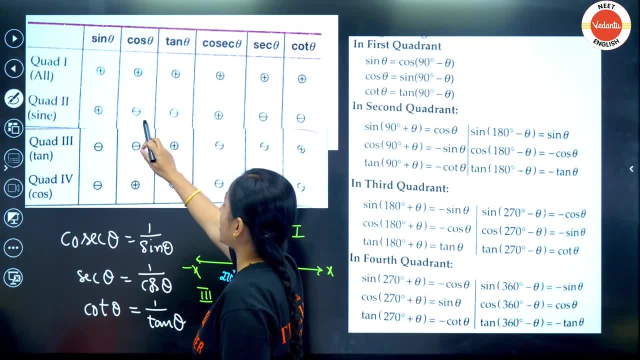 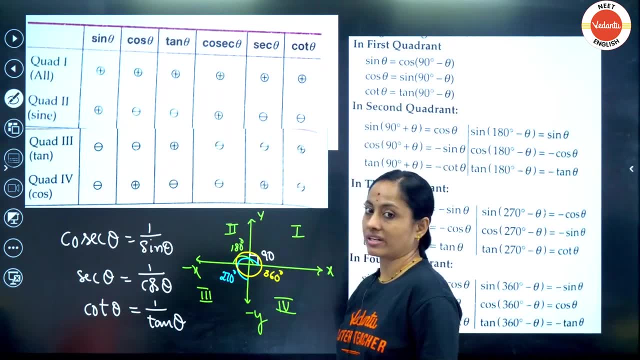 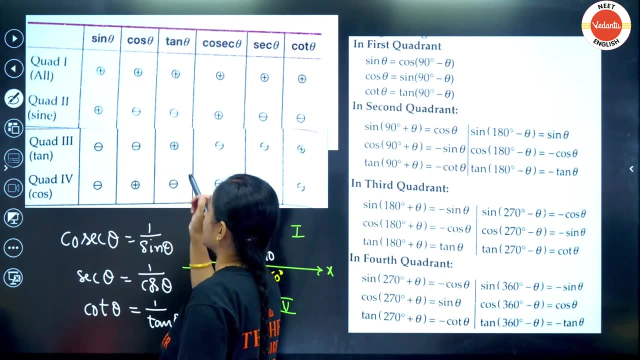 quadrant 2: sin positive, cos and tan are negative. when sin is positive, cosecant is positive. when these two are negative, the other two are also negative. so what i tell you is no need to remember for cosecant, secant cot, only remember for sin, cos, tan, and for this there is a shortcut also. 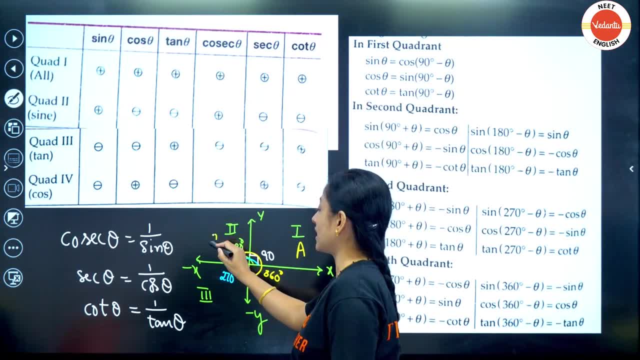 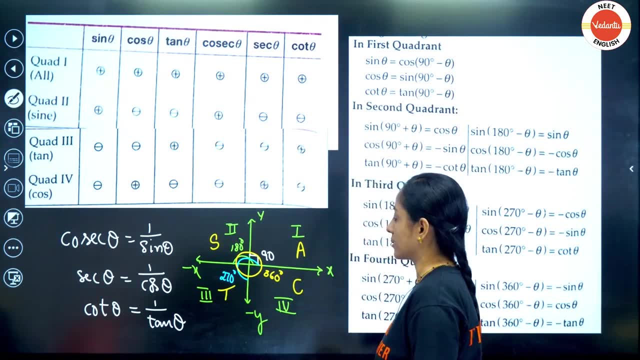 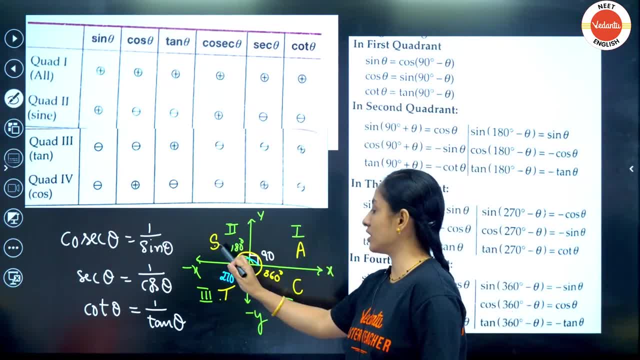 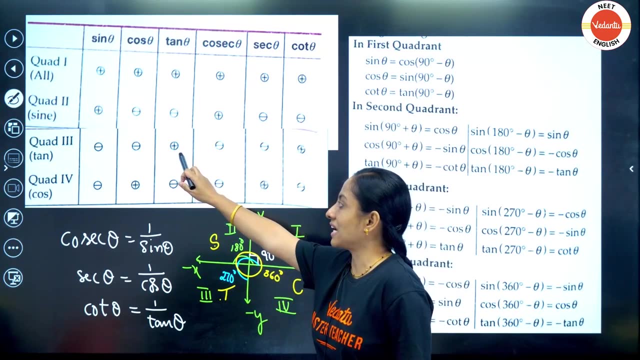 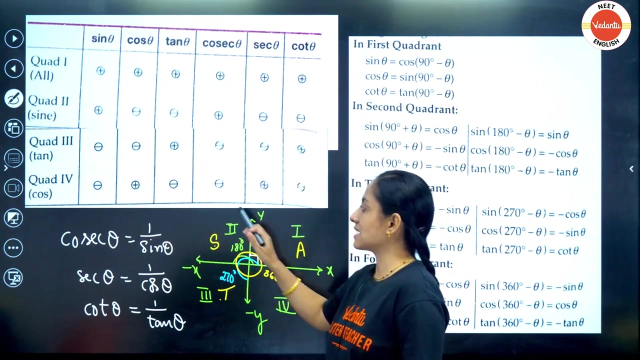 add sugar to coffee. add sugar to coffee or all silver tea cups. all are positive in first quadrant. second quadrant: only sign is positive, others are negative. third quadrant: only tan is positive, others are negative. fourth quadrant: only cause is positive, others are negative. 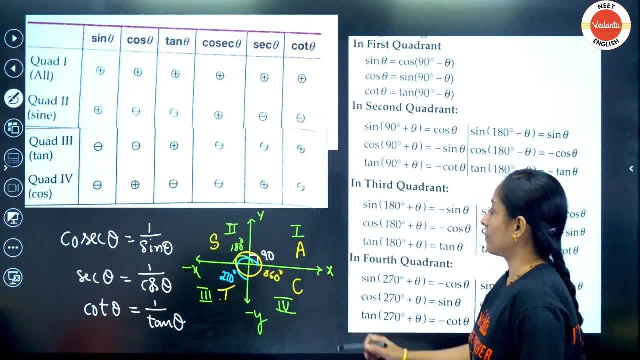 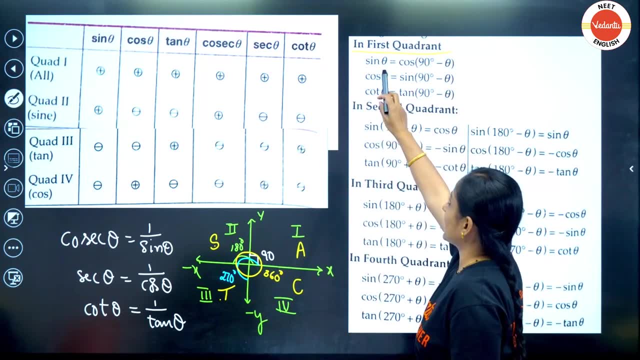 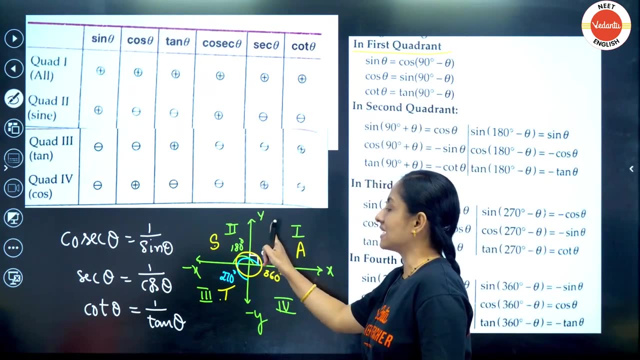 I am telling reverse, I guess. so I hope you got the point. so, basing on this, only here the formulae are written. let us see in first quadrant, first quadrant, sin theta. let us come like this: cos 90 minus theta, 90 minus theta, 90 minus theta comes into first quadrant. remember, 90 plus theta comes. 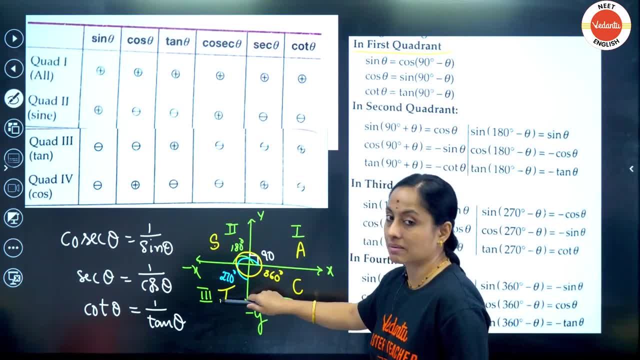 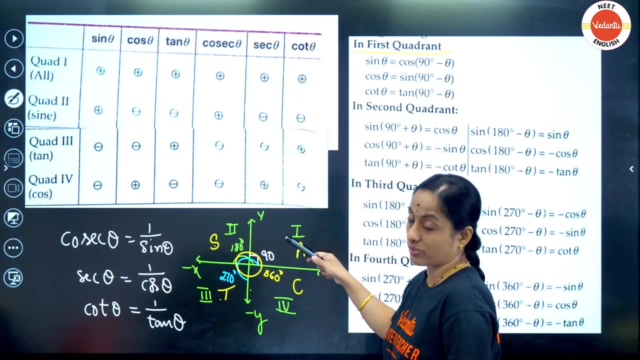 into second quadrant. 180 plus theta comes into third quadrant. 180 minus theta comes into second. next, 270 plus theta comes into fourth. 270 minus theta comes into third. 360 plus theta comes into first quadrant. 360 minus theta comes into fourth quadrant. so this basic knowledge, if you have, 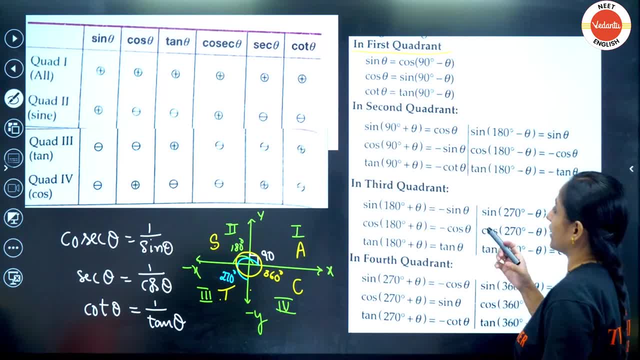 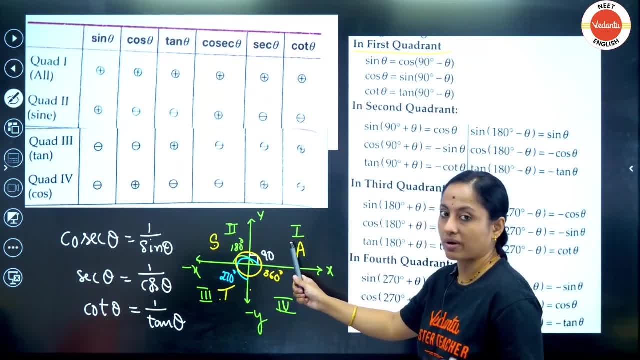 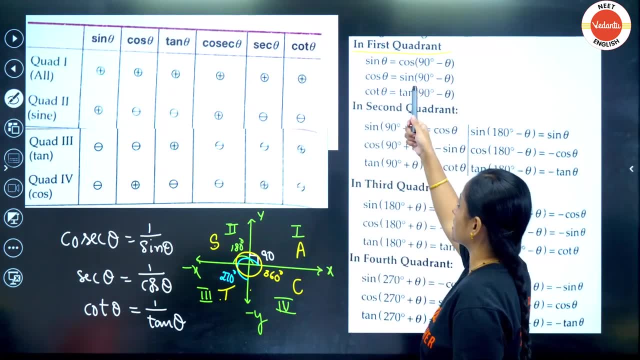 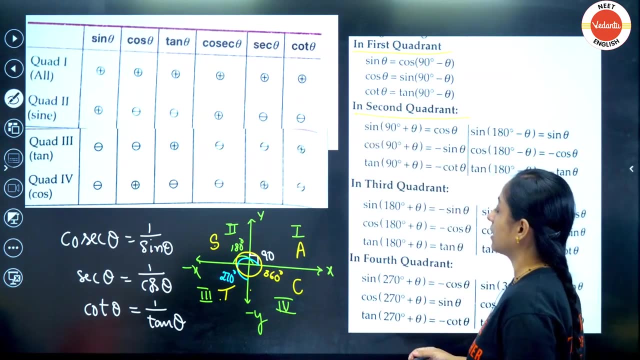 cos 90 minus theta comes into first quadrant. first quadrant: all are positive. cos becomes a sine, positive sine 90 minus theta. first quadrant: all are positive. sine becomes cos, cot becomes tan, tan becomes cot. now coming to second quadrant, just check second quadrant: 90 plus theta. only sine is positive, others are negative. so sine becomes cos 90 plus theta. 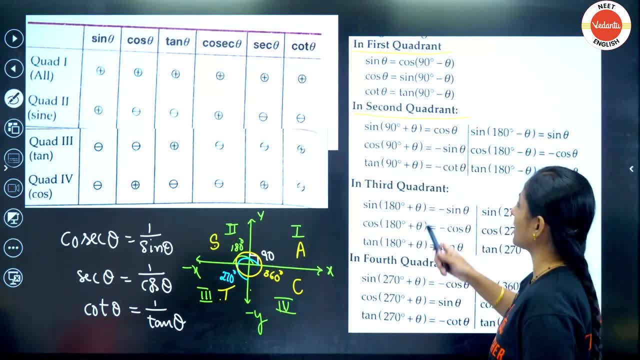 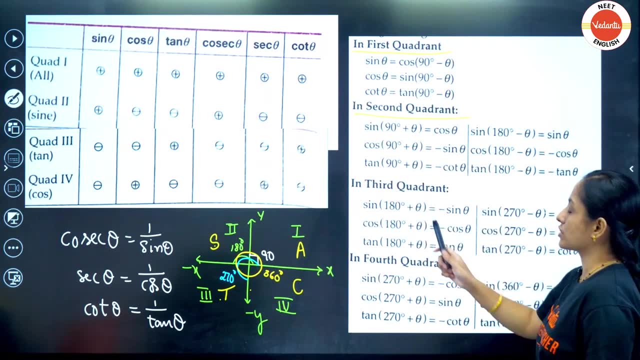 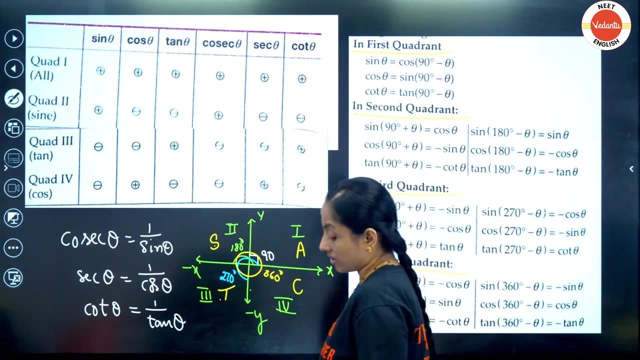 so sine is positive, so it remains positive. so similarly you can see: 180 minus theta also comes into second quadrant. 180 plus theta goes to third quadrant. 270 minus theta goes to third quadrant. so just remember these three, four segments. okay, so either you can learn the formulae by heart. 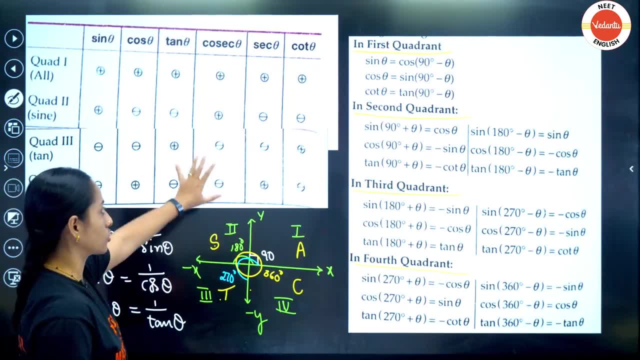 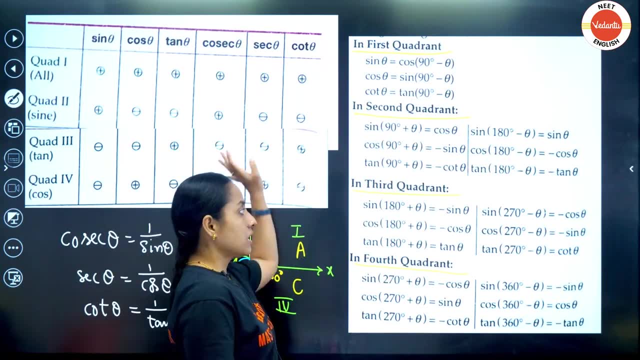 or you can understand from these quadrants also by using this table or simply remembering all silver tea cups. you can learn from these quadrants also by using this table or simply remembering all silver tea cups. that's technique also. you can remember. so this page. yes, memorization is very much important. 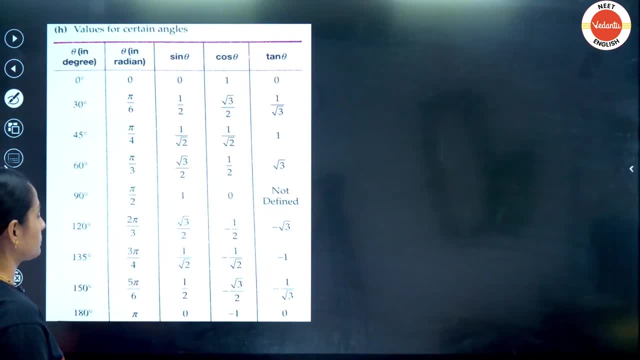 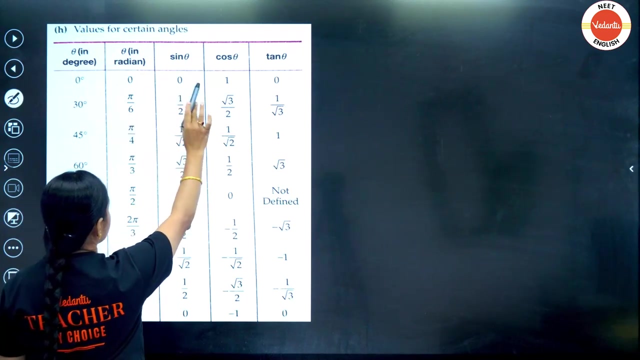 now why this page is required. i'll give you an example also, for example: so here i hope you know this: all table also these values. also you have to make up like a sine zero value. uh, then, in radians and degrees, sine zero, zero, cos zero, one tan zero, zero sine thirty. one, one by two sine thirty, or 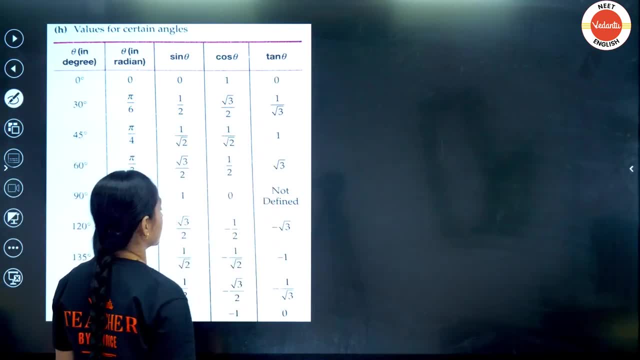 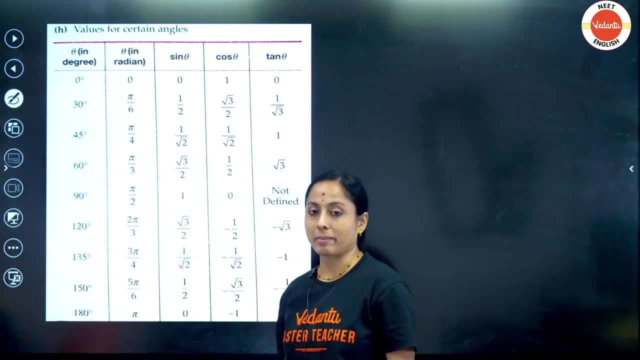 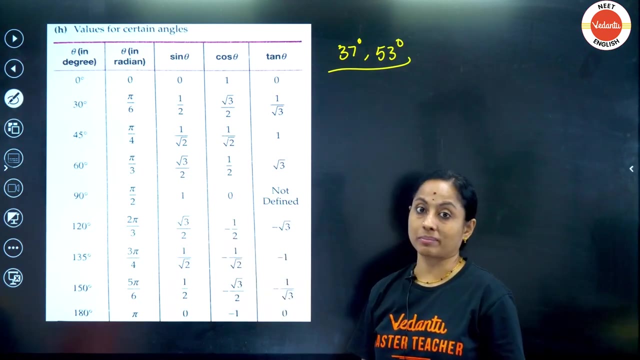 120, 135, 150, all these things you need to memorize, but i'll tell you a technique also. okay, but before that, just remember that there are some angles given as 37 degrees and 53 degrees. sometimes in problems you will find, but 37, 53 is not mentioned here, so i'll give you a shortcut method. what is that? 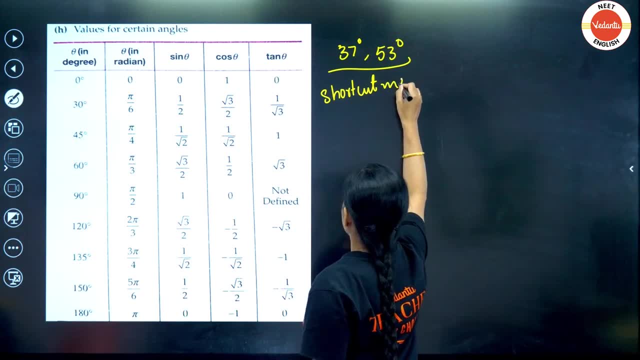 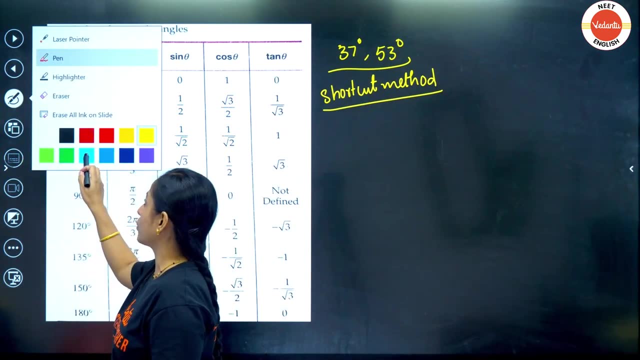 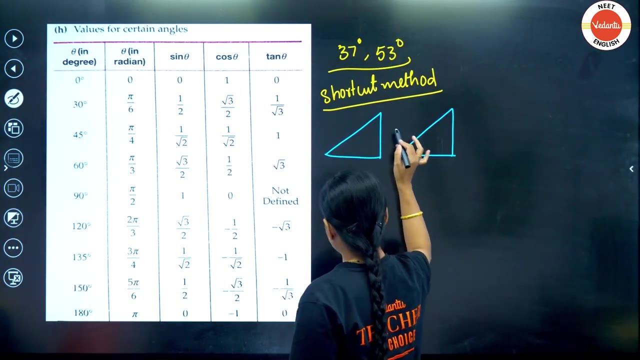 shortcut method. i'll tell you now. see further shortcut method. first of all, draw two right angle triangles. draw two right angle triangles, one for each right angle triangle. write the pythagorean triplet, but first write the angles. whatever you want. one 37 degrees, other contains 53 degrees. 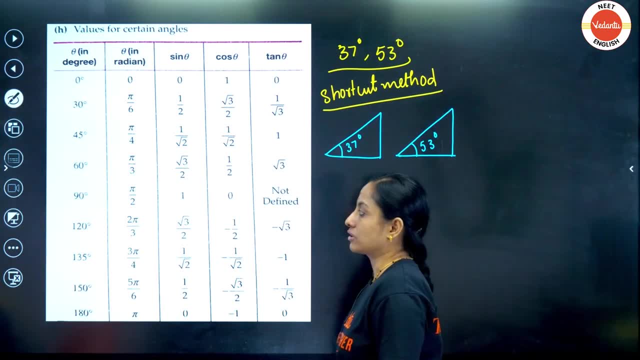 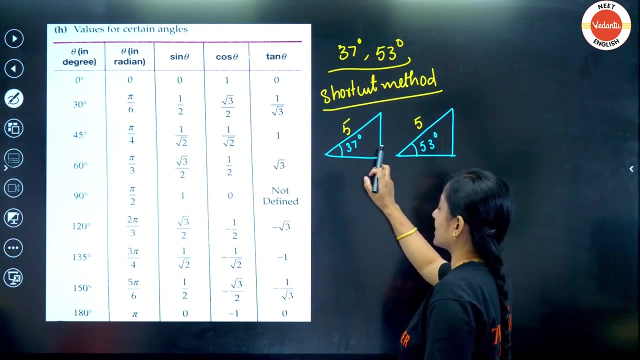 now using pythagorean triplet. do you know what is pythagorean triplet? three, four, five is considered as pythagorean triplet. five is always hypotenuse. write down five here. now, three, four are remaining 37, 53. when you compare, 37 is smaller angle, 53 is bigger angle, smaller number, smaller number. 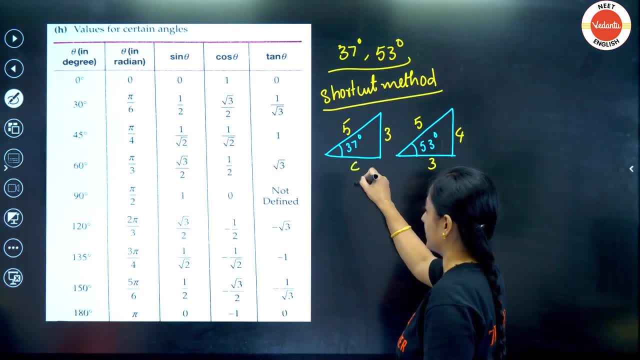 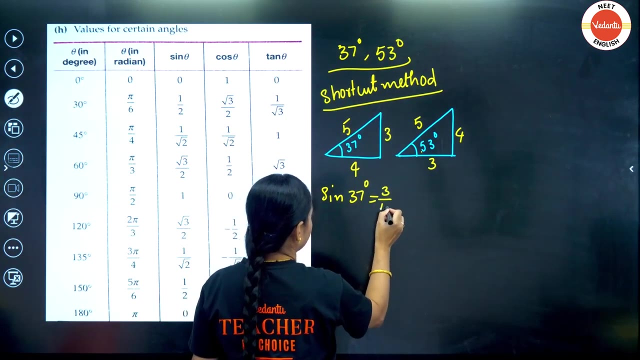 bigger number, bigger number. the other parts come here. have you understood? smaller number, smaller number, Bigger number, bigger number. That's it. From here you can write down sin 37.. How do you write sin 37? Sin 37 is opposite by hypotenuse 3 by 5.. What is cos 37?? 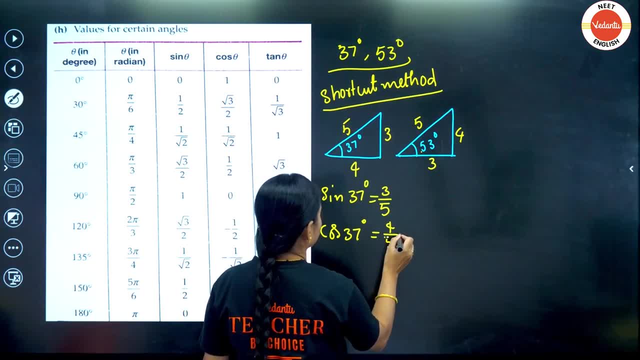 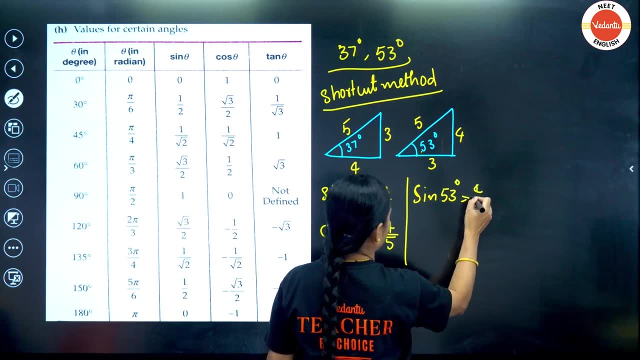 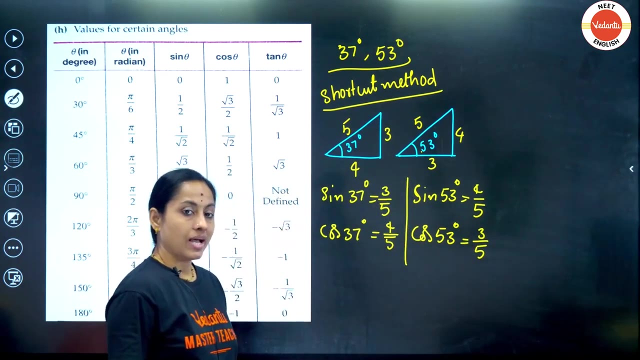 Cos 37 is adjacent by hypotenuse 4 by 5, right. Next, what is sin 53?? Sin 53, opposite by hypotenuse 4 by 5.. What is cos 53?? Cos 53 is 3 by 5.. Have you understood this trick Now, when you know sin? 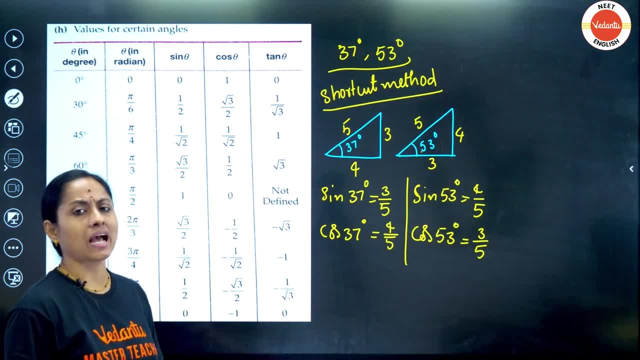 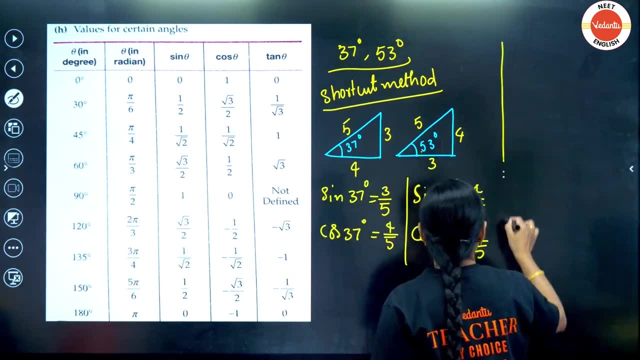 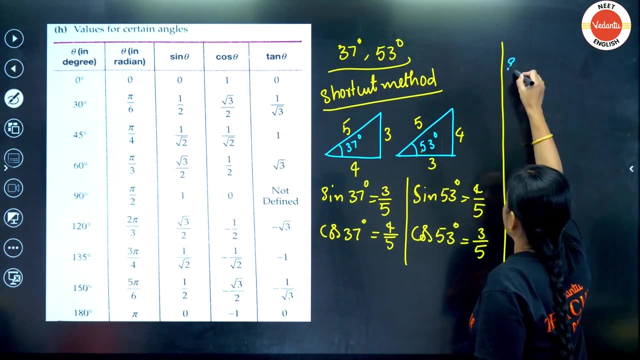 and cos you can obviously write down: cosecant, secant, tan cot, anything you want you can write down. Okay, So this kind of memorization is needed. But I will give you an example also how the problems you will be facing, what kind of problems you will be facing, For example: 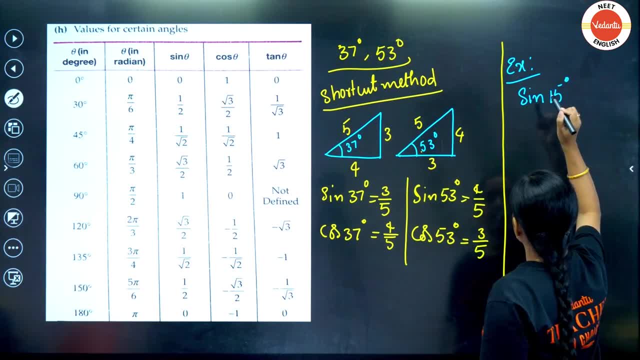 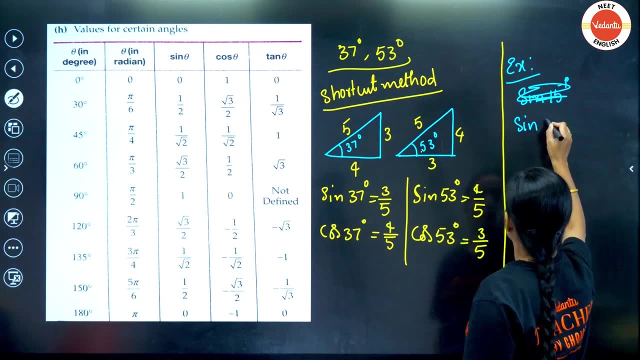 you have sin 15 degrees. Okay, Let us go with the 135 degrees. Let us go with sin 135 degrees, Sin 15. also, I will tell you, don't worry about it, Because sin a plus b. I did not give you the. 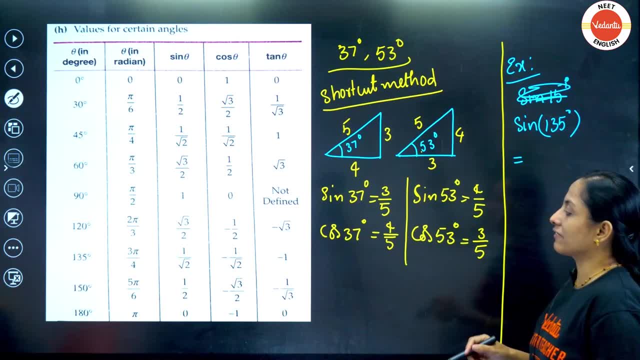 answer. So sin 135, I will find out Now. sin 135, do I need to remember these Without remembering? also, you can solve How So you can write down sin 135 as sin 135.. two possibilities are there. one is 90 plus 45, or you can also write sin 180 minus 45. 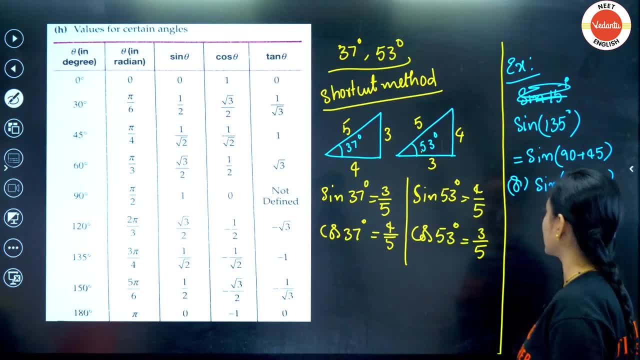 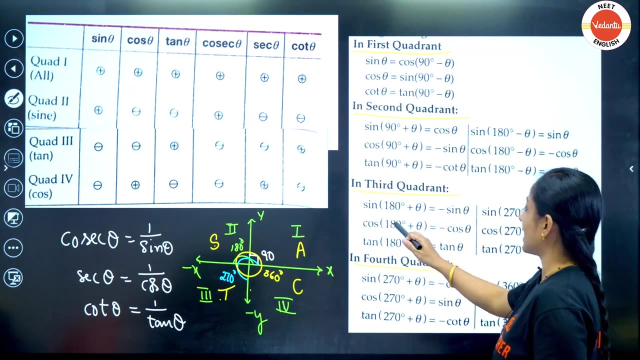 am I correct? 90 plus 45 is 135, 180 minus 45 is also 135. so any formula you want you can choose. you already know what is sin 90 plus theta, formula sin 90 plus. where is it? sin 90 plus theta is cos theta. sin 180 minus theta. sin 180 minus theta is sin theta. so anything you want. 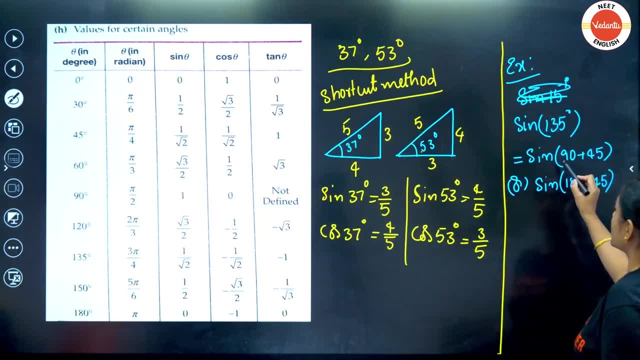 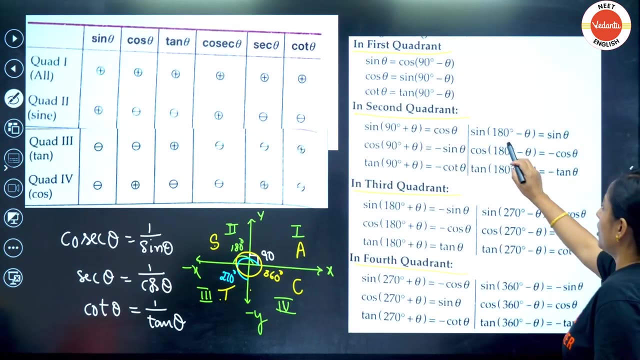 you can write: sin 90 plus theta is cos theta. so sin 90 plus 45, sin 90 plus 45. if I am selecting this, sin 90 plus 45 is cos 45. answer is 1 by root 2. let us take sin 180 minus theta: 180 minus theta: 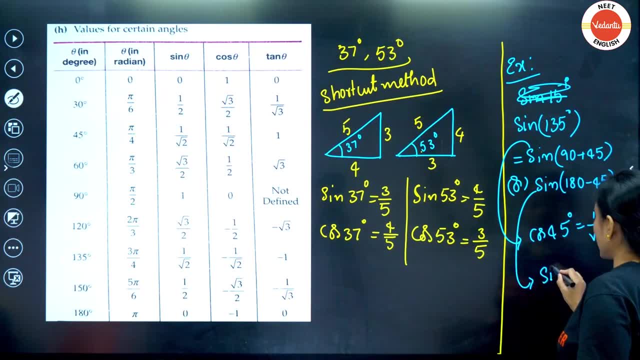 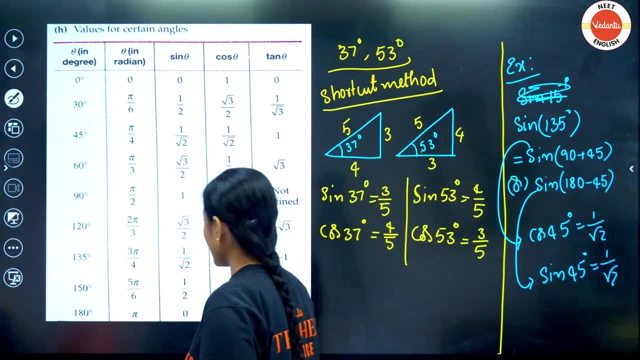 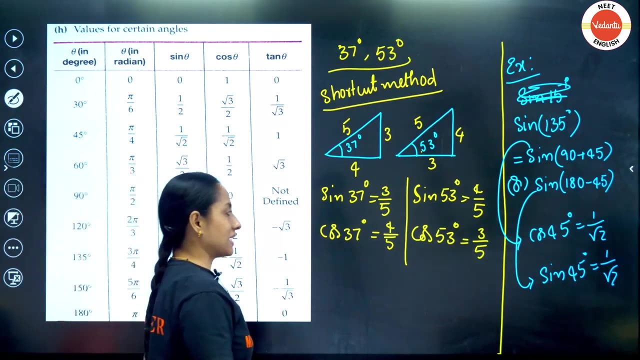 is sin theta. so if I am selecting this sin 45, the answer is 1 by root 2, you will get the same answer, no worries at all. so for the, if you can learn that method, then from here onwards you need to memorize or mug up. you can easily write down.